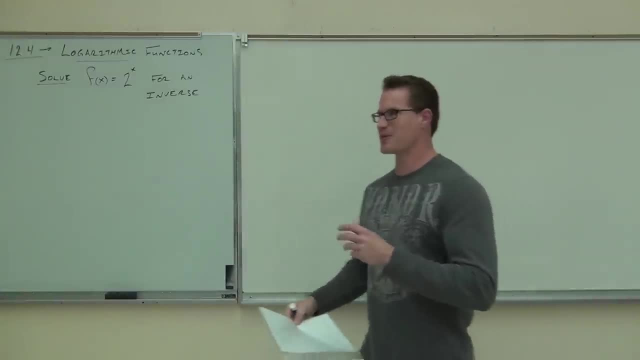 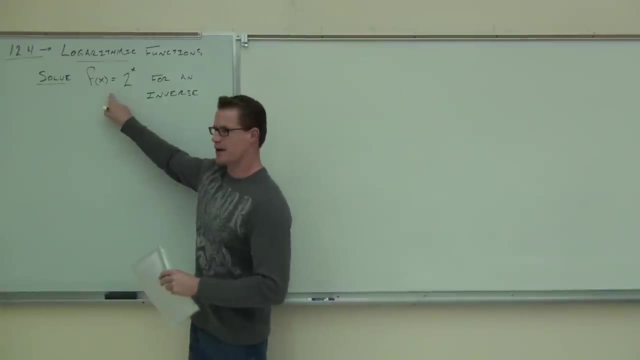 Well, we're going to talk about logarithmic functions. I already had you pronounce that. for me, Logarithmic- it's a weird word, right? In fact, this thing. you're going to find out why this comes about, because we're going to try to solve this. This is called exponential. 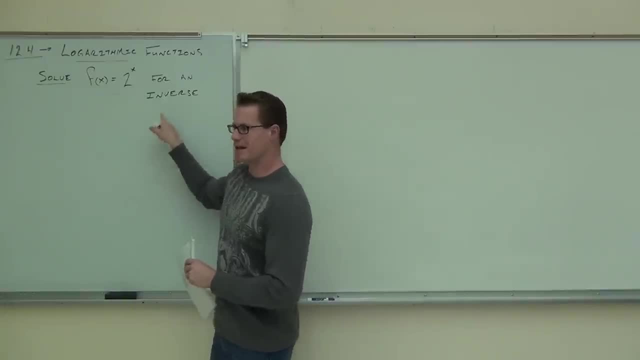 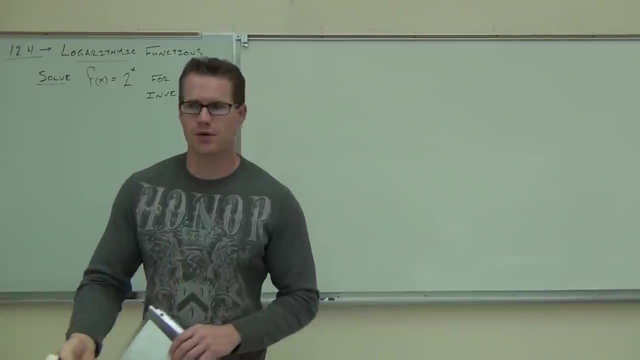 function- You guys did homework on that, right- An exponential function for an inverse. Firstly, tell me what the base is here. Two Good, and the exponent is actually a variable x When we solve for inverses, which hopefully you remember how to do this. the first thing: 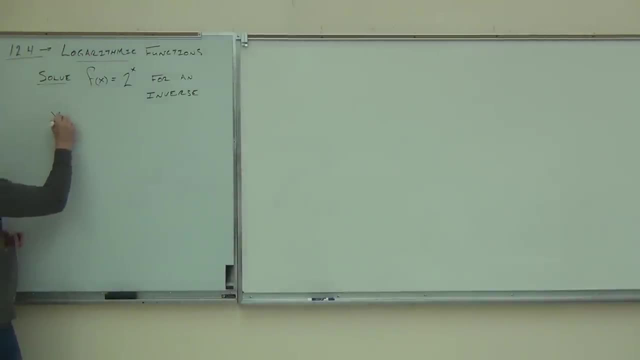 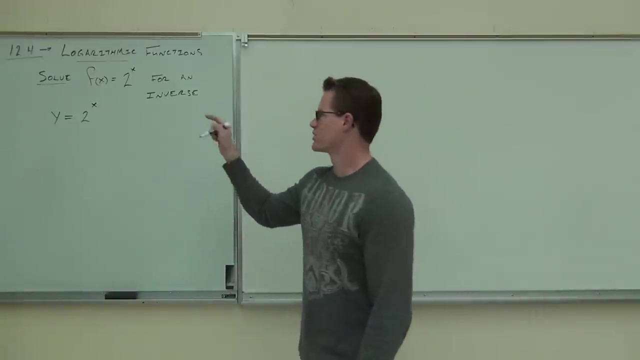 you do with an inverse is you replace your f of x with a y. Do you remember that? Hopefully you do. And the next thing you do, what do you do after you replace your f of x with a y? You replace the x with a y. Yeah, you switch them right. Every x becomes a y every. 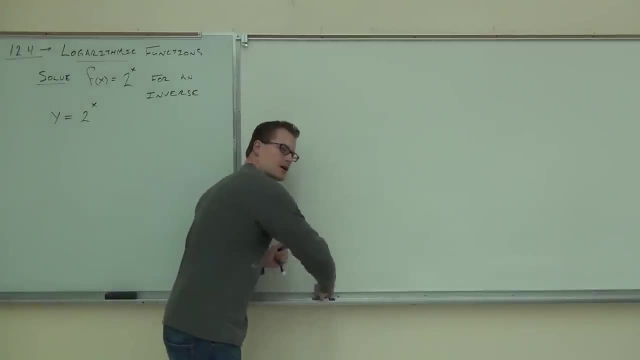 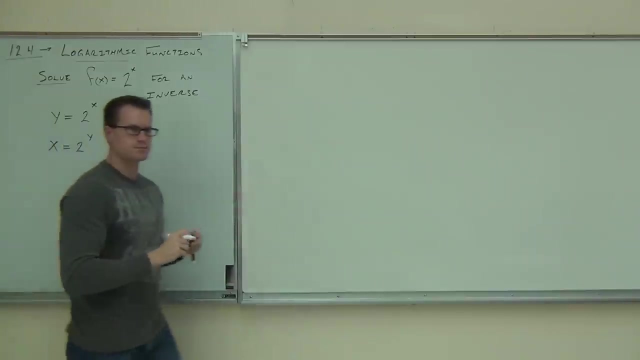 y becomes an x. So check this out. If I'm trying to solve this for an inverse, my very next step is to go: okay, instead of y equals 2 to the x, it should be x equals 2 to the y. Do you follow? Hopefully, yeah, you follow. 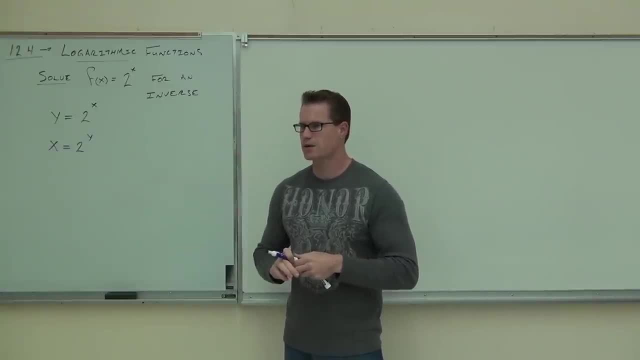 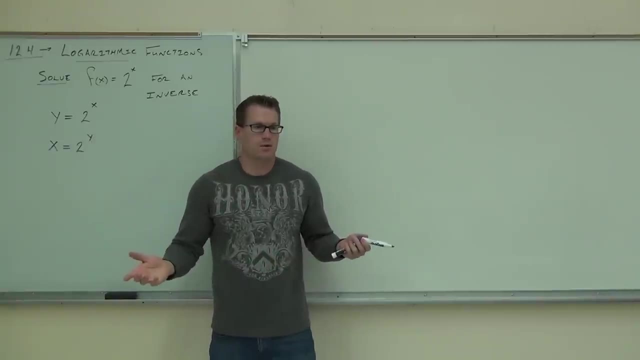 And the next thing you do is you try to solve that for y, correct. How in the world do we solve that for y? Well, you don't know. That's not going to get y by itself. That would get rid of the y, but it would have a y inside of a root right. We don't want that. We don't. 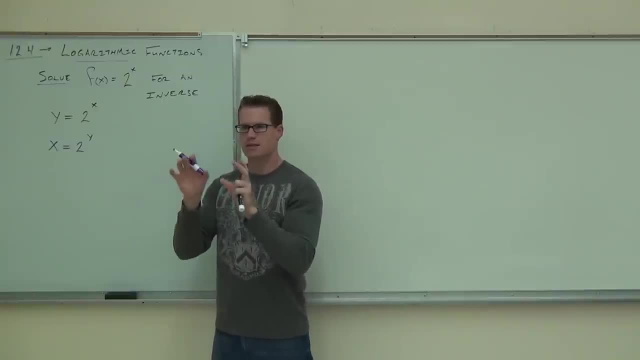 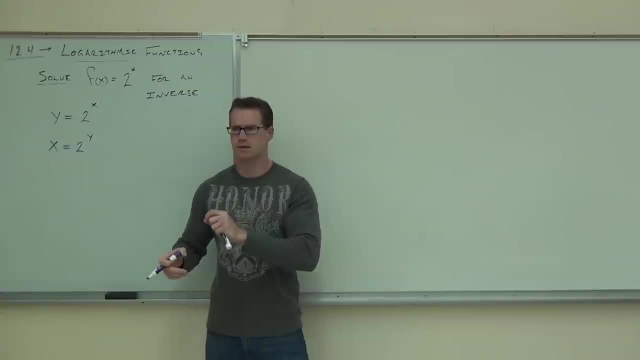 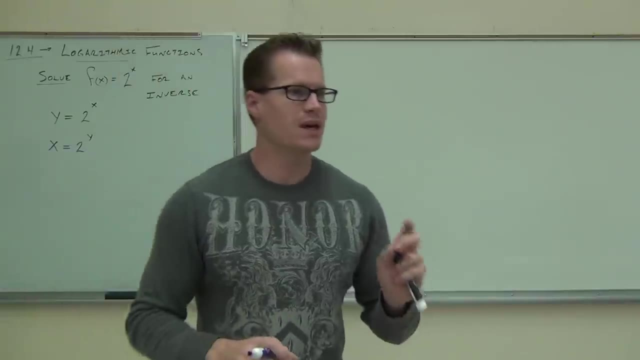 You'd have 2 to the y minus 1 up there. Any other ideas? You guys are having the right thought process. That's great, But there's no way, conventionally, that we can get rid of this scenario. There's nothing. you know how to do that. You don't know how to do that. 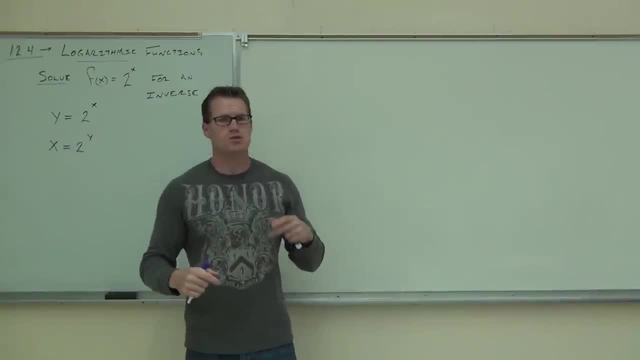 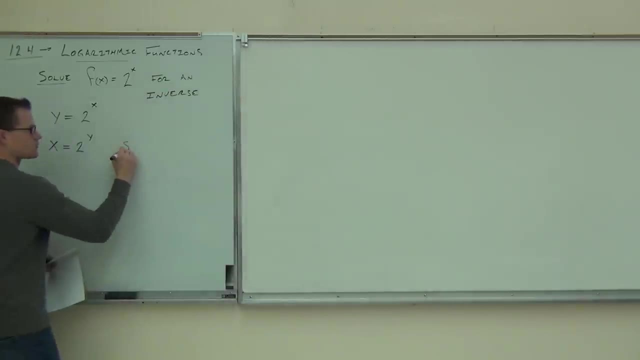 yet That's why, when we get to this point, you'd be stuck, unless we create something called a logarithm. A logarithm is the way you deal with this thing right here. See, right now, if we solve for y, you're going to go: ah what? You're not going to get it because there's nothing. you 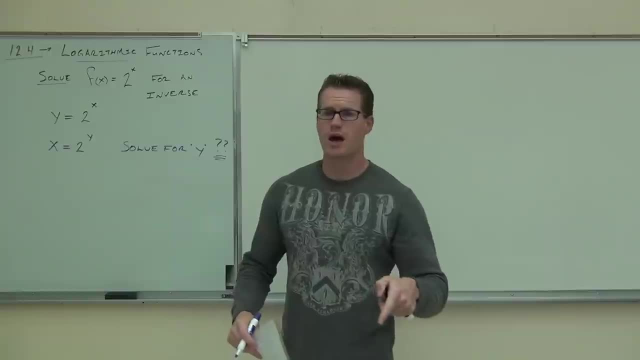 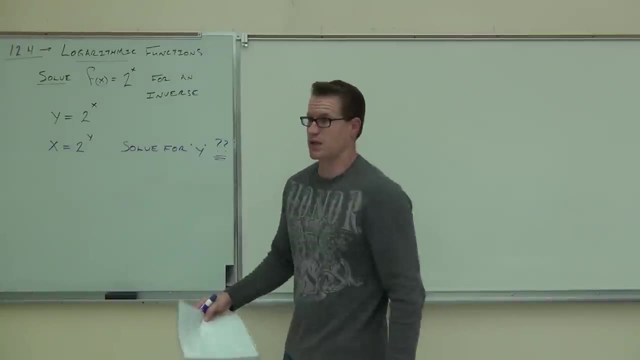 know how to do to solve for y right now. That's why I'm going to introduce to you something that's going to make it so that you can solve for y. Would you like to learn that? Otherwise you can't do this, Otherwise you're like: ah done, stuck. Well, maybe some of you would. 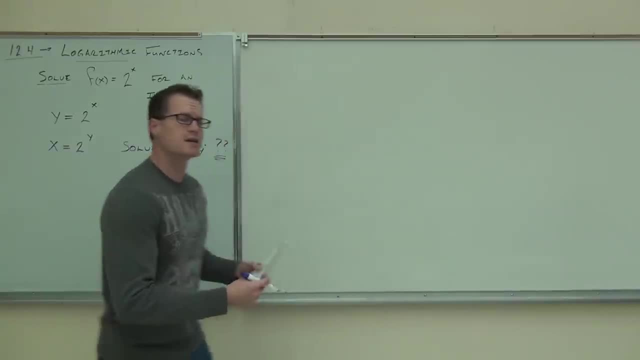 rather be stuck right, Say no solution. But there is a solution and it's given to you by something called logarithmic notation. Here's the idea I'm going to give it to you in general. If x equals b to the y, very much like this, right Instead of 2, though I have a general unpacker. If 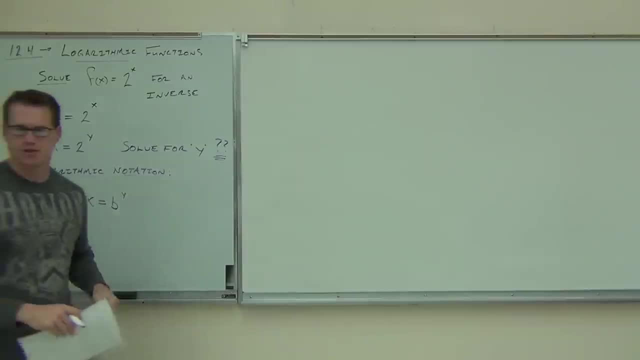 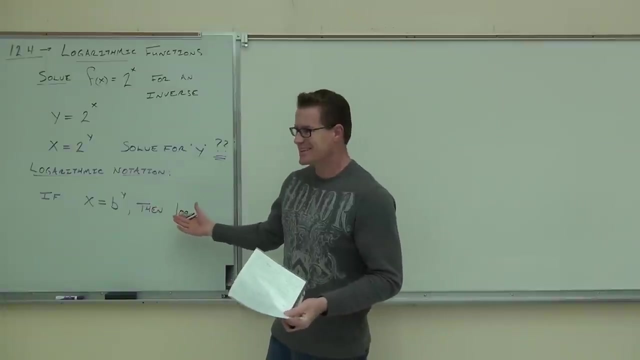 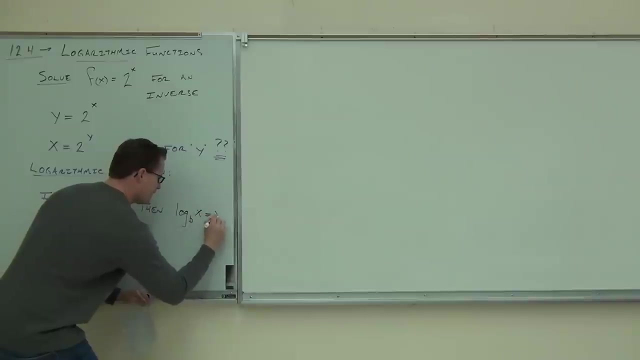 x equals b to the y. here's where the logarithm comes in. Here's where the logarithm comes. It's a perfect season for log rhythms, right since you build fires. what do you use for fires? Logs, obviously. Here's how this is set. this says log base B. what's B? 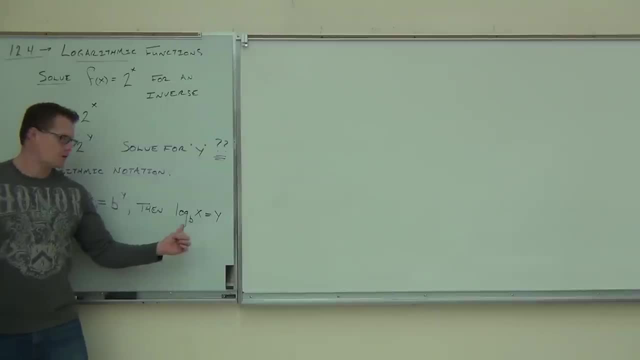 A base exponent. what is it? It's your base. I want you to look over here. what is your base over here, please B. What is your exponent over here? Y? And then B to the Y would equal X, right. 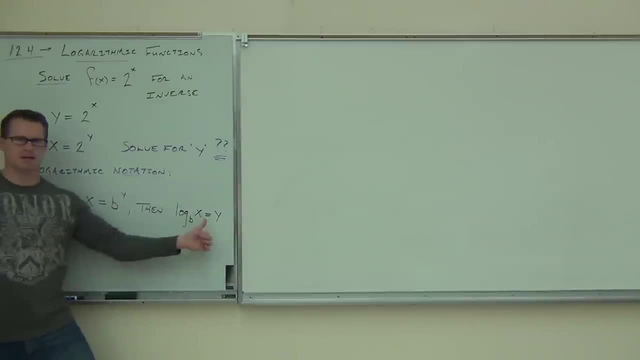 Yeah, Your base over here is still B. these are the same exact letters. Y. that's where your exponent goes. it's kind of strange, right, But look what it does. Do you see how this solves an exponential for Y? 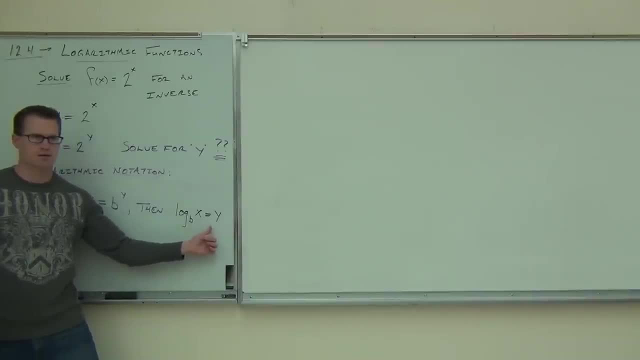 Do you see how Y is all by itself right here. I hope you're awake. today some of you guys are coming in late, which is ridiculous, But right here. do you see how your exponent is now all by itself? Yeah, You got Y equals to this log rhythm. 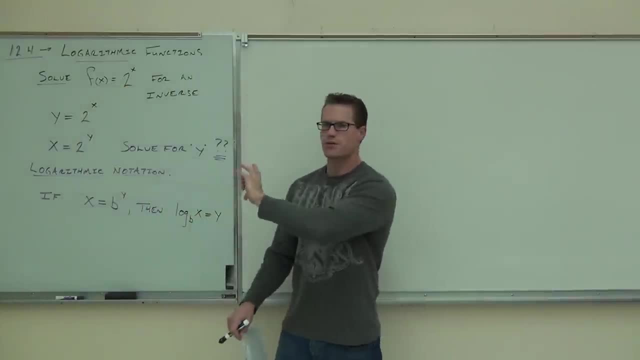 That's actually solved your exponential for you. that's solved for the inverse of your exponential. So it's taking your exponential and said, how am I supposed to solve for Y? Hey, it did it. It did it for you. This notation is something you need to get really, really familiar with. 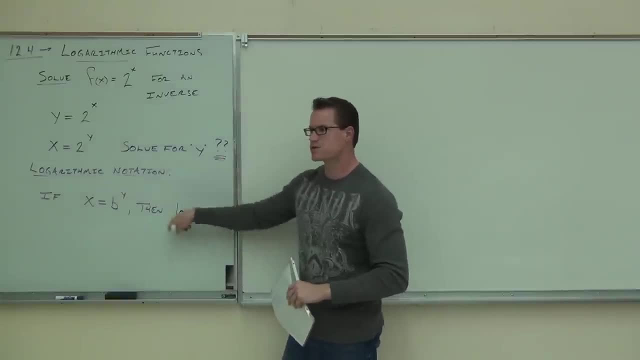 Would you still have to rewrite that Y as the F minus 4 and X? Yeah, if you were trying to find the inverse, absolutely, We're not going to be working with that just yet. we won't in a few minutes, But for right now, no. 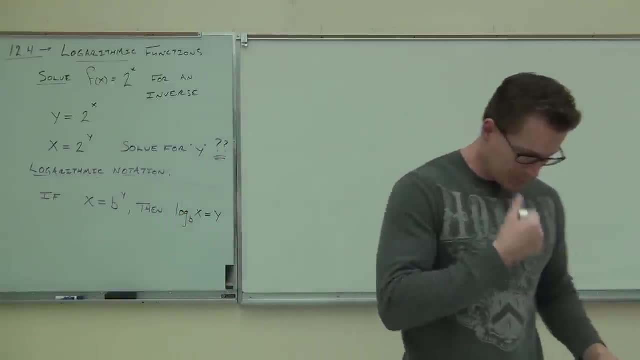 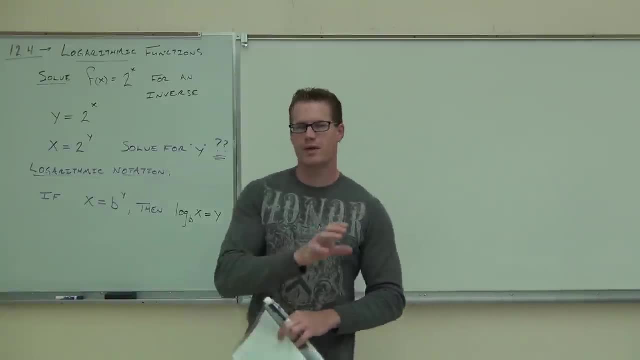 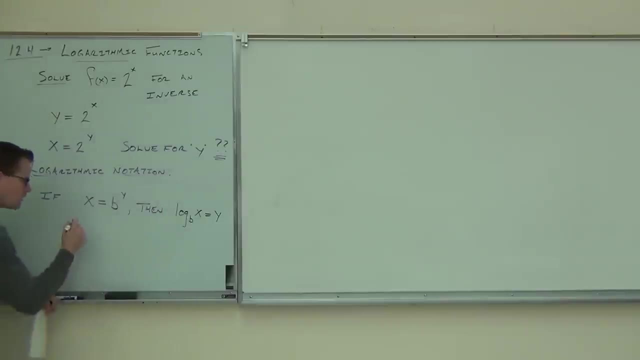 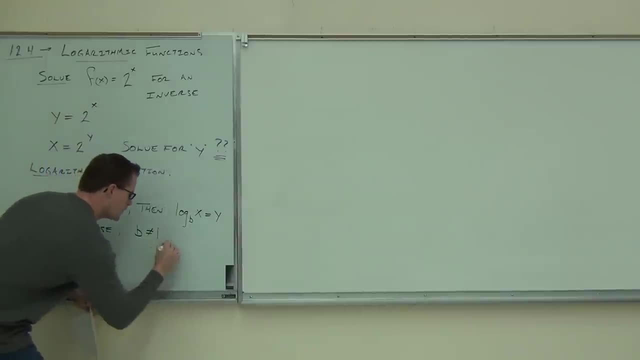 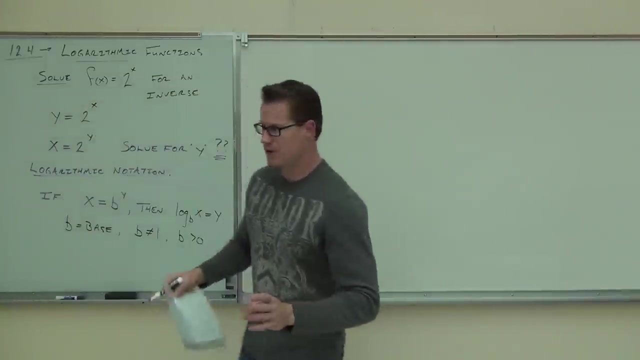 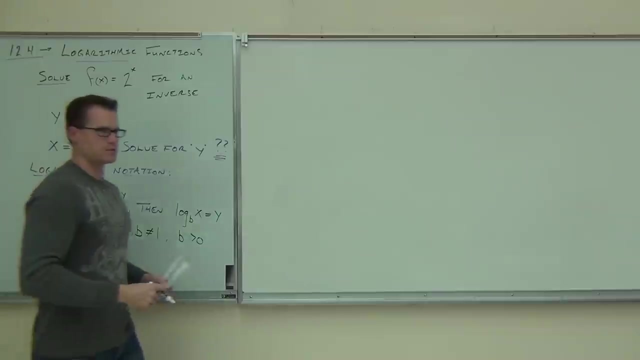 1. And it was online That one will be very fun. B is always going to be greater than 0. So you're never going to have a negative base. We can't have that logarithms. and also, X is going to be greater than zero. you're not going to. 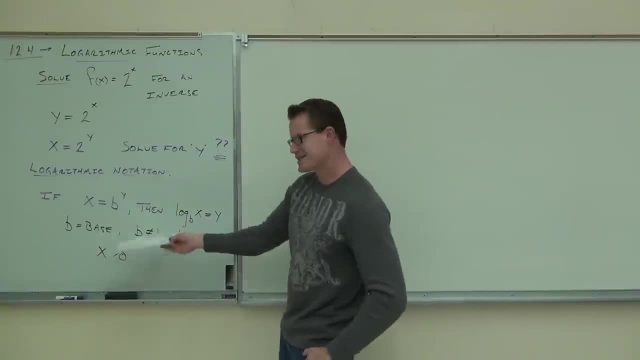 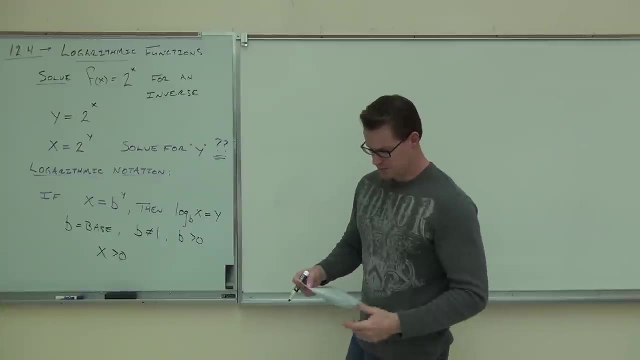 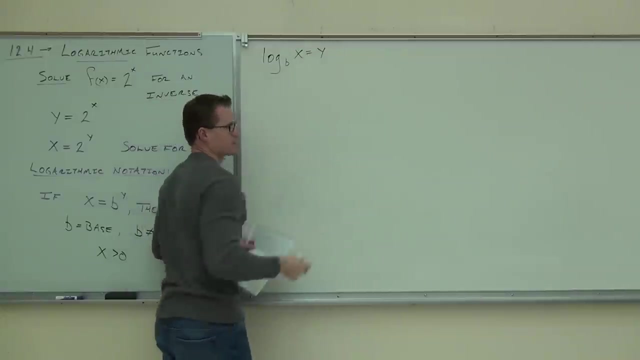 have a negative X. so a couple conditions here: B is still your base, never equal to one. B is going to be greater than zero and X is always going to be greater than zero. so here's what this says. if we're talking about log base, B of X equals Y. here's: 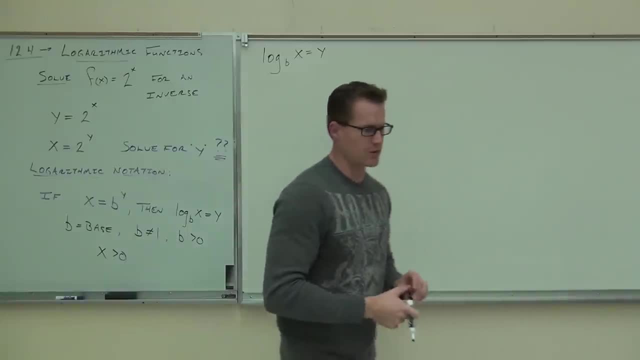 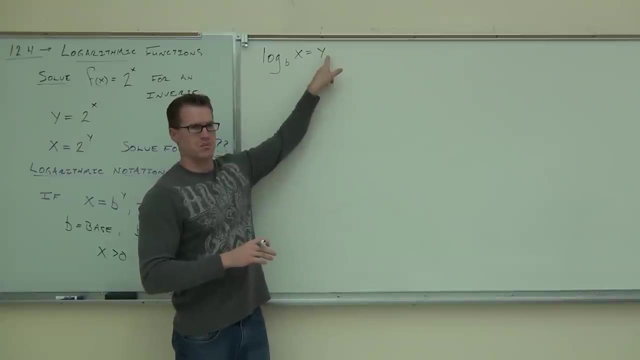 how you can think about this in English. here's what it says in English: Y is the power. what's Y? is it a power? yeah, it's a power, not a base. what's your base here? yeah, it says Y is the power to which B is raised in order to get X. it's a weird. 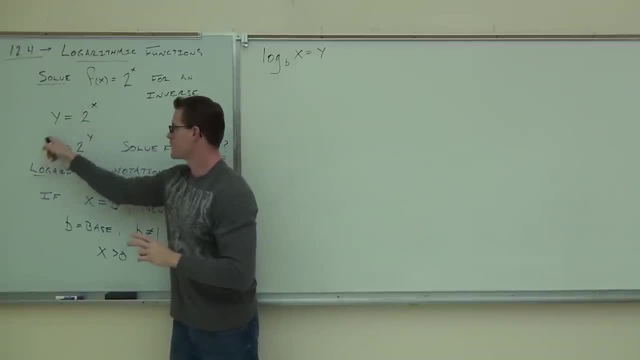 way of looking at this situation right here. it's a weird way of looking at this thing. Y is the power, it's an exponent, to which B your base is raised in order to get X. so, all right, I'm going to write that out for you. here's how you think of this. 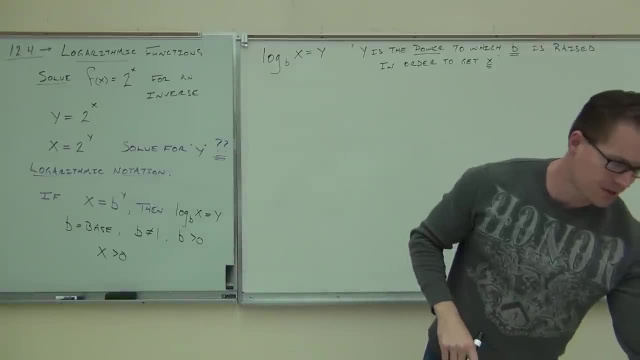 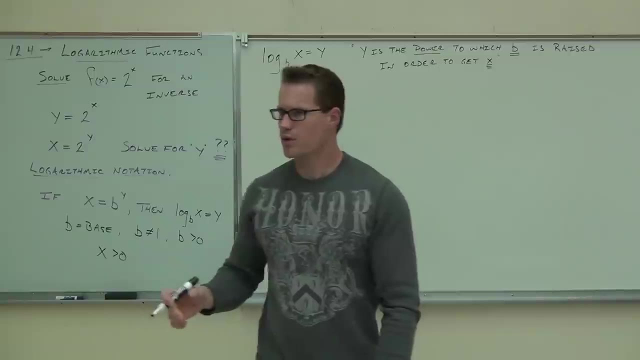 Y is the power to which B is raised in order to get X. Now would you like to see a couple real life examples of this, Just so you can kind of get the picture of how this stuff works. What we're going to try to do is translate from what's called log-rhythmic notation. 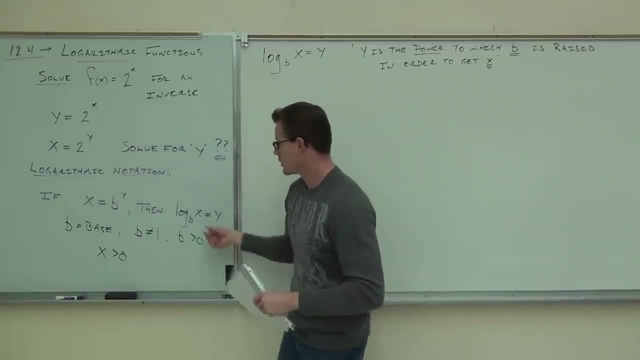 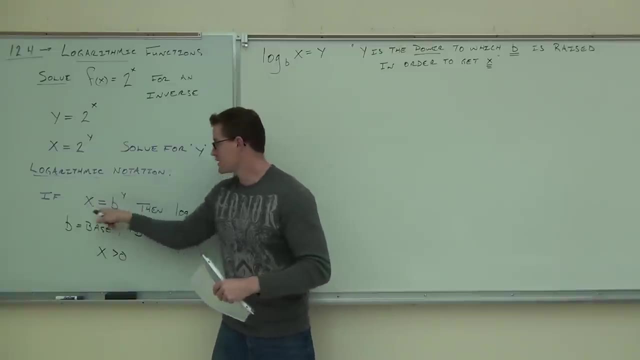 If you say log-rhythmic, you've got to have a log. So this right here, that's log-rhythmic notation. This is exponential notation, So we need to have that in our heads. You need to know that. exponential means this: no logs. Log-rhythmic means well, logs. 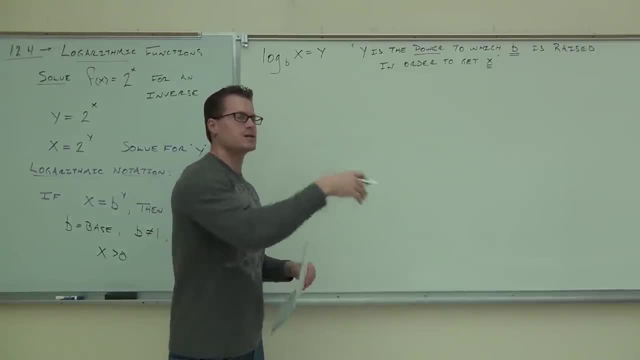 We're going to translate from log-rhythmic to log-rhythmic. So we're going to translate from log-rhythmic to log-rhythmic. We're going to translate from log-rhythmic to log-rhythmic. So we're going to translate from log-rhythmic to log-rhythmic notation into exponential notation. 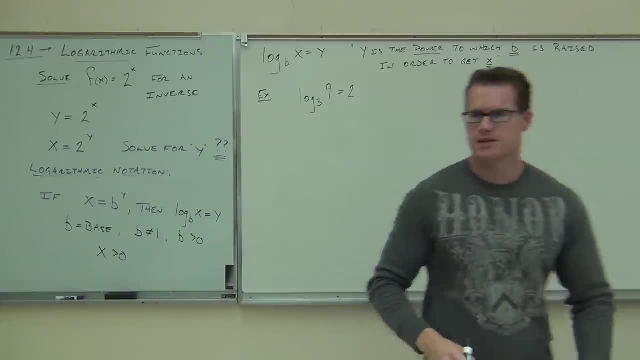 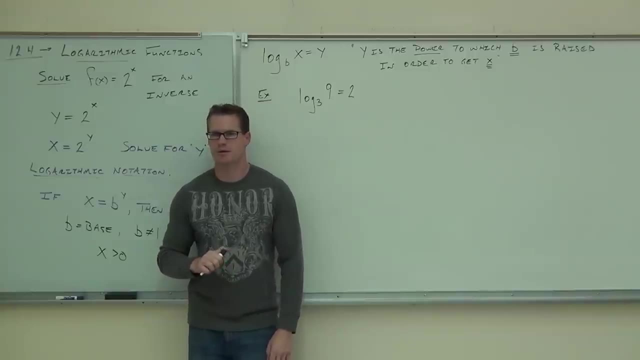 And I want your full on participation up here. Let's make sure we all are getting this. This is going to be a real big second zone for us to make sure we get to the next part. So, everybody in here, what is your base in this problem here? 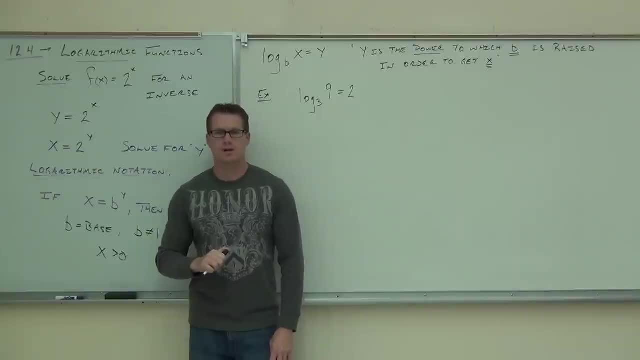 Good. What is your exponent? Notice how it's very easy to say 9.. It looks like: oh, the 9 is right above No 9 is not your exponent. Your exponent right here is your y or your 2, in this case. 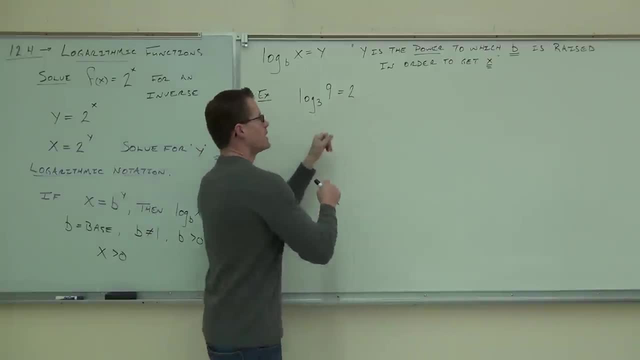 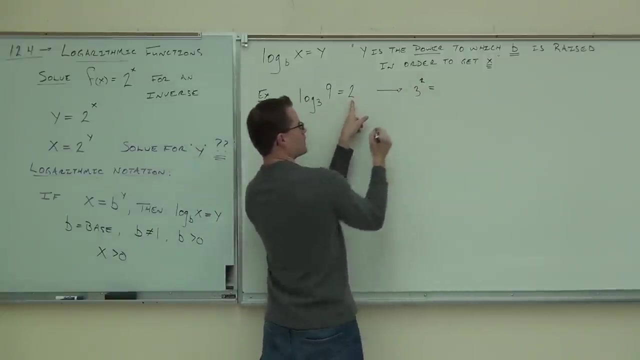 Your base is 3, your exponent is 2.. And here's what this says. It says 2 is the power to which 3 is raised in order to get what number. That's what it says. So if you were to translate this, your base is 3, your exponent is 2.. 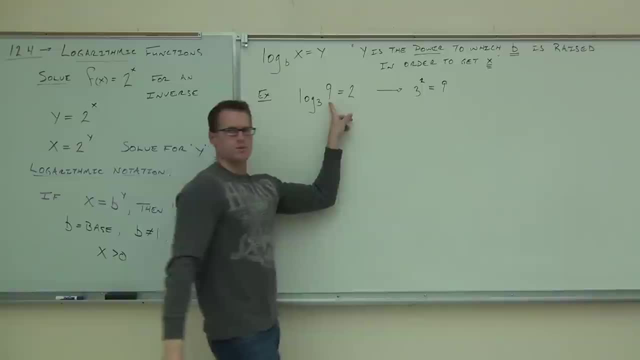 That's supposed to equal this number, does it? Is 3 to the second equal to 9?? Good, That's your base, That's your power. It says this number is what you must raise this base to in order to get this number. 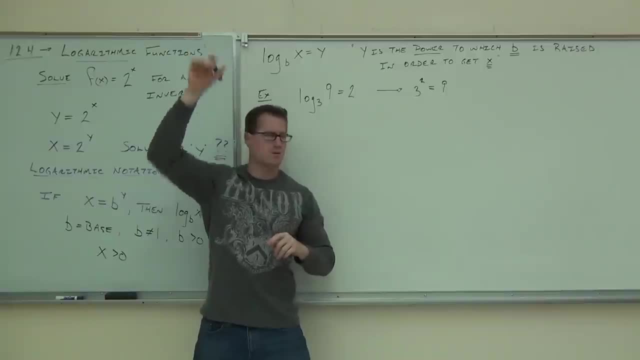 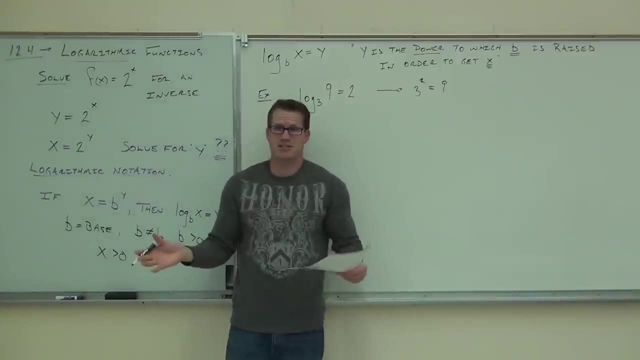 That right, there is your exponent. How many people feel okay with this so far? We're going to try several more, just so you can get the hang of it. This is brand new for you, right? You've never seen this before. This is something you're going to have to know how to do. 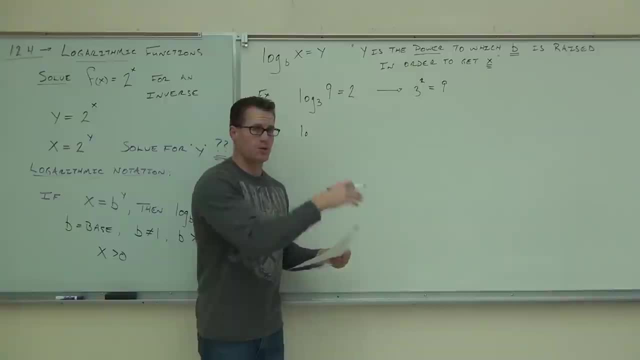 It's a construction. It's something somebody made up in order to represent this easier. What is your base here? 7. Good. What's your exponent here? 2. Good, And so you're supposed to write what first, 7.. 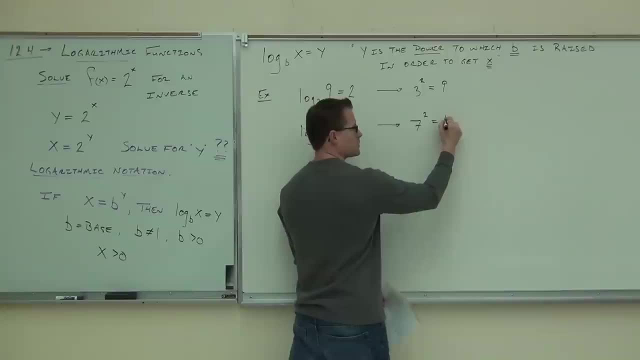 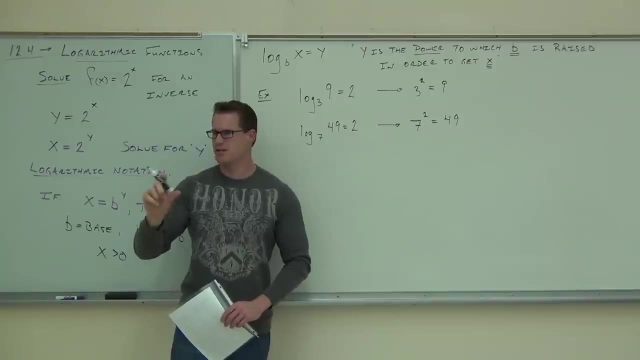 7 to the what Equals how much: 49.. Perfect, You're starting to get it more and more where the base is coming from, what the exponent is and what those two things have to combine to equal. so your base to your power has to. 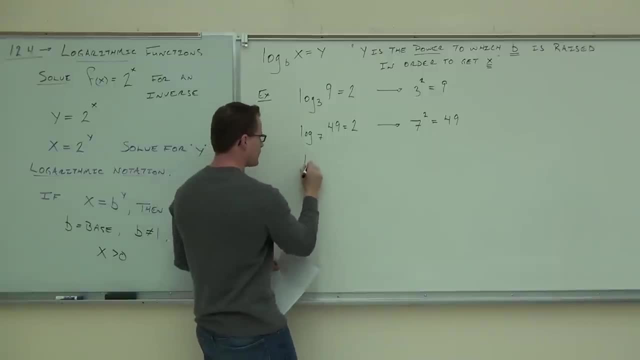 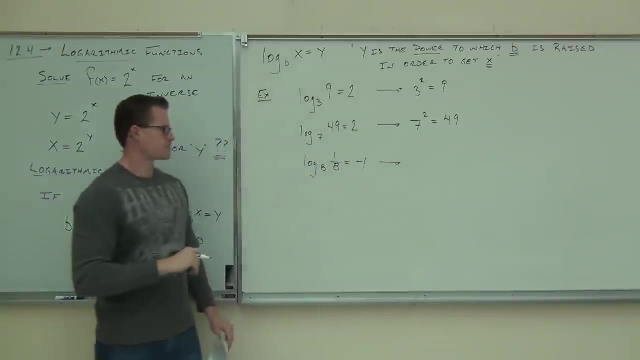 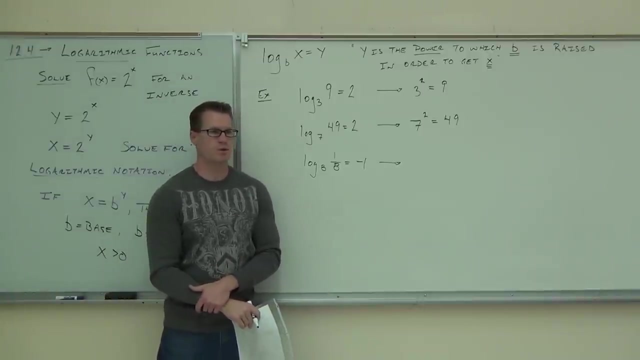 equal that number right there. All right, Ladies and gentlemen, let's do this one together. What is your base here, folks? I want everyone to participate and let's look up at the board real quick. What's your base? 8.. 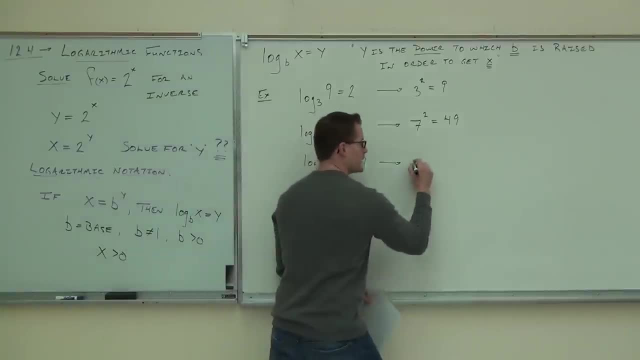 Good, What's your exponent? 1. So you're supposed to write 8 to the negative 1. That's how it always works. Your base is raised to your exponent and that equals how much? 1.. Hey, is that a true statement? 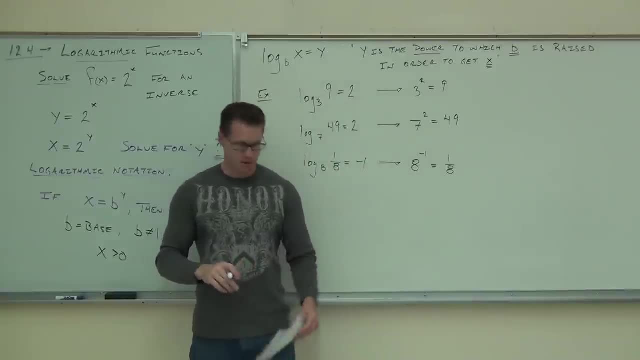 Is 8 to the negative, 1 equal to 1-eighth? Yes, Absolutely, That's what it means. You know, in fact, some of these. you might be able to tell me what's your power. Can anybody think of what that power has to be? 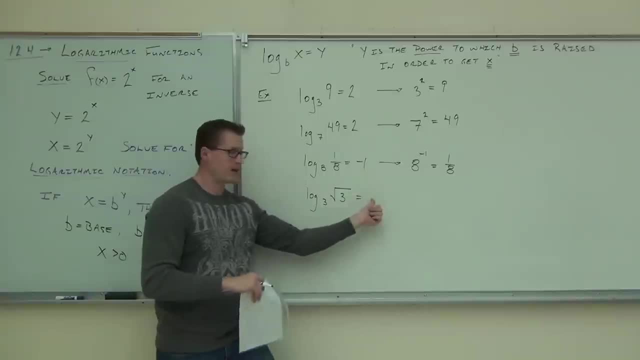 If you're really starting to get logarithms, you should understand kind of what. that is right. What's your base here? 2. Your base is 3. Not 3.. What would you have to raise 3 to in order to get the square root of 3?? 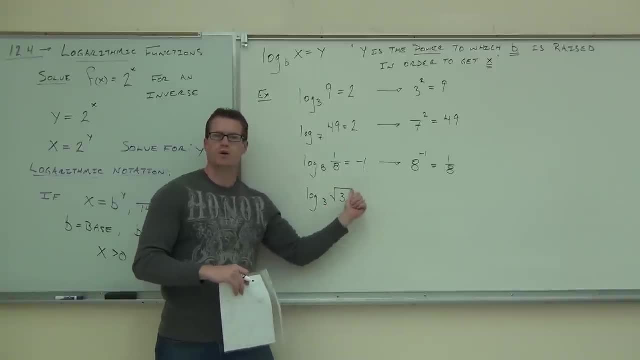 1. 1. How about 1-half? Yeah, Your base is 3.. Your power is 1-half And that's supposed to equal the square root of 3.. Is that a true statement? It's 3 to the 1-half, equal to the square root of 3.. 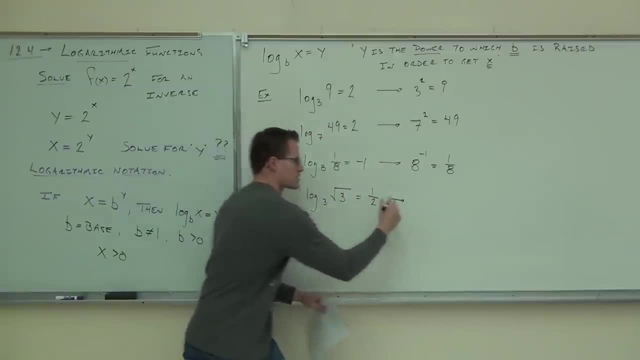 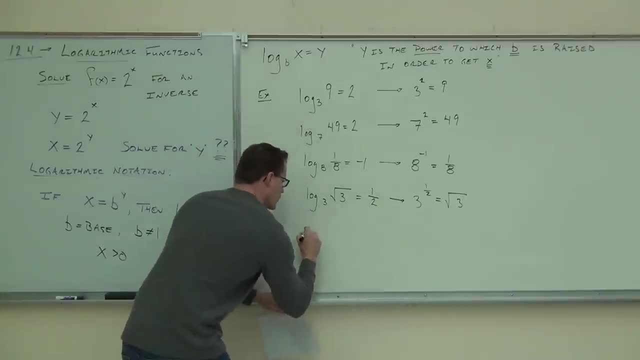 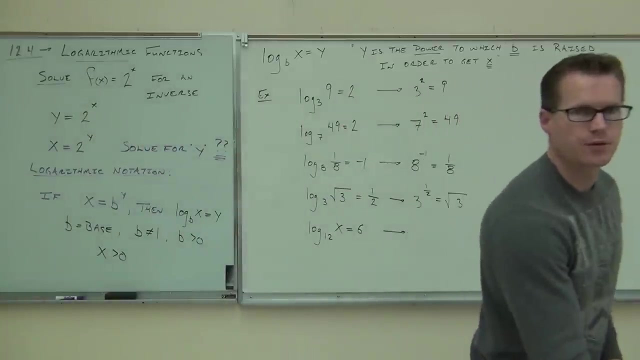 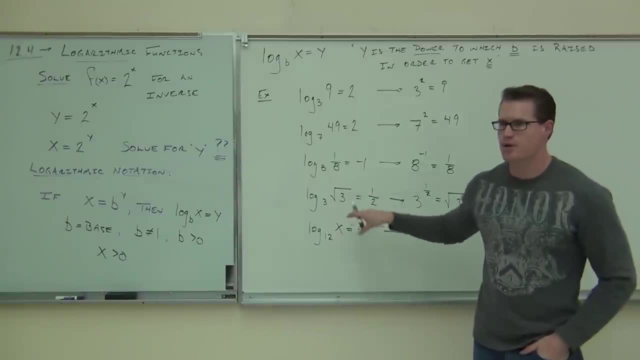 1.. 1. Can you still translate that one? Can you still translate that folks? Sure, OK, let's do that. It doesn't matter what we have up here. we could have all letters and still be able to translate that appropriately, because we know how to write this 1.. 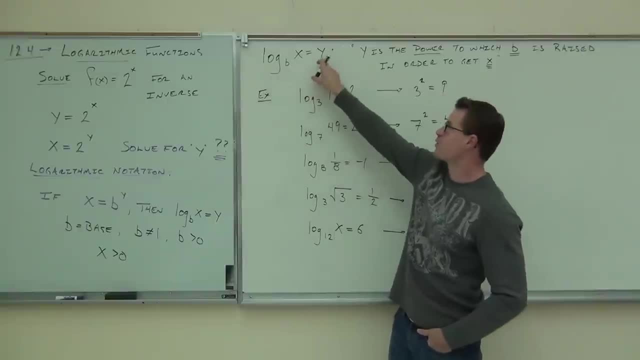 1., 1., 1.. and that's an exponential. We know that's your base, That's your power, That's what the base to the power equals: 2. What's your base here, ladies and gentlemen? 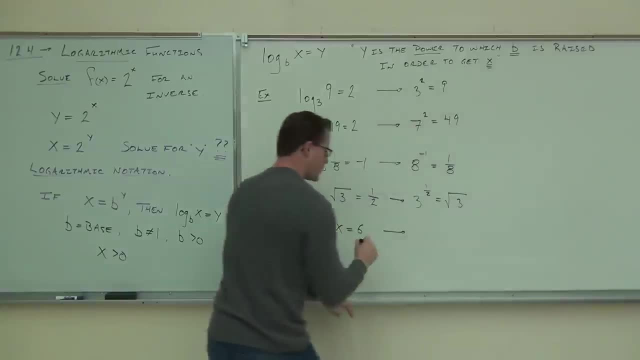 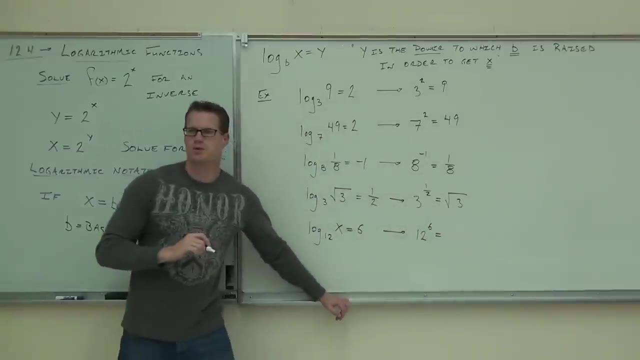 1. 1.. So we write what? what is this over here? 12 to the 6th, 12 to the 6th- Very good. How much is 12 to the 6th equal to? I don't know. Well, no, I'm sorry. How much is what's? 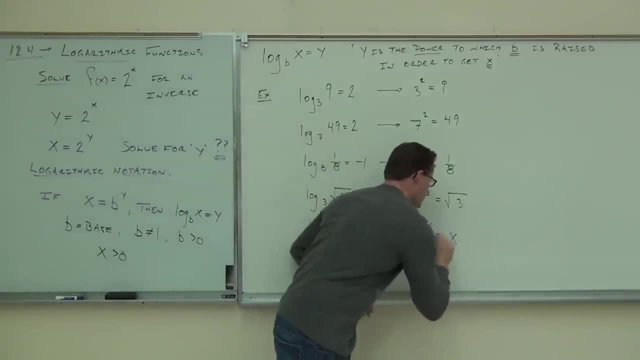 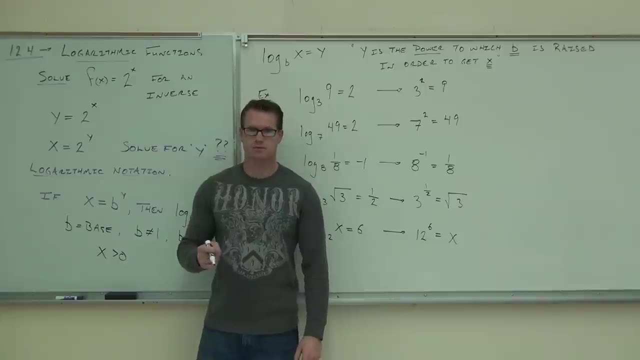 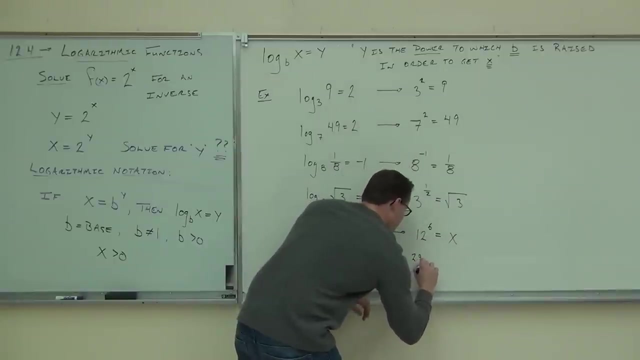 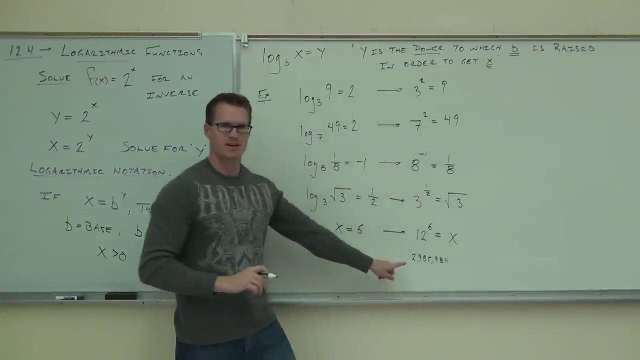 supposed to go right there? X. Hey, could you do 12 to the 6th power? What is it? A lot Big number, I don't know. Almost 300,000.. Tell me exactly what it is. It's almost 2,985,984.. 2 million 985,984.. Oh, that's interesting, isn't it? That number, That number, That number, Really? That's what it says. Yeah, Crazy, That's big right. Here's why people invented logarithms. for one reason, Well, one of the reasons they invented them: Firstly, to find the inverse of an exponential. Secondly, because if you have a base over here and you 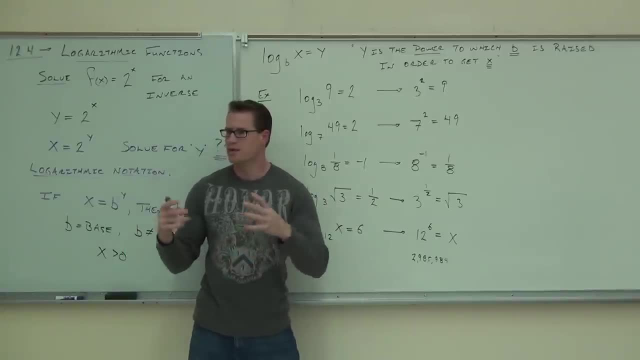 have another logarithm base. we're going to learn in just a section that we can combine logarithms, expand logarithms and use logarithms to do basic math operations. So what people did a long time ago when they were doing calculations that were like astronomical, like big numbers, they changed them into logarithms, used this number, then, at the very end, changed them back into the numbers that they represented. Because is it easier to work with this number or this number? That number 6 is easier to work with than 2,985,984. 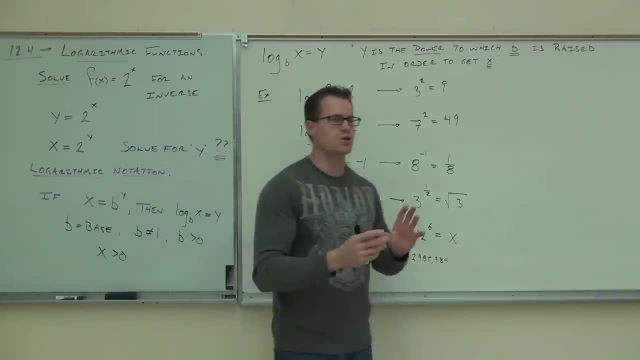 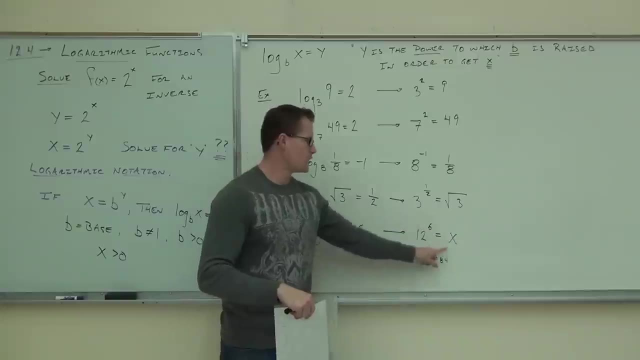 Okay, Way easier. So that's what people did. They used those logarithms to do math. It's kind of cool. Okay, try one on your own here real quick. You don't have to go this far, by the way. I just want you at this point, to be able to. 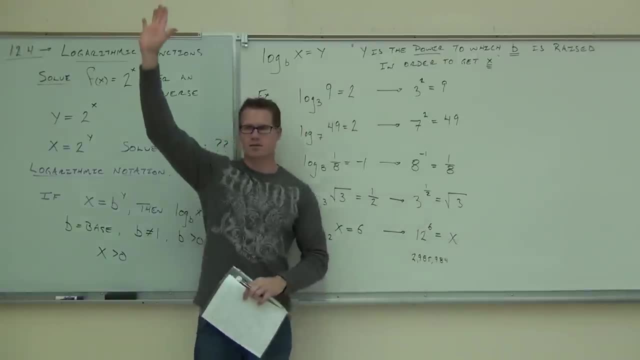 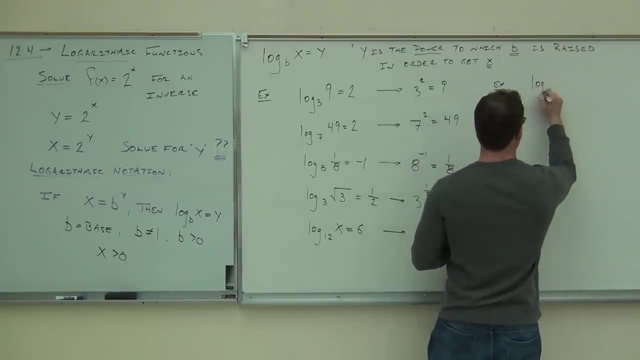 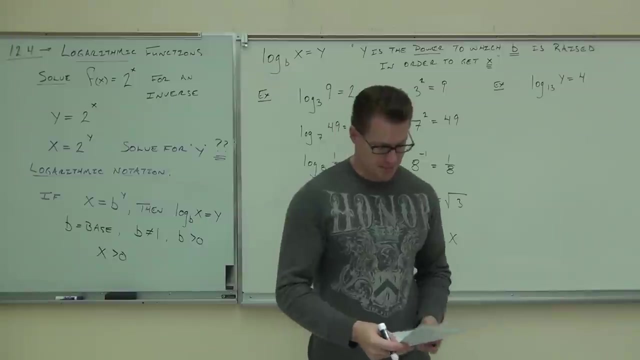 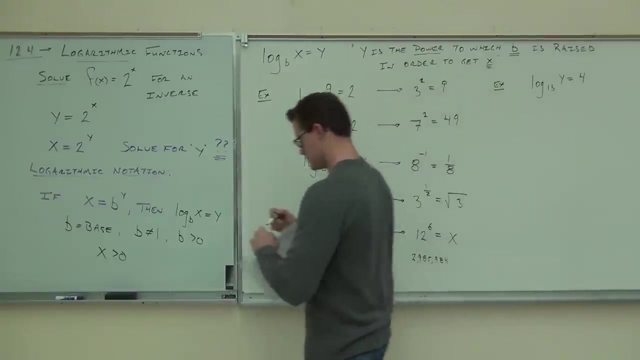 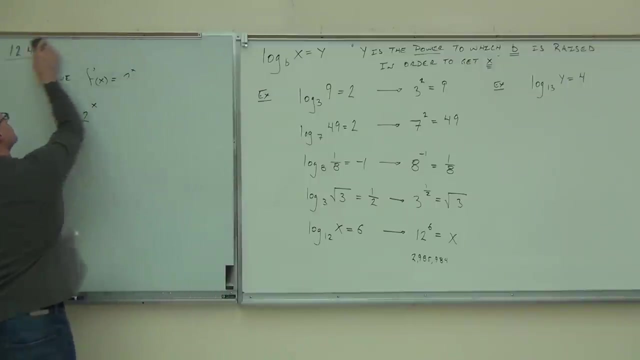 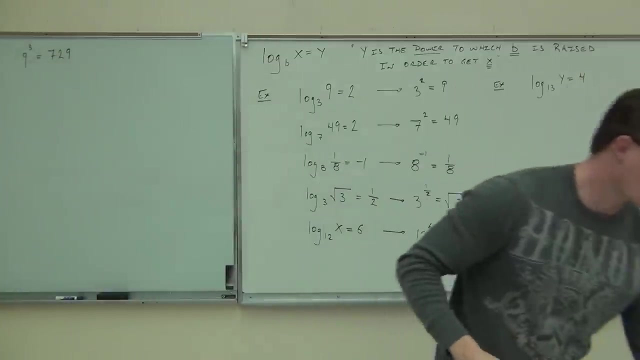 get this far. Raise your head if you feel okay with these several examples. Okay, try one on your own. I want you to translate that into an exponential. Okay, what is your base, folks? What's your base? 13.. 13 is your base. 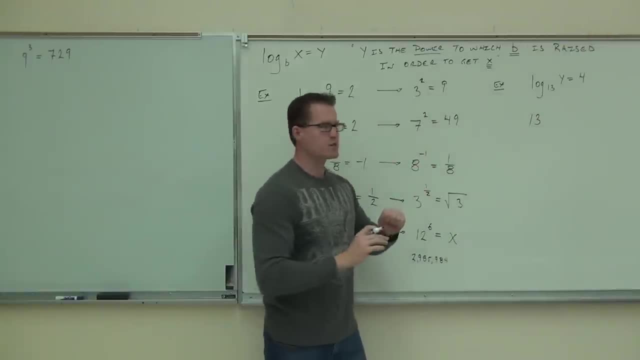 So you write 13 first. That's your base. that doesn't change. What is your exponent here, What's your power? 1. So should I have 13 to the y or 13 to the 4? To the 4.. 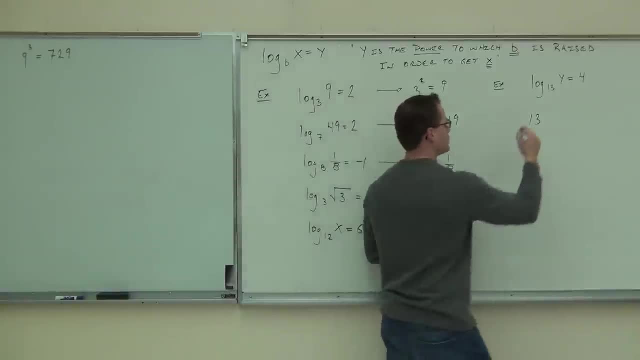 To the 4.. And what's that? equal Y, Y. What does your head feel okay with translating that? Do you have a good idea about what these logarithms are coming from? They're just a different way to write an exponential. 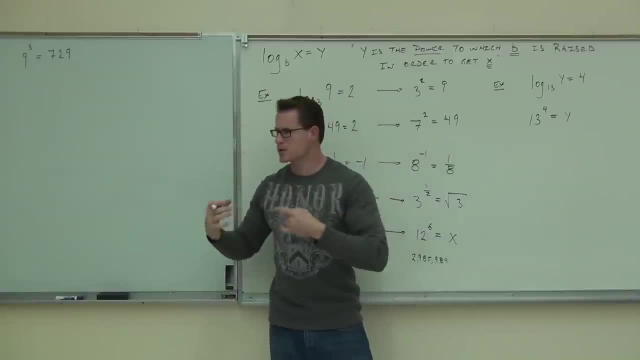 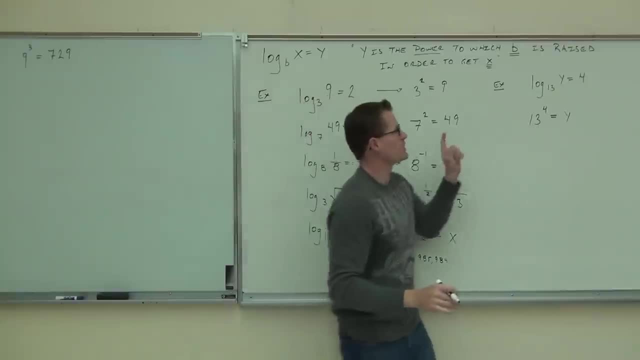 That's why we do that. That's why we do that. The whole idea was trying to find an inverse of some exponential function. We'll talk about inverses graphically in just a bit. Now, one other question is: can you go backwards? 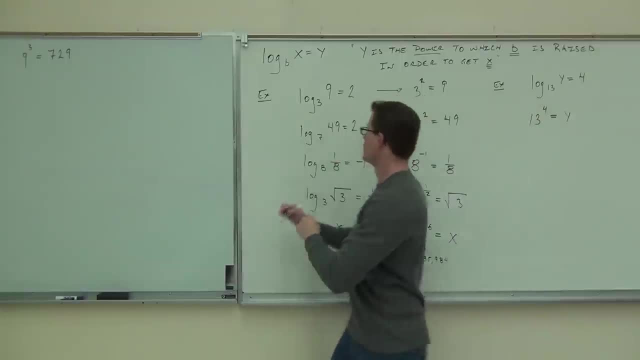 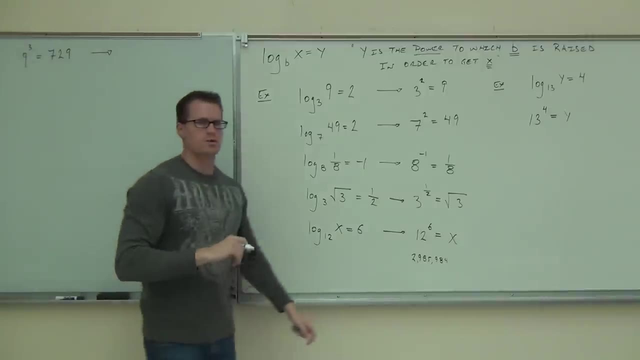 Can you go from this stuff to this stuff Or that to something that has a logarithmic? This is exponential notation. We're going to try to write this in logarithmic notation. Firstly, if you're trying to write logarithmic, you better have a log. 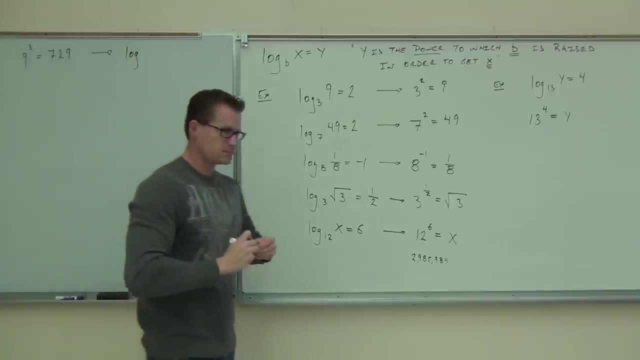 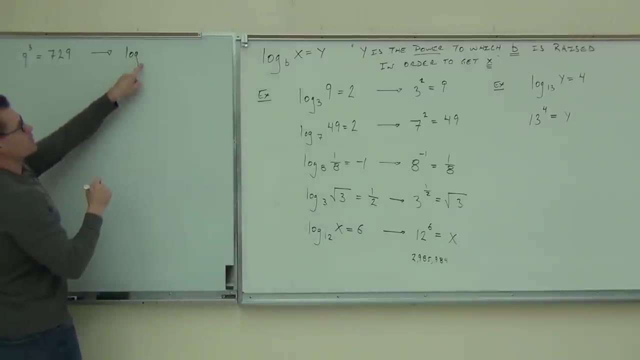 Okay, What is your base here, ladies and gentlemen? Nine, Nine. So where does the nine go? Option one, option two: option three: One One. Notice how it's a little bit below the log. Okay, It is a subscript. 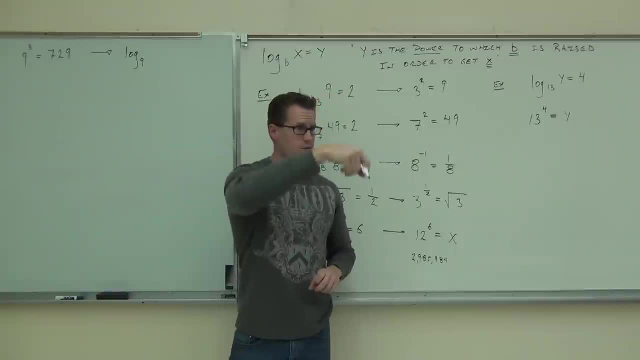 So when you write in your paper, don't just put log nine at the same level. That nine goes a little bit below it. Do you notice how I've written it? It wasn't a mistake. It's below the log just a little teeny bit. 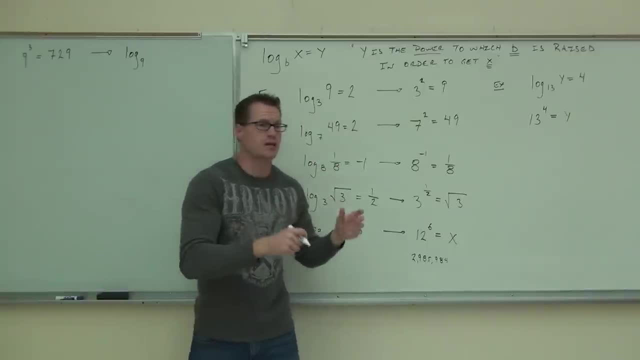 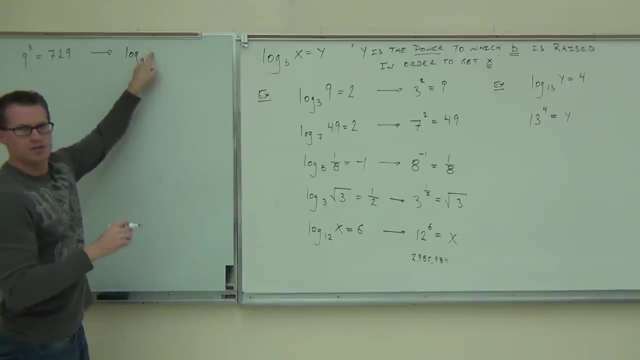 Do you guys see that? So don't write it right next to it. That's a little mistake there. So we've got log base nine. Okay, now what number goes here? This is the key part that you've got to know. 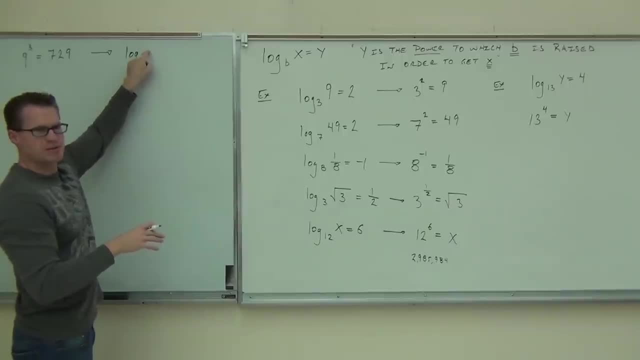 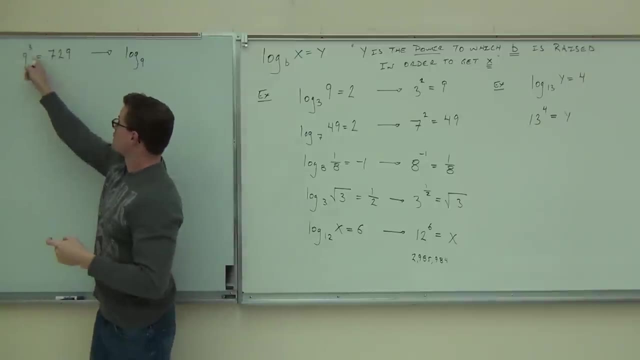 Most people are going to be able to get the base just fine. It's this one that people mess up. if they make any mistake at all, Is it going to be the three or is it going to be the 729?? 729.. Yeah, this shouldn't look exactly like this. 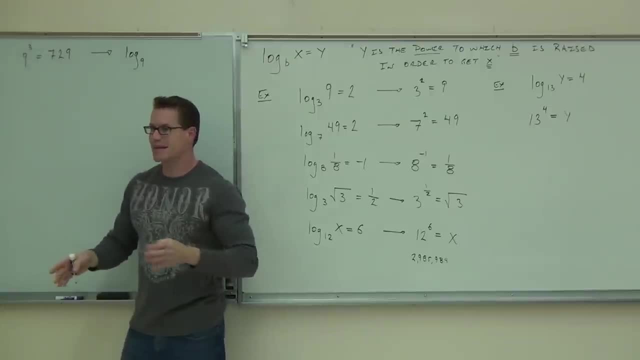 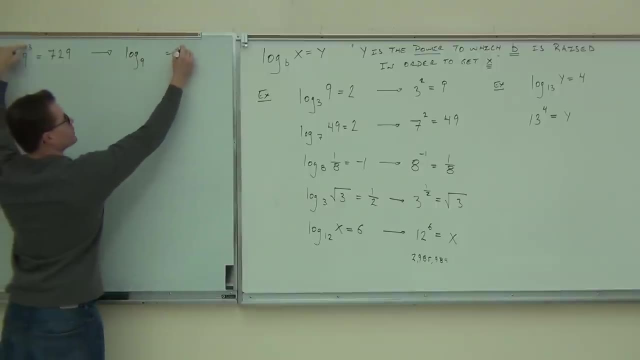 It shouldn't just have a log in front of it and have it right. That's not the same thing. It's got to change a little bit, And what we know is that the base does go here, The exponent, though, goes over there. 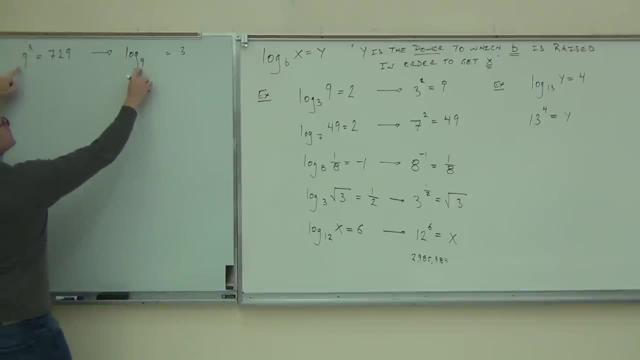 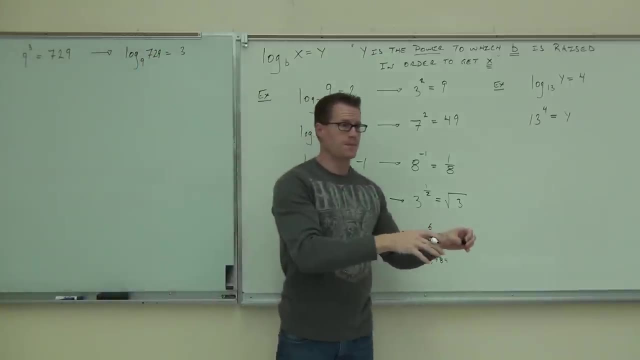 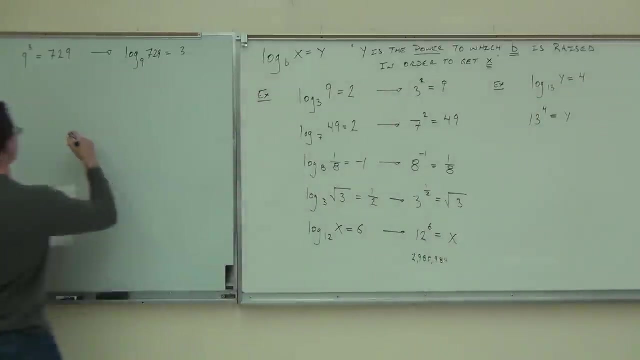 So we can say: log base nine to the third power gives you what's right there- 729.. Are you guys okay going that way? All right, It's different, isn't it? It's something unique for us. Let's try a few more. 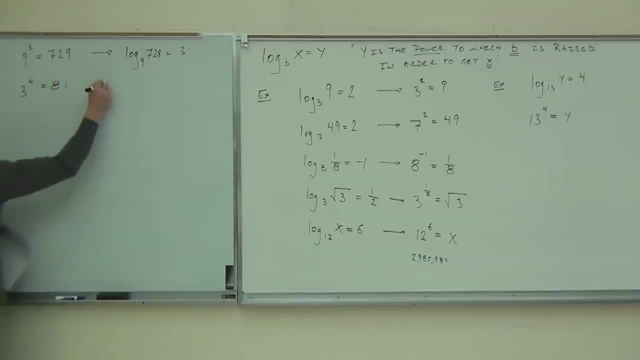 How about three to the fourth equals 81?. Let's write that one. Can you tell me log base what? here folks Log base what? So three is going to go right here. What number is going to go here, the four or the 81?? 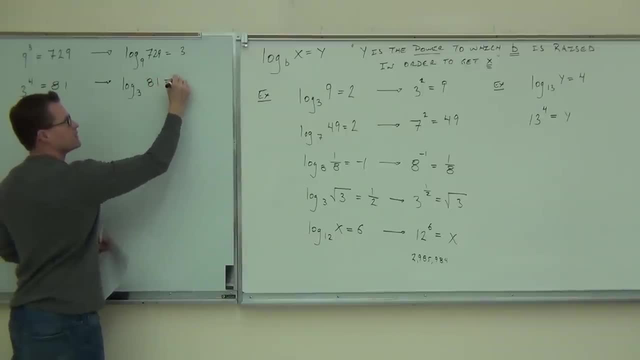 81.. And that gives you what Four. Notice how they do say the same thing. This says: four is the power to which three is raised in order to get 81.. Four is the power to which three is raised in order to get 81.. 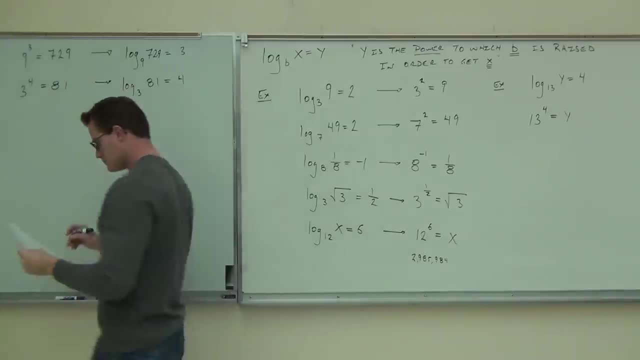 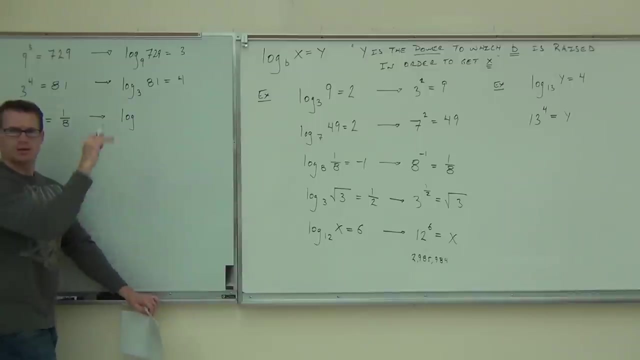 They say the same thing, It's just a different way to write it. Let's try a few more here. Two to the negative, three equals one-eighth. Tell me the first number I'm going to write, please. Two, As they go at the same level, a little bit below the log. which one? 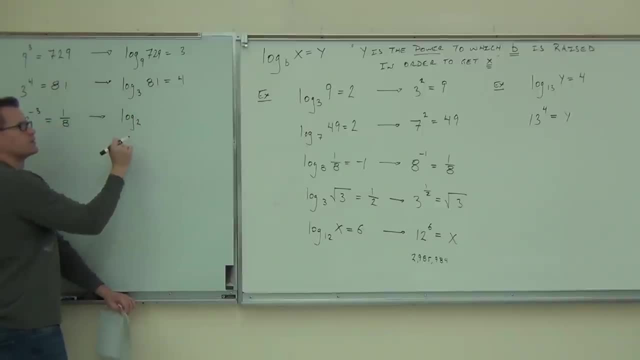 Two, So two. What number is going to go right here now? One-eighth, One-eighth Equals Negative three. Negative three. Negative three, Three, Because that's your power. By the way, that is a true statement, right? 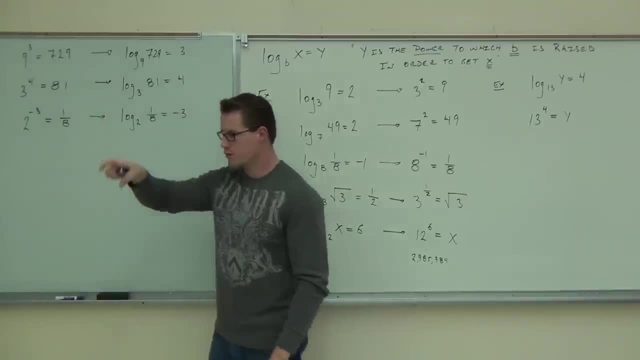 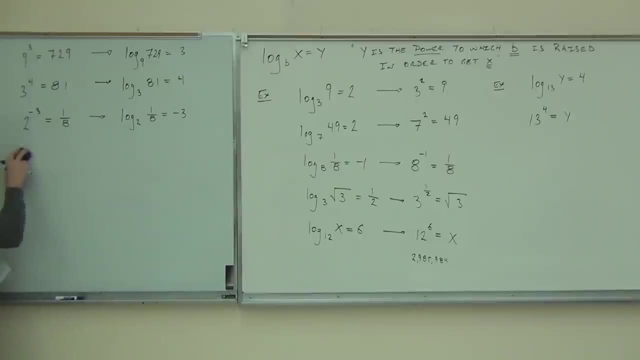 Two to the negative three equals one-eighth. That would be one over two cubed, or one over eight. Hey, what's a one-third power? mean again. Oh, this is coming back to you, this chapter 10 stuff that we had a couple of chapters. 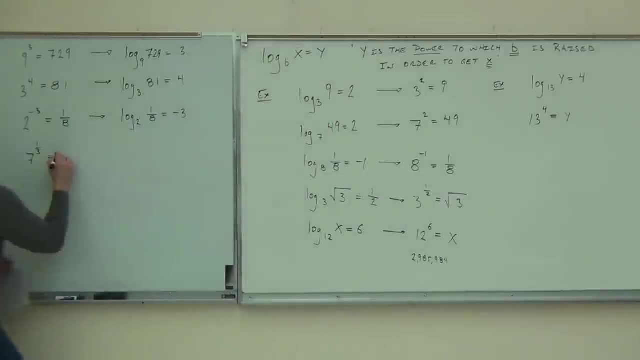 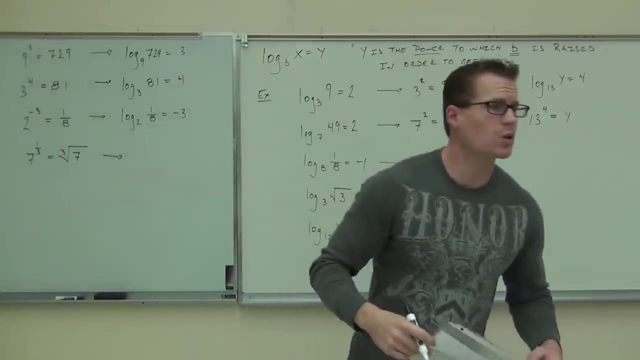 ago. What is that? It's a cube root of seven. That's a true statement. Let's see if we can write this in logarithmic notation. Everybody in here, What is your base, please? Seven, So we should have log base seven for sure. 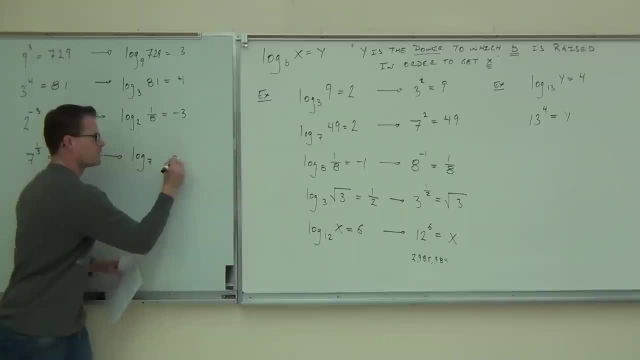 That's absolutely right. Can you tell me what goes on this side of the equal sign? everybody One-third. Where do you get the one-third From the power? Aha, And the cube root of seven must go right there. Yes, 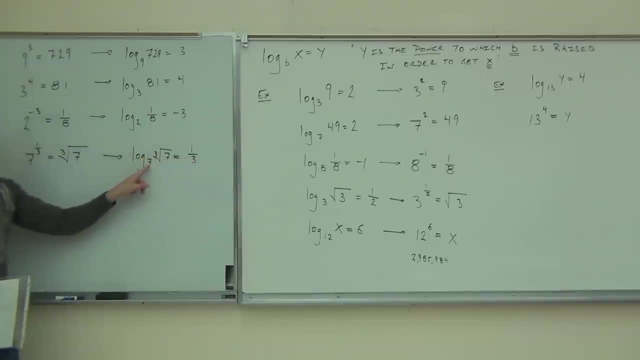 It must go right there. It says one-third is the power to which seven is raised in order to give the cube root of seven. We'll try one more together. I'll give you a couple on your own and we'll move on. 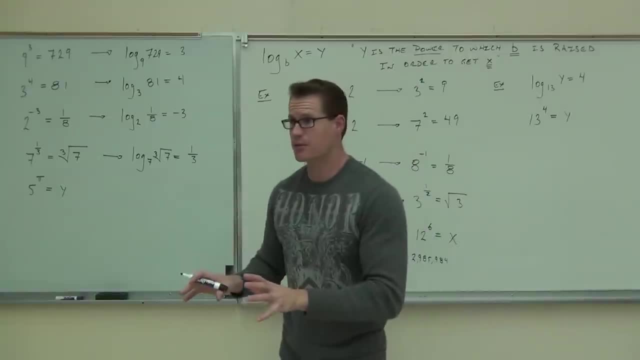 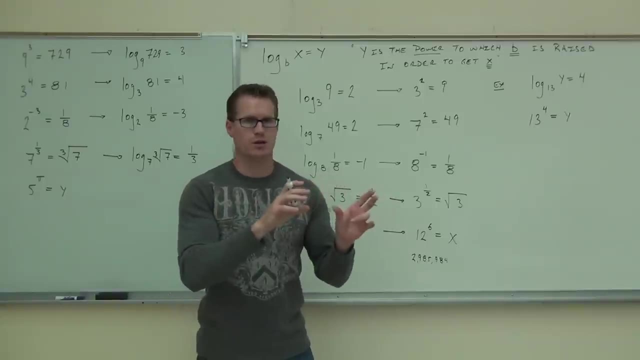 You know, right now we're actually, have you noticed, we're not doing any math. We're really not doing any math. I may have asked you a couple questions here, But really this is all just symbolic translation. You're translating from exponentials to logarithms. 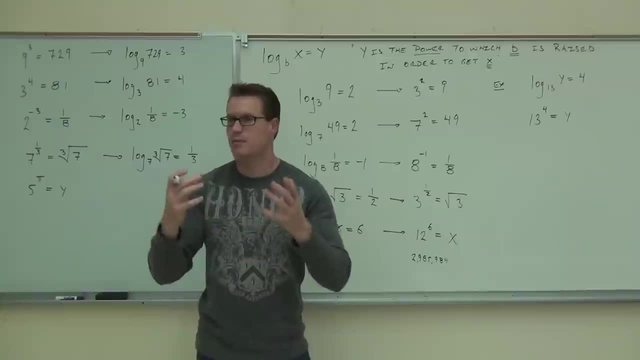 or logarithms to exponentials. Have you noticed that We're really not doing much except translating here? So really it's all about symbols. Does it matter if I give you a pie up there? You should still be able to translate this. 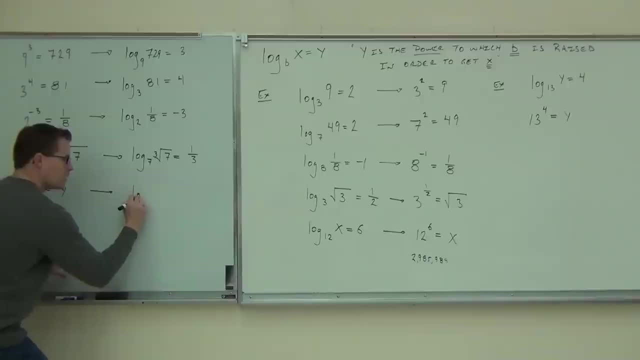 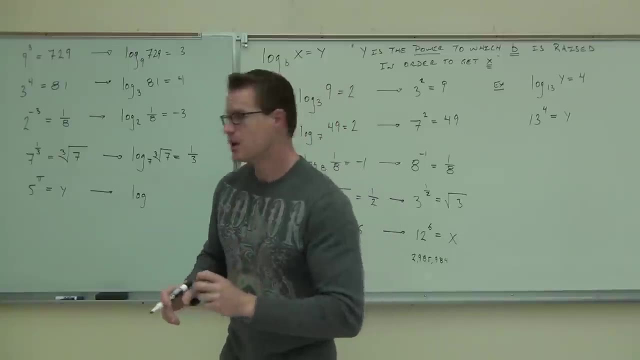 So let's go ahead and try that. If I'm translating this, of course, in logarithmic notation, I've got to have a log. You just need to be able to identify your base and your power and where those things go. So what is going to go right here for me, please? 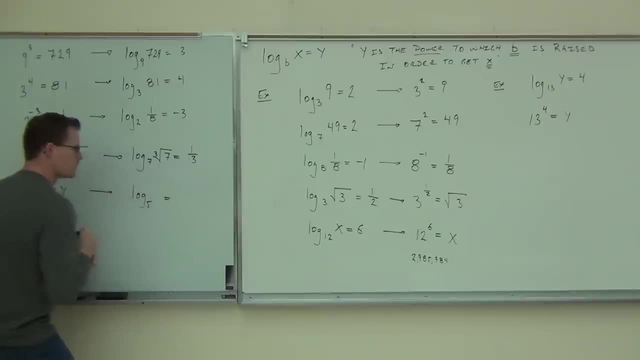 Pi Good. What's going to go right here for me, Y The Y, Mm-hmm. And over here, Pi Good, Because you're just making a base. go here a power. go here, and what the base. 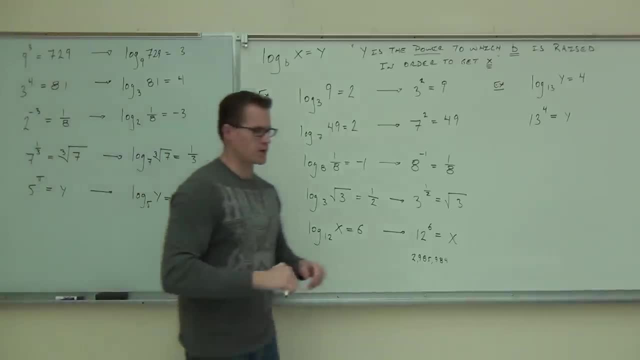 to the power equals goes right there. It's a different way to write your exponential. Okay, try two of these on your own. Let's do 5 to the negative. 3 equals 1 over 125.. I want you to translate that. 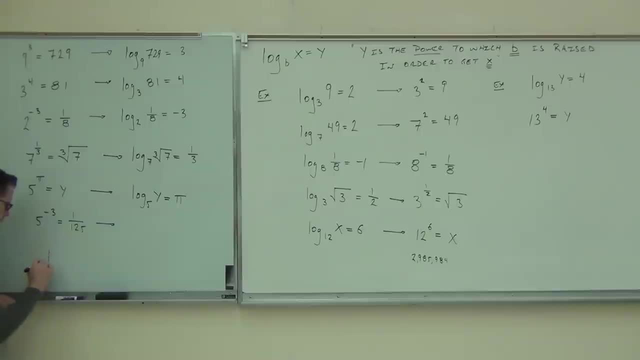 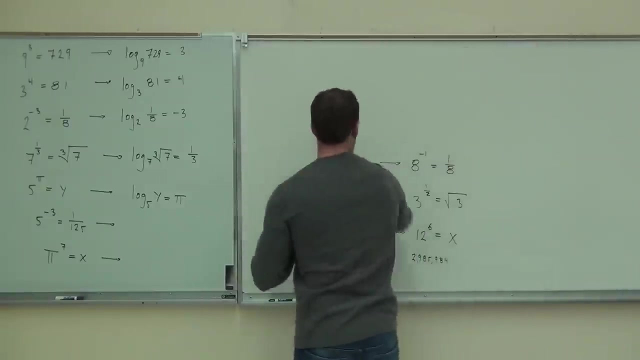 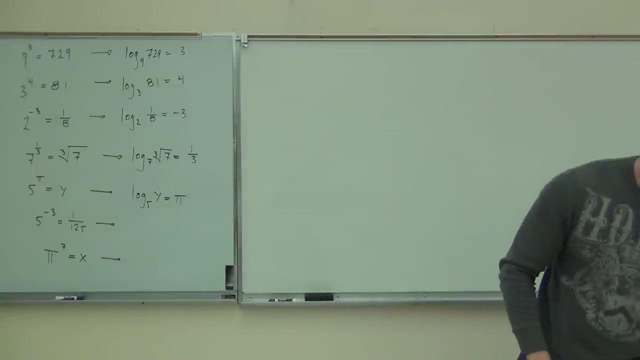 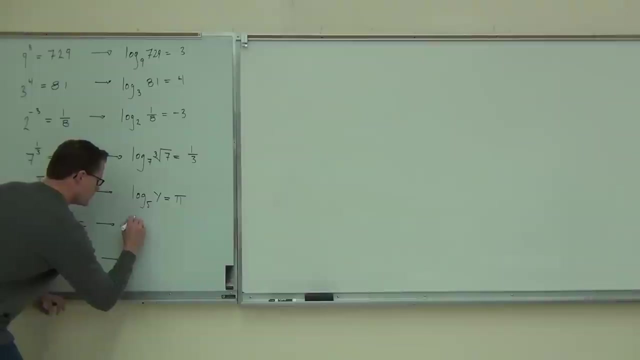 As a logarithm in logarithmic notation. and this one: Aren't you glad we don't deal with that stuff for real in this class? huh, That'd be crazy, Although I'm sure you can handle it. Well, we're supposed to have a log in each case. 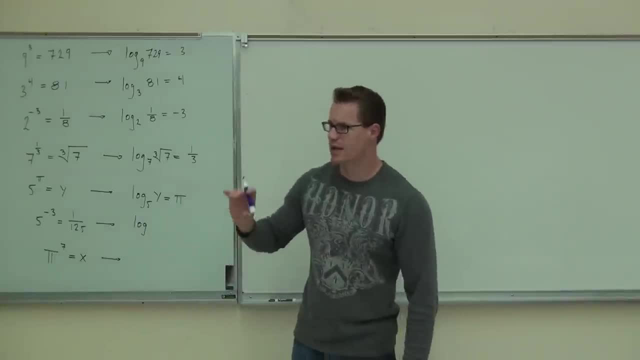 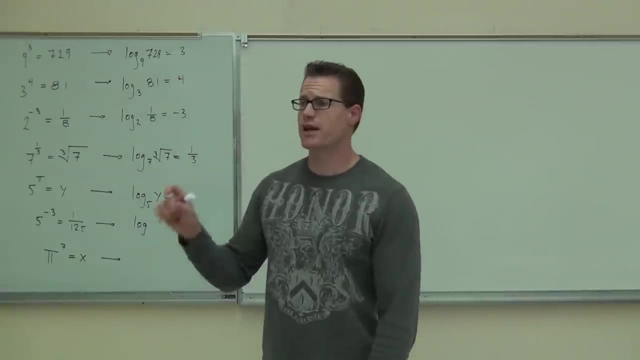 because of course, we're dealing with logarithmic notation. We're translating exponentials- these are all exponentials- into logarithmic notation. It has that little log in front of it. Again, you just got to find out what your base is. 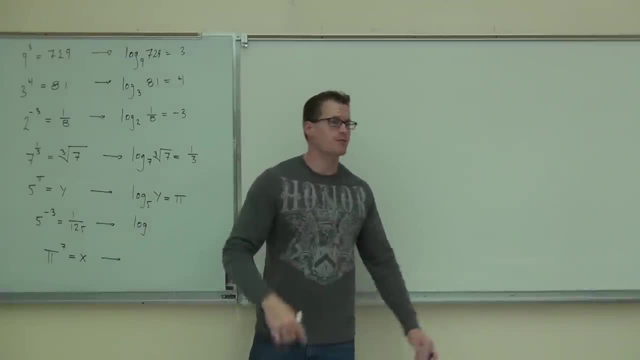 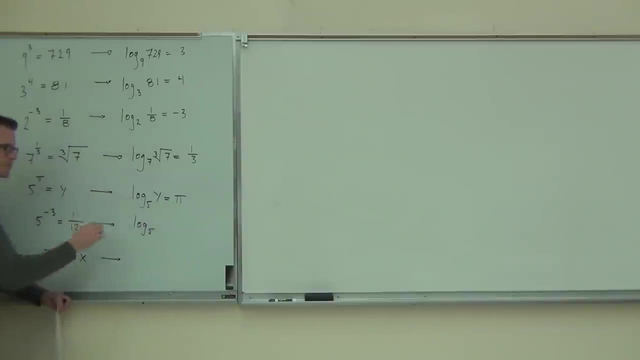 put it in the right spot, Find out what your exponent is, put that in the right spot and you'll have this thing down. So in our first case here, this is going to be log base what 5.. Good, Log base: 5 of what is what goes here. 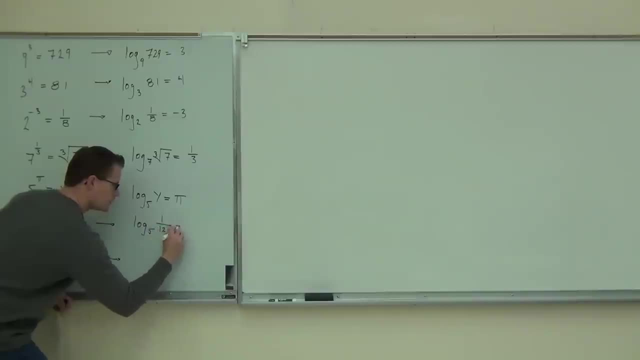 1 over 125.. Equals how much 1 over 125.. Here's how you say this again. Practice this with me in your head. You'd say: log base 5, say it, say it, Log base 5.. 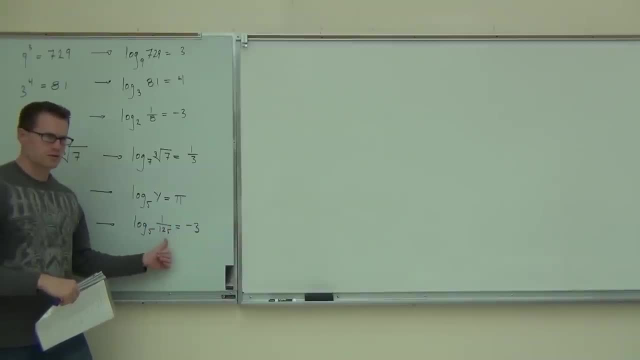 Of 1 over 125.. 1 over 125.. Equals negative 3.. Equals negative 3.. That's how you say that Log base whatever of something equals. you don't say log of 5 of That doesn't work. 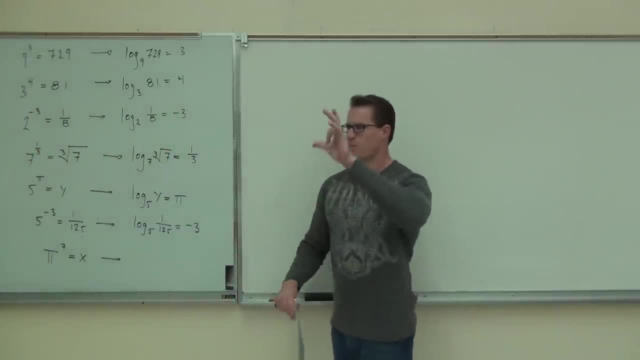 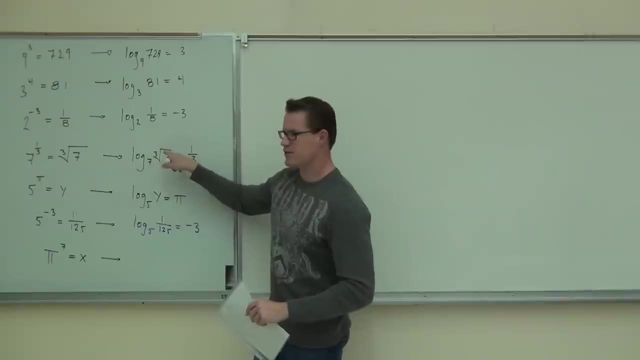 Doesn't flow right, Doesn't sound good. right Say: log base 5 of 1 over 125 equals negative 3.. That's how we say these logarithms. This would be: log base 7 of cube root of 7 equals 1 third. 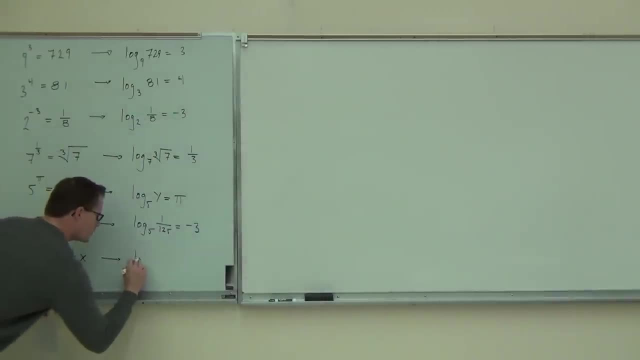 That's how you say these logarithms. Okay, last one. we have log log base. what Pi? Oh, that's weird Log base. pi Of Pi Pi Equals Pi Pi. Perfect, That's exactly how you write them. 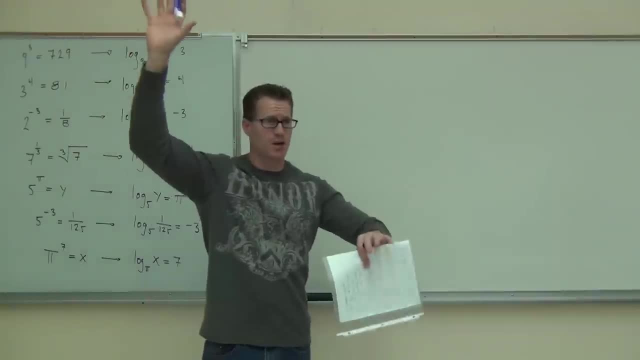 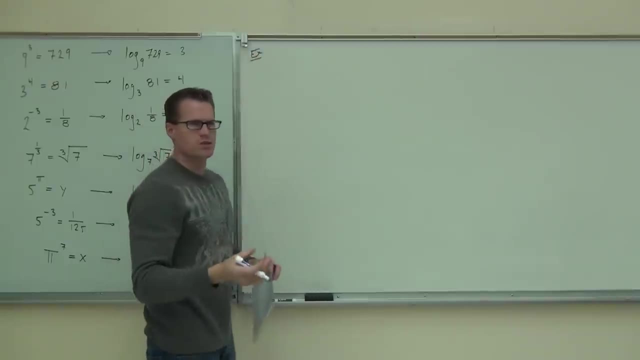 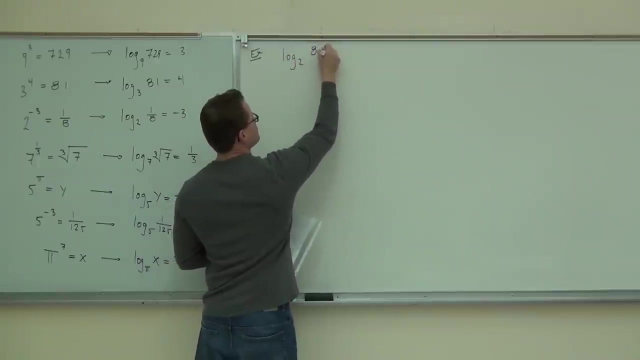 Raise your hand, if you feel okay. Translate between logarithm and exponential, and backwards. Good for you, That's fantastic. Now could you, since you now should have a decent idea of what these logarithms do, could you find out what some missing information is? 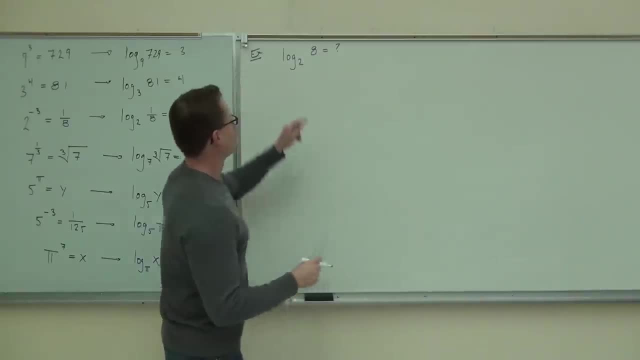 For instance, if I ask you that question, can you tell me what that is? If you had to think about it, what does this stand for? Is this a base? Is this a power, Or is this what a base to a power equals? 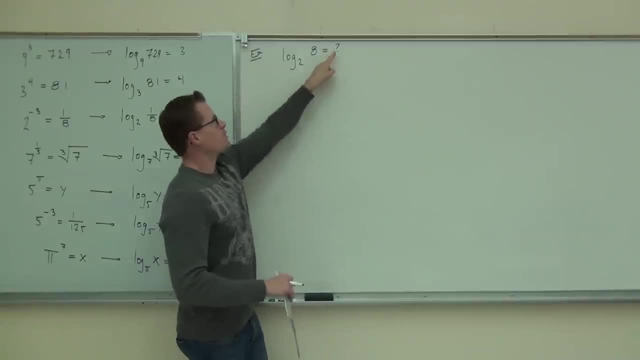 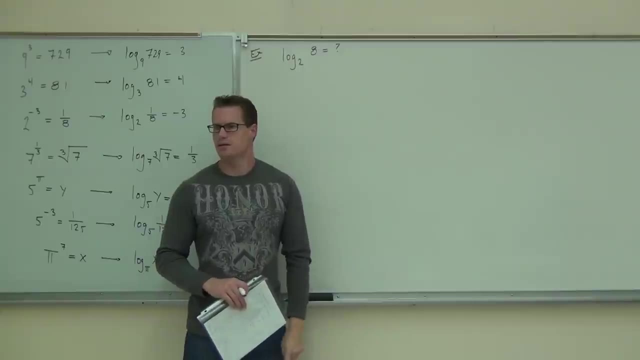 That's a power. That's a power It says. what this says is: what power do you got to raise 2 to in order to get 8?? What power is that? 3., 3. 3. 2 to the 3rd equals 8, right. 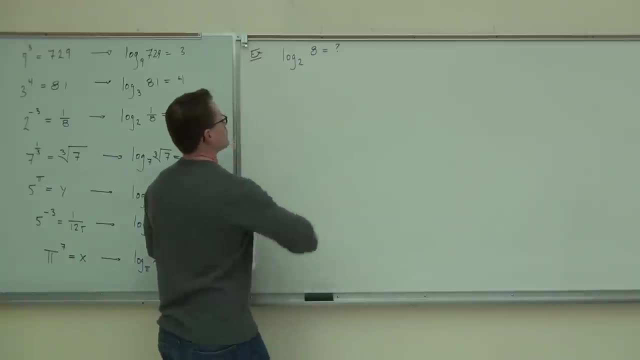 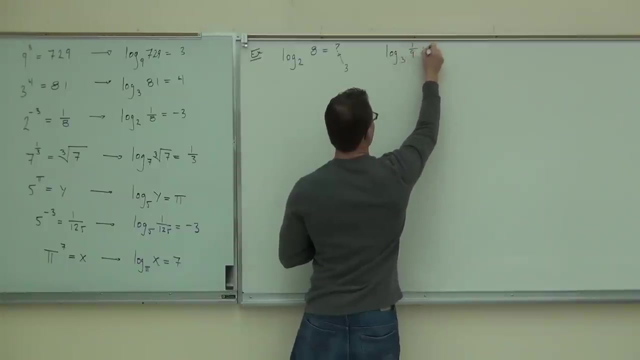 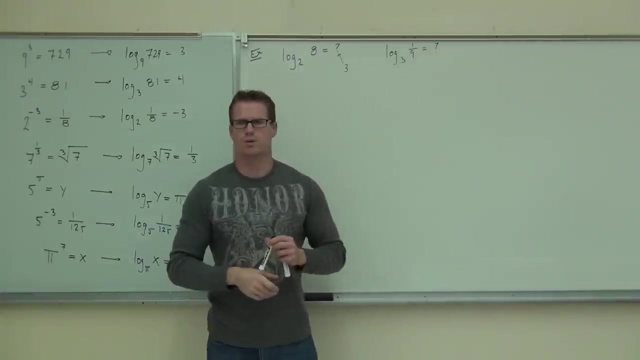 So you know for sure that this right here, That's got to be a 3. It has to be, Otherwise this thing's not going to work. How about this one Log base? 3 of 1, 9th equals what? 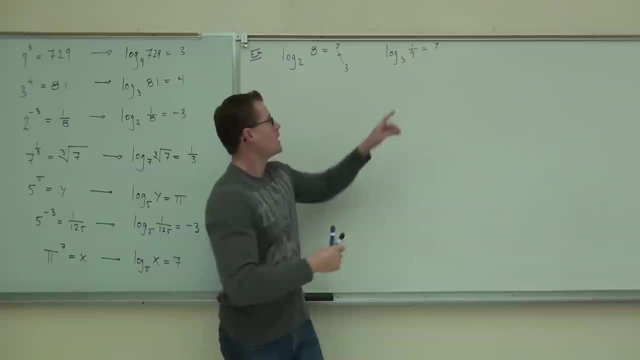 Oh Well, here's how you think about this. 3 to what power gives you 9?? 2.. But it's on the bottom. It's on the bottom of a fraction. How do you know? It's going to be negative 2.. 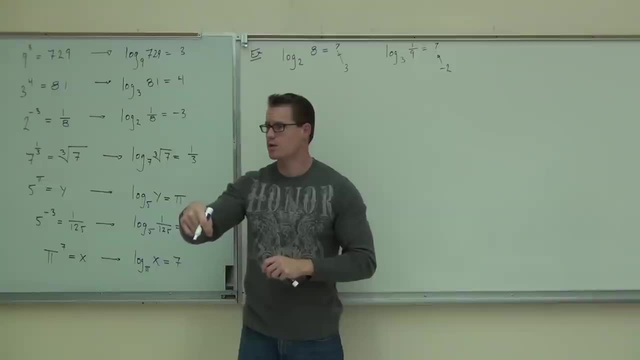 You see why it's negative 2? 3 to the negative 2,? well, that's going to give you 1 9th. Then negative will move to the bottom of a fraction. 3 squared is 9.. Well, how about this? 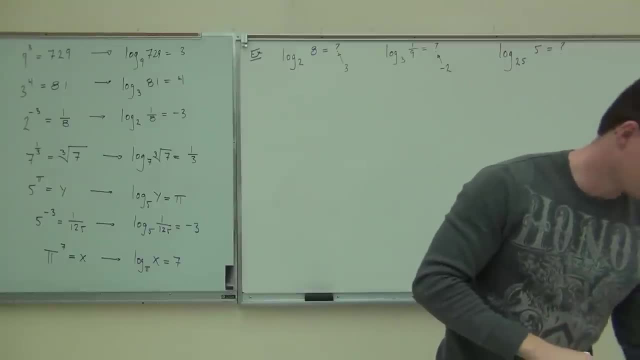 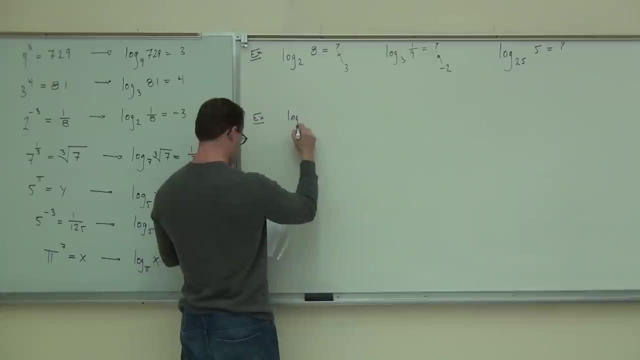 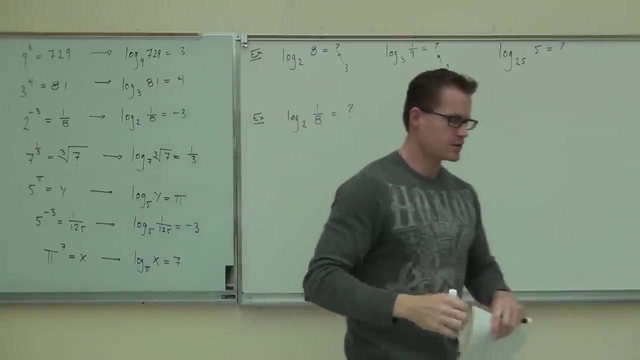 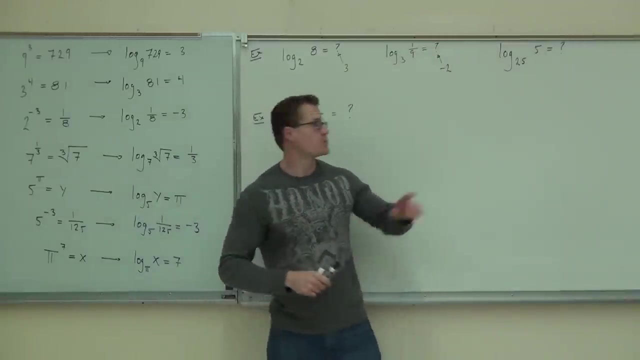 Don't say it out loud, Just think about it for about 10 to 15 seconds. I want you all to kind of think for a minute. It's a reminder for all of us here. Will you work or will you not? What next? 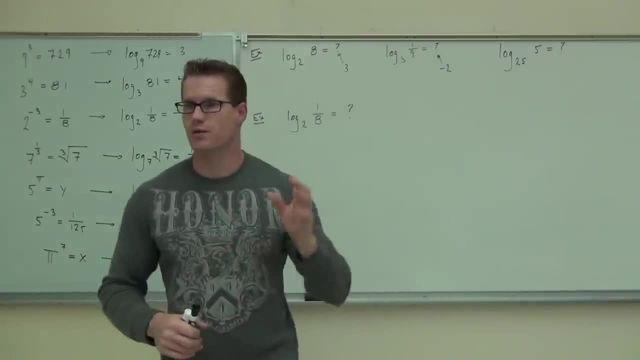 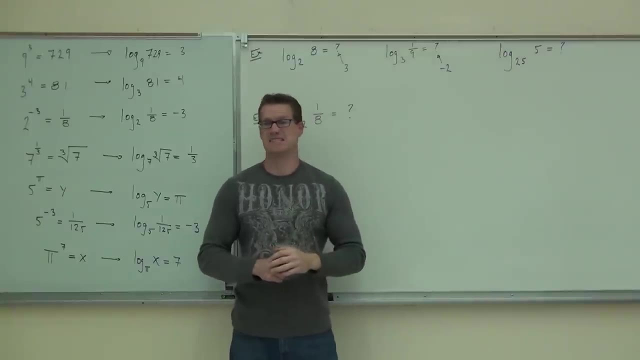 Log base: 25 of 5 equals 6.. with the power It says, 25 raised to what power gives you 5?? What do you think? Can you square 25? It's going to give you 625.. That's not right. How do you get from 25 to? 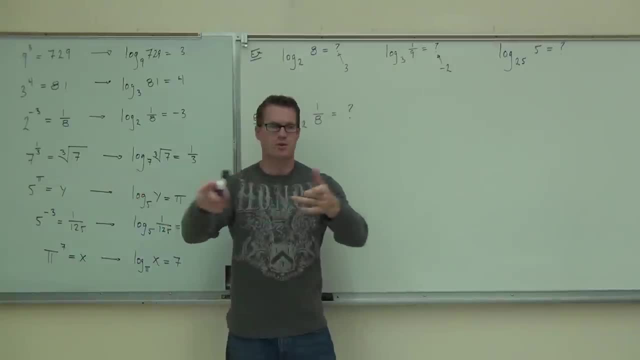 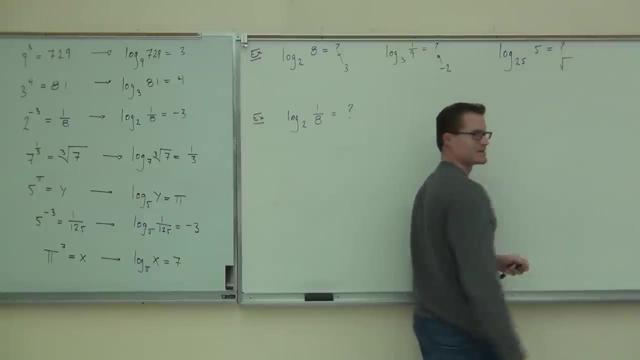 5?? I hear some people say square root. Some other people are saying one half. Is that the same thing? However, you can't write this right. You can't just write that, because that's not a number We need to go. oh, it's square root. Yeah, it is a square root to get from. 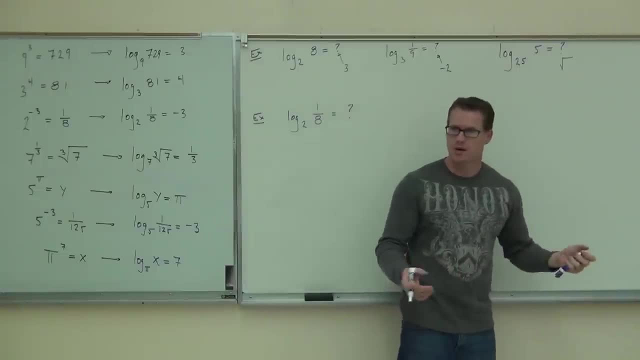 here to here. You just need to know how to represent that as power. So if a square root is the way you get from 25 to 5, then that means that this thing is a one half And in fact 25 to the one half equals 5.. Why don't you try this one on your own? Tell me what. 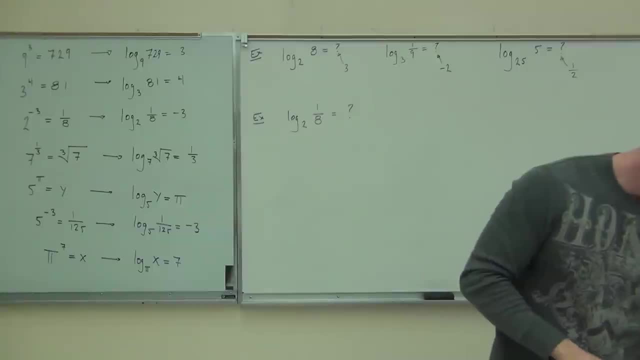 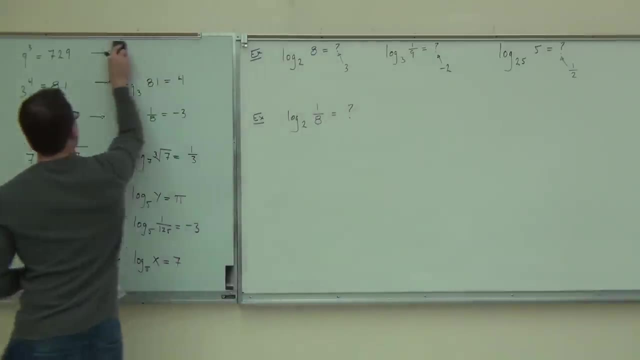 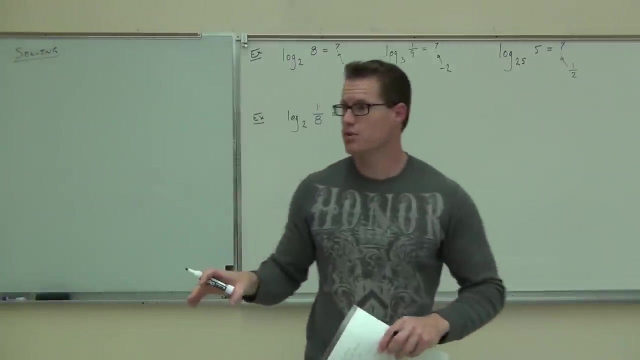 that is, Just write it on your paper. You don't have to say it out loud. Have you found it? Two: to what power gives you one? eighth: Have you thought about it? Okay, the way maybe you think through this instead of just jumping right into it: think. 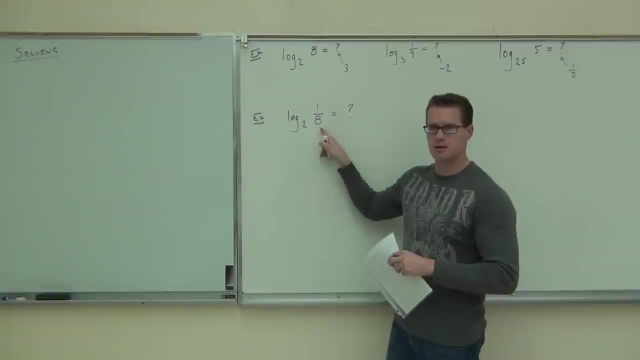 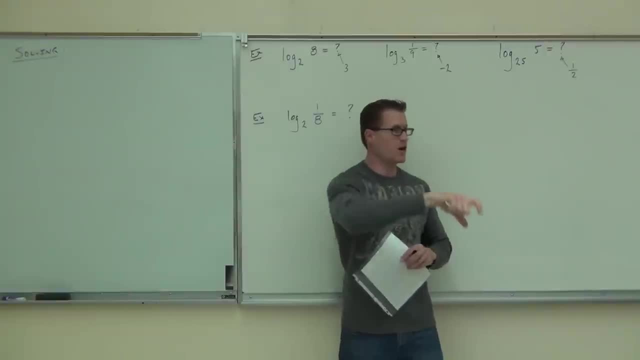 that? What power gives you that? What power gives you that one onde? you would have a three right there, But you have one over eight. How do you change that to the bottom of a fraction? That's what that negative exponent. so that's going to be negative three. How? 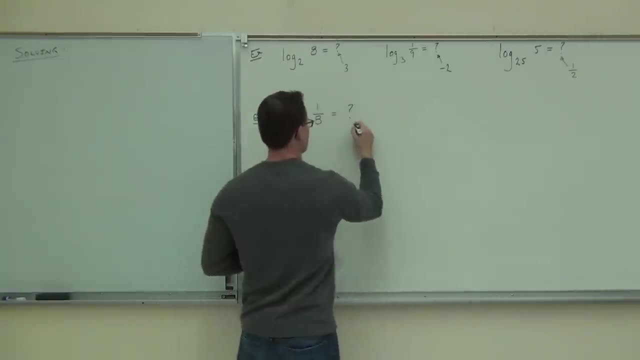 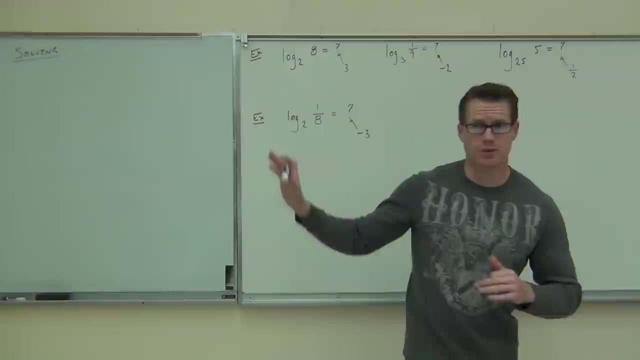 many people have thought about negative three. That's good. All right, That's mostly done. Now there is another thing that we can do. I really I kind of just had you do it. We are going to solve some of these logarithms. Talk about solving. You did it in your head. 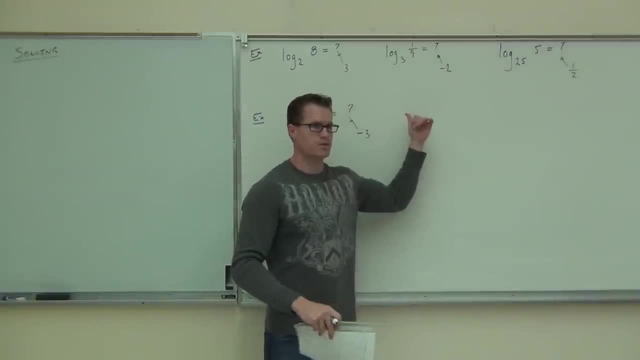 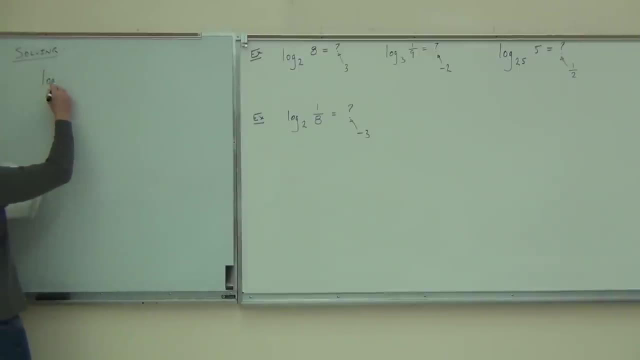 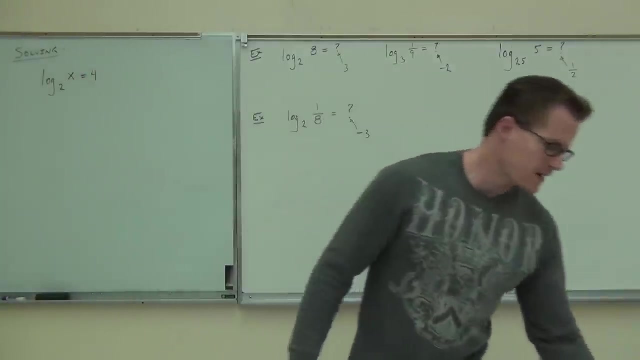 just right now. You did several of those by yourself, right? It wasn't too bad. We are going to learn that, in order to solve some logarithms we are going to solve some of, In order to solve your logarithms, one very nice thing that you can do instead of just. 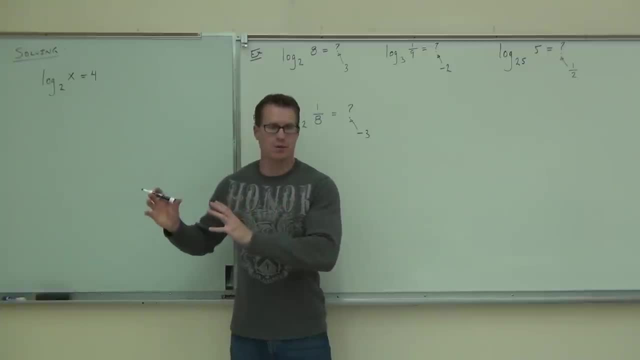 thinking about it in your head. since we have a variable up there right now, we could actually write these as exponentials and solve them. So, in order to solve a logarithm, what you're going to do is set it up as an exponential. 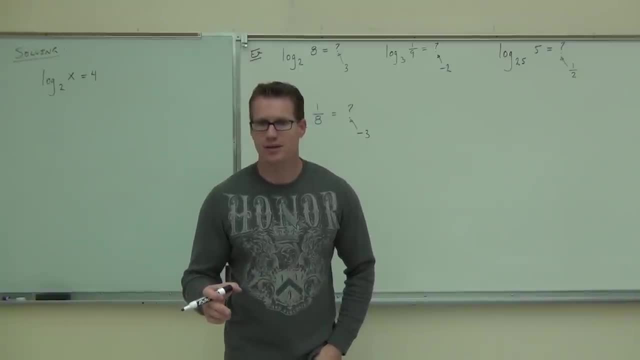 How are you going to solve logarithms, Exponentials? You know how you solve exponentials: Logarithms- It's their inverse operations, right? I want you to think about this: When we solved the inverse of an exponential, we got a logarithm. 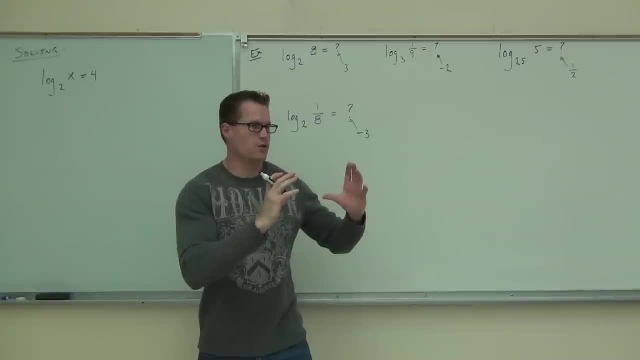 Doesn't that make sense? If you found the inverse of a logarithm, you know what you're going to get. An exponential Inverses undo each other. How do you undo multiplication, Division? How do you undo addition, Contraction? 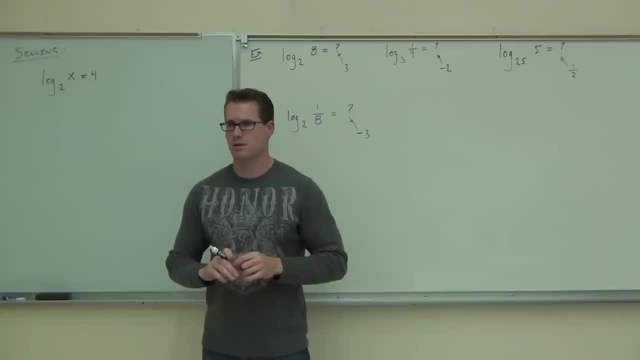 How do you undo a square root, An exponent of 2,? as a matter of fact, You square it. Does that make sense? You do that because they're all inverses. Now, the way that you're going to get rid of an exponential is with logarithms and the 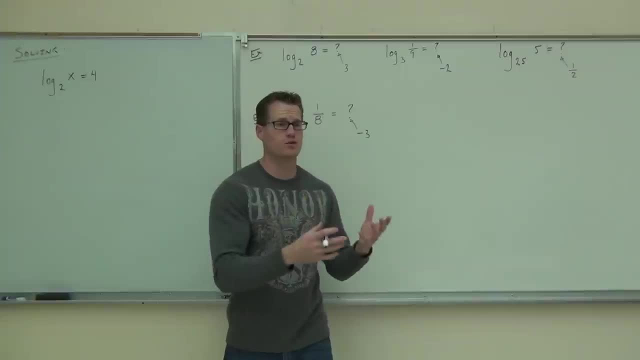 way you're going to get rid of logarithms is with an exponential, Because those things are inverses. they work just like multiplication and division or addition and subtraction, or squaring and square root. They undo each other. So, as long as you can translate- that's why we spent so much time just translating right- 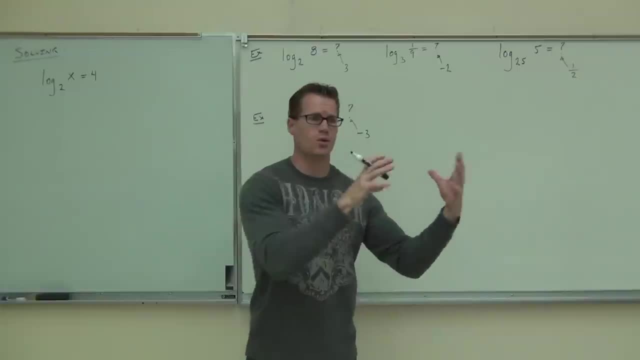 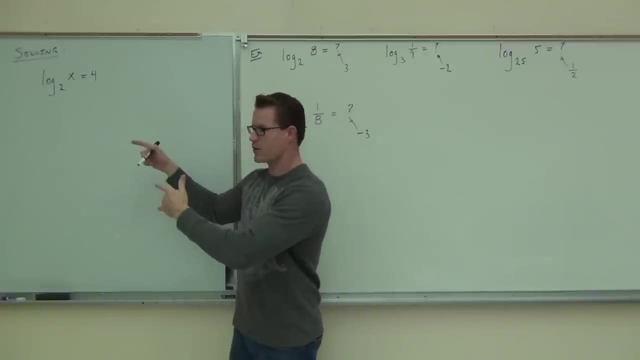 now, as long as you can translate from a logarithm to an exponential or an exponential to a logarithm, you're going to be able to solve these things. You ready to see how that works? So now that we have a variable up there that we can work with, let's go ahead and see if. 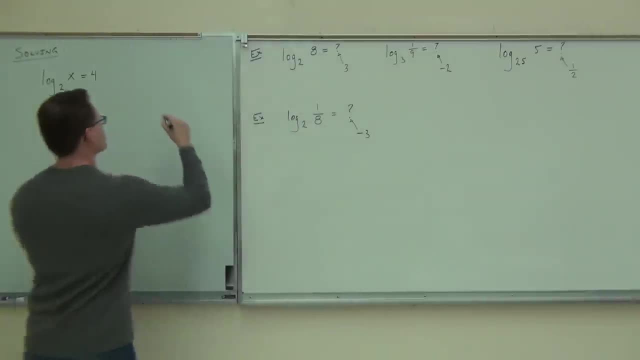 we can write this as an exponential, So your first step here is to write as an exponential: Okay, So, Okay, Okay, Okay. So if you see the word solve and you have a logarithm, the first thing that should be: 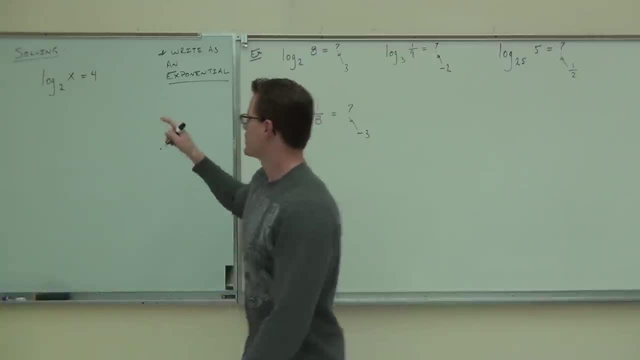 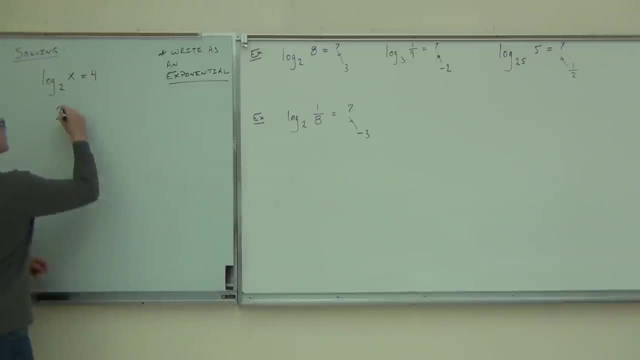 in your head is, oh, exponential, Try that. So let's go ahead and do that. What's your base here, folks? So I would write two: To what power of the x? or to the fourth Equals, Oh, okay. 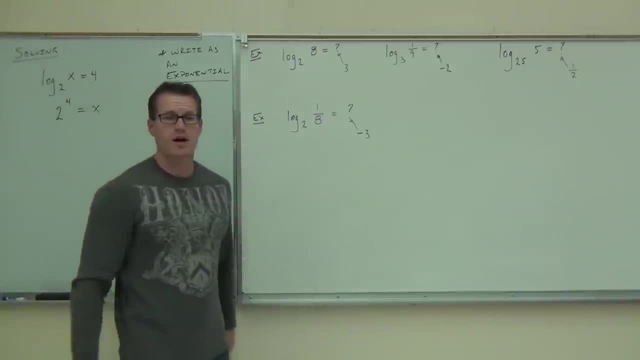 Hey, look at that. X is already by itself. Can you tell me what two to the fourth is? So as soon as you write that as exponential, that's a lot easier to think about, isn't it? As I'm trying to do that in your head, you go: oh, yeah, okay. 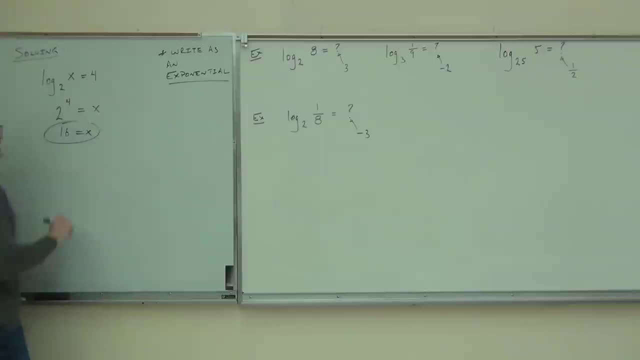 That means x equals 16. And if you go back to the logarithm that says 2 to the 4th should give you 16.. Does it work? Now? of course we can move that variable around and have it in different locations. 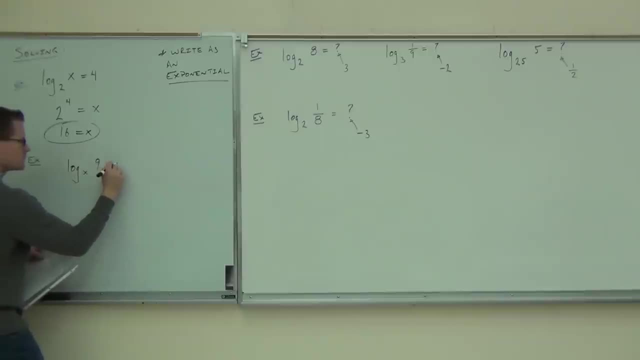 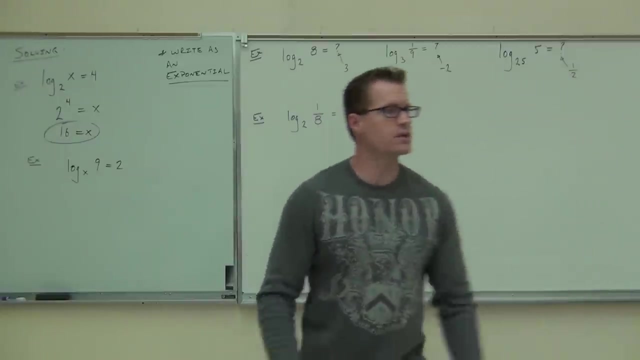 Let's try this one Log: base x of 9 equals 2.. Can you still write that as an exponential? What do you think? Well, go ahead and do it now. I'll give you about five seconds. It should be pretty quick for you to write that as an exponential. 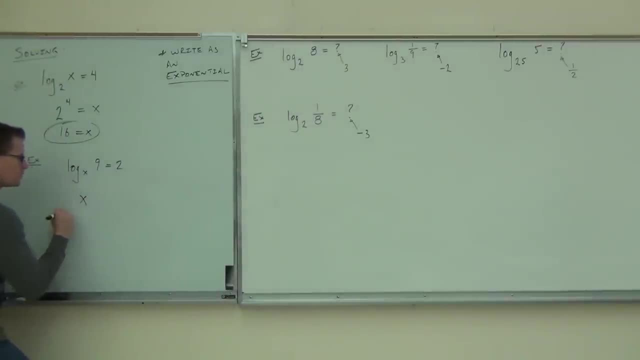 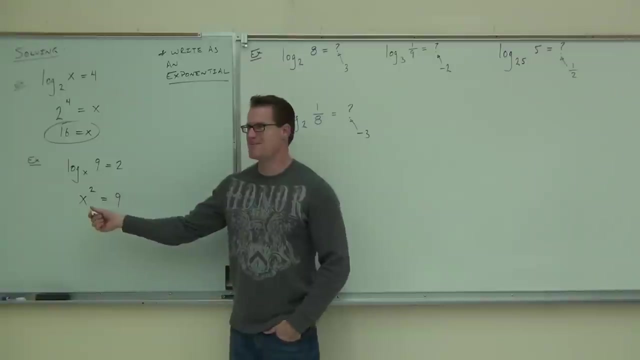 What's your base? What's your power? Equals what? Oh? Have you seen those before? Oh yeah, How do you solve that? Take a square root of it. Sure, take a square root Now. I want you to know something on the board here real quick, okay. 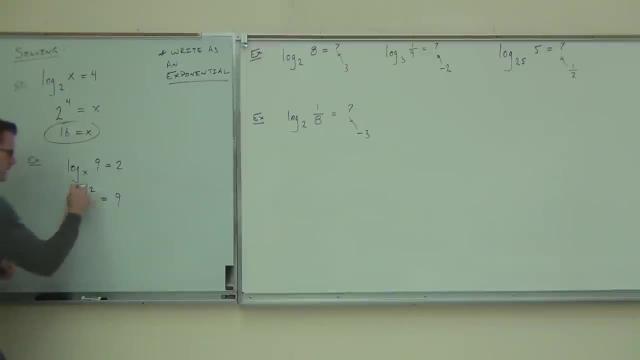 If you take a square root of this like that, right, like that, you're supposed to have what? here, Both angles equal 5 times Good And that would give you x equals 3 and negative 3.. Do you follow me? 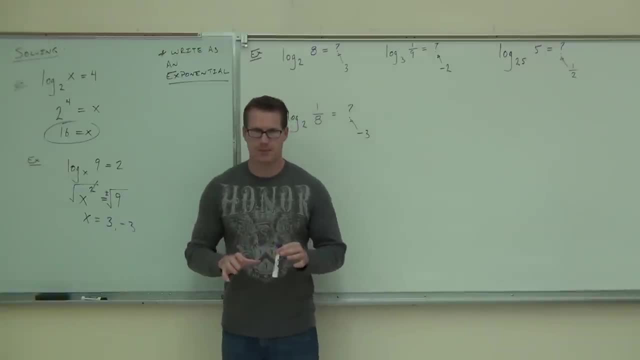 Now there's one thing about logarithms that we talked about. I had it on the board a little while ago. You probably didn't know why it was important, but here is why it's important. Notice that your x, in this case, was a base. 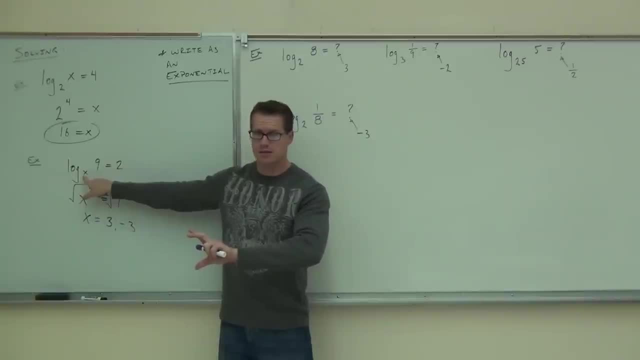 Your base has some conditions to it. First thing, it's never going to be able to move. It's going to be able to move in a little bit. Second thing, it's going to be greater than 0. Do you have that on your paper? 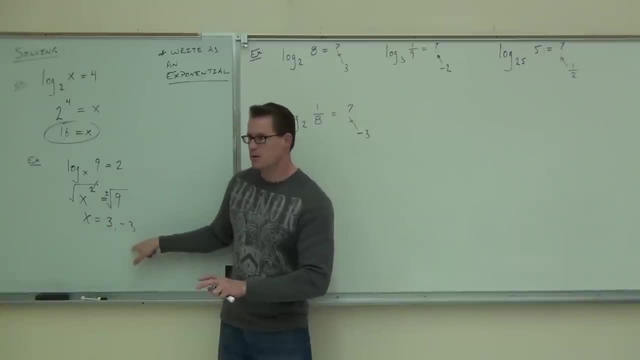 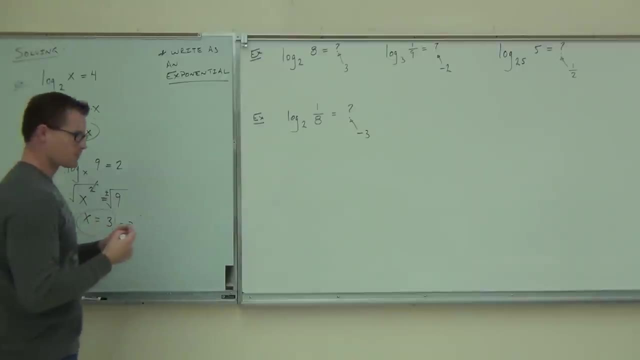 Which one of these is not greater than 0? Negative 3.. That negative 3 is a false solution. You can cross it out And it would say 3 to the second gives you 9.. Does that work for you? And that's the right answer? 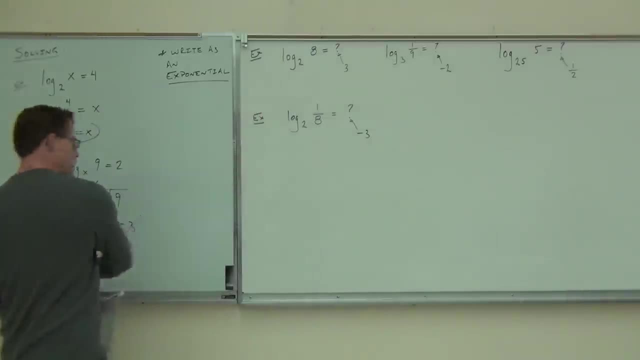 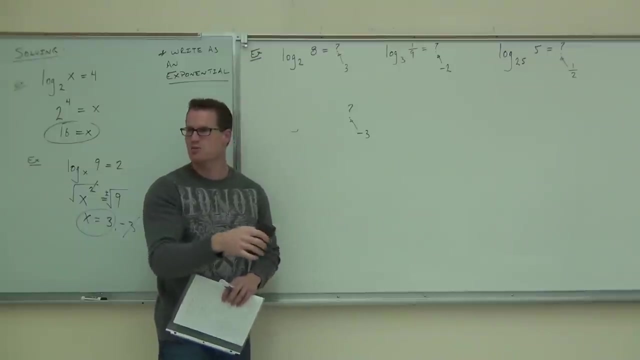 That's a correct solution. Let's try a few more up here. Are you liking this logarithm statement? It's kind of interesting. you learned something new today. right? It's not that bad, as long as you know how to get from a logarithm to an exponential. 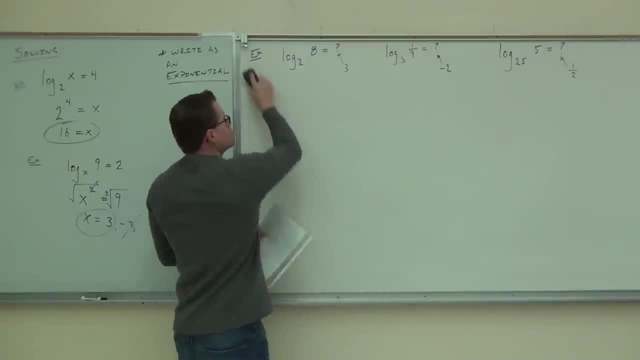 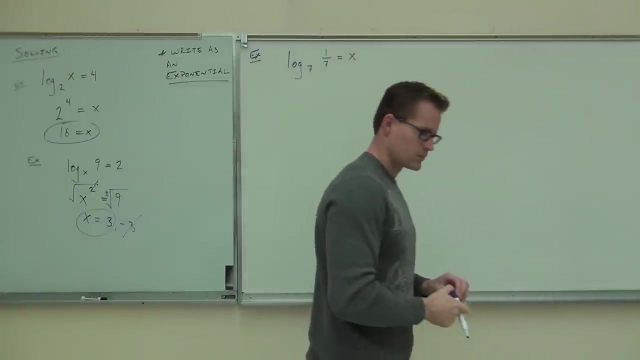 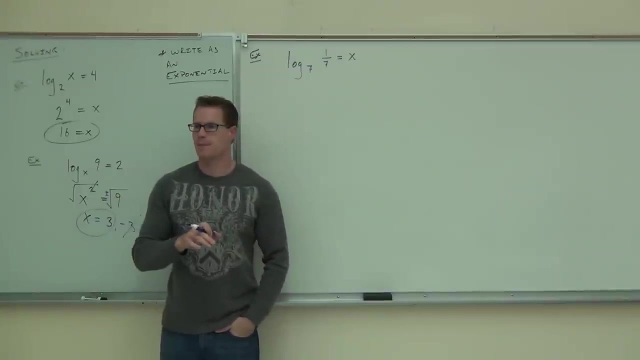 If you forget that, then yeah, it's bad because you don't know how to do it. Can you write that as an exponential Good deal? What's your base? 7. 7 is your base. What's your power? 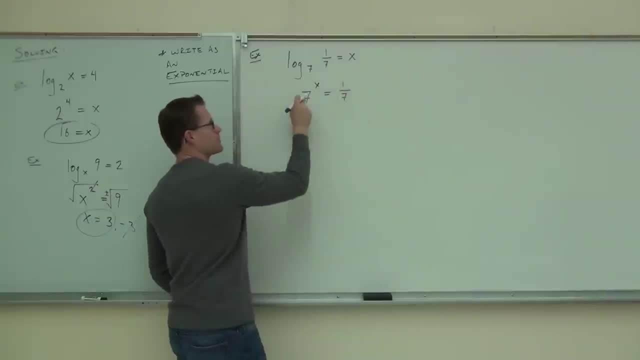 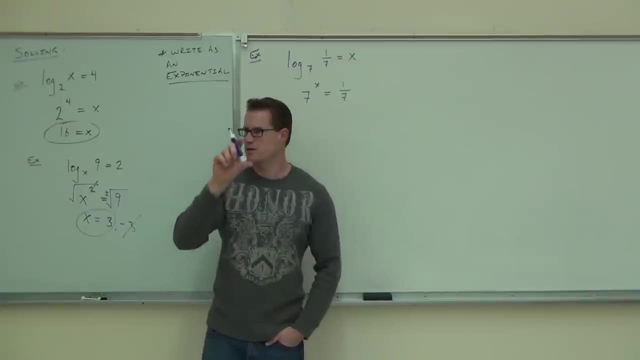 X Equals 1.. Is there a way you can do it from here to here? Do you know how much x equals 1? Negative. It's got to be negative, right? So x is negative 1.. In fact, you know what? 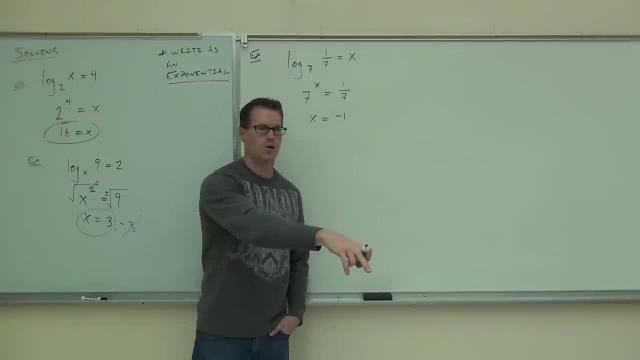 You can do this. If you look at this, this should look exactly like your homework book that you just turned in, shouldn't it? Doesn't that look the same to you? In fact, I showed you one of those negatives. I said, well, hey, the first thing you're supposed to do when solving exponentials, 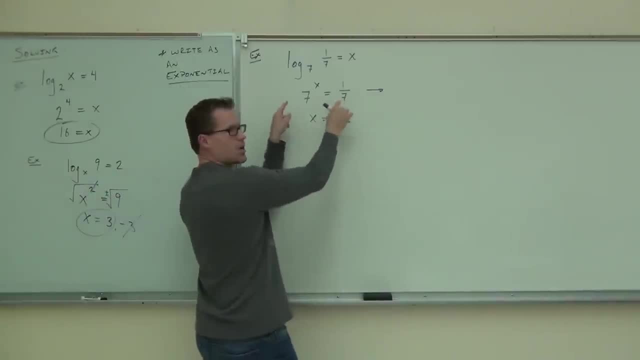 this is going to tie everything together. Look at it. The first thing you're supposed to do is get common bases, aren't you? This would be 7 to the x equals. this is 7 to the negative 1.. Remember how we moved up that number to get that negative 1?. 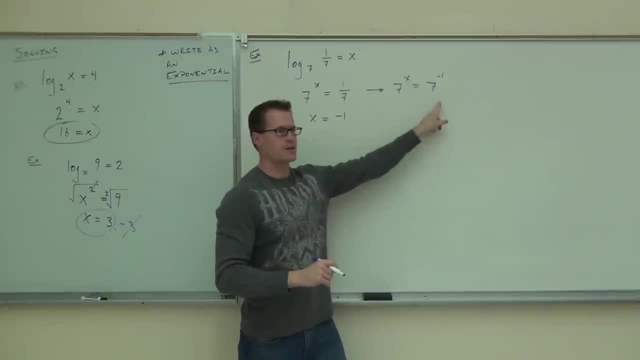 Look at that. Are the bases the same? What's it tell you? If the bases are the same, the exponents must be equal. You are solving exponentials again, Folks. we're now just translating from logarithms into exponentials, and now you have a way. 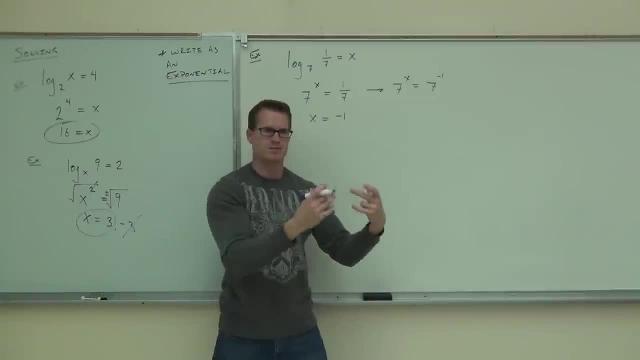 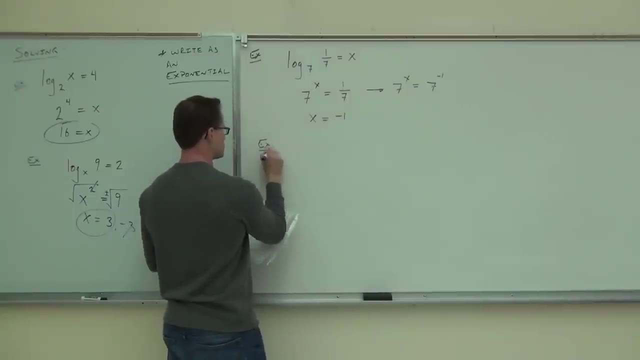 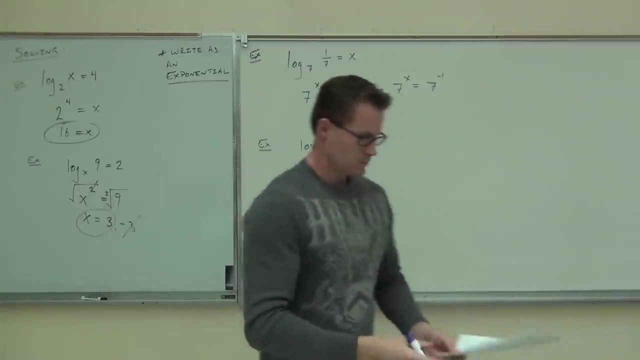 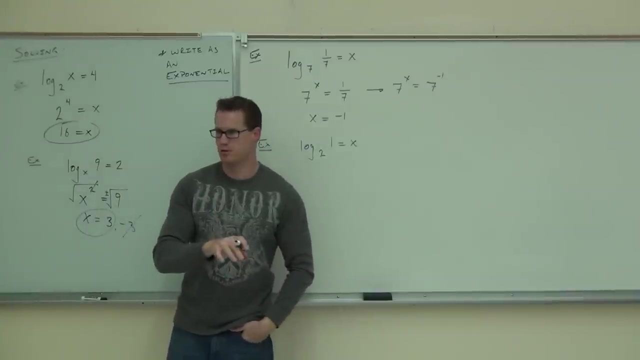 to solve. it, Isn't that kind of cool. Yeah, As long as you can translate to exponentials, you got it. Log base 2 of 1 equals x. This is going to show you something about logarithms here. If I write this as an exponential, what's your base? 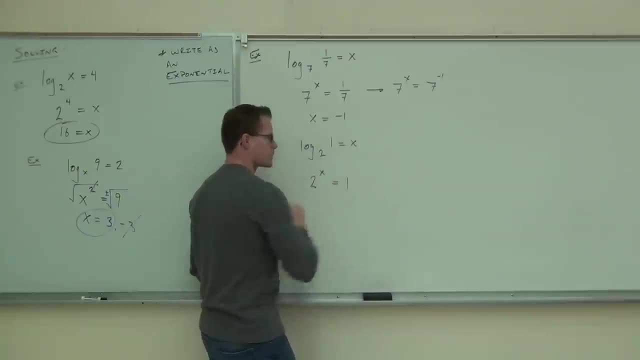 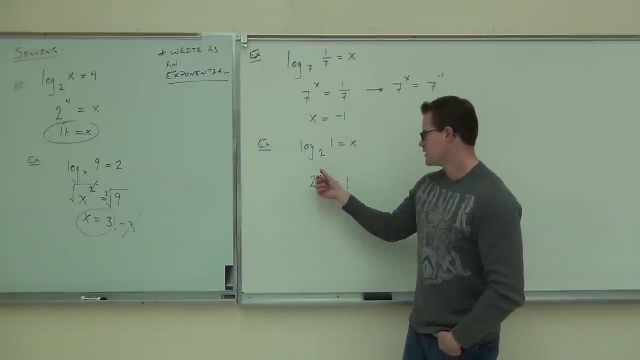 2. To the x Equals 1.. Okay, Now you tell me what's the only way in the world I can get from 2 to the x and make it equal to 1? What does the x have to absolutely be? 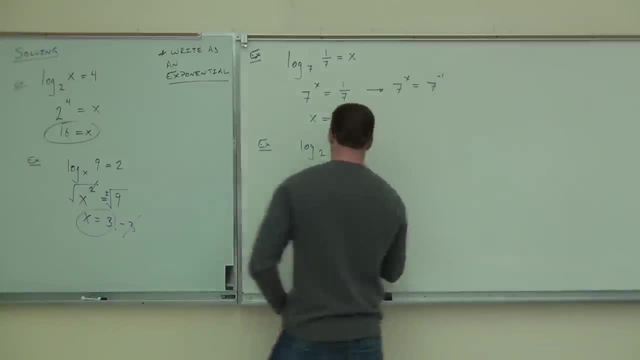 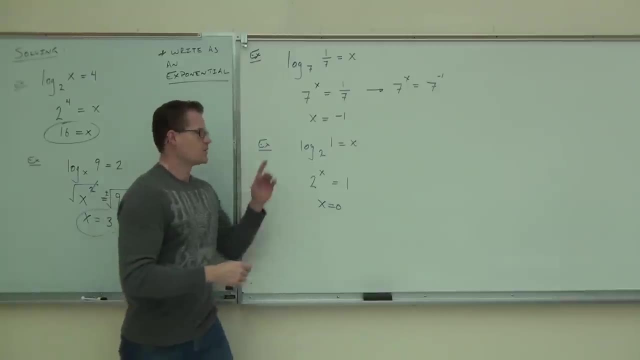 0.. 0. Absolutely, it has to be 0.. Now here's the question for you: Do you understand why it's got to be 0?? Yeah, The question is, if I change this base to anything, is this answer going to change? 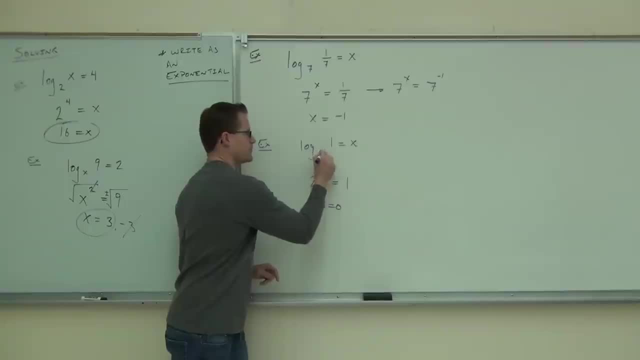 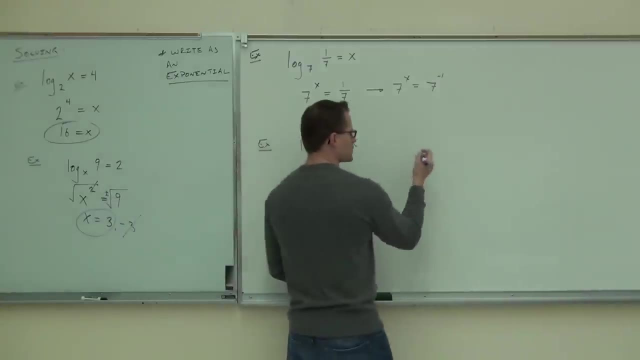 No. So if I say: oh, now the base is 5,, so that would be 5.. Is x still equal to 0?? Yes, Here's what this says. Just a little property Log base: anything of 1.. 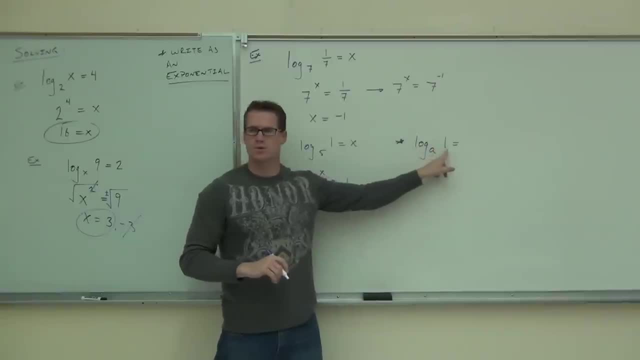 Log base. anything of 1 gives you what. That's a property right there. If you have a logarithm of 1, no matter what the base is, it's going to equal 0. So on your paper, every time you see log, if that's a 1,, whatever your base is, it doesn't. 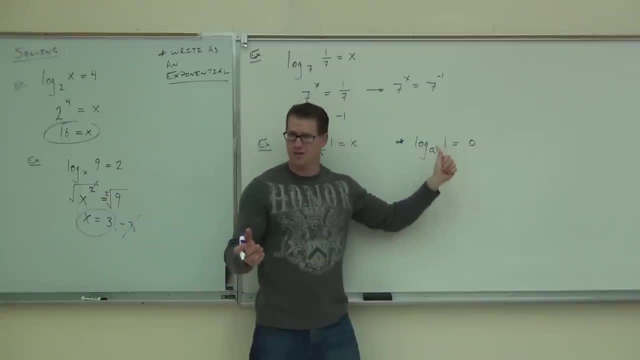 even matter Log base whatever of 1 is going to be 0. Do you see why? Because it says: no matter what you have, you have to raise it to the 0 power in order to get 1.. That's how exponentials work. 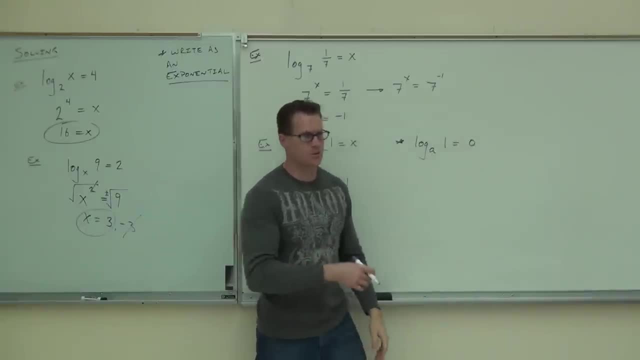 That's how this works. That's just a little property that we have up here. So what's the answer? 1. 1. 1. 1.. All right, so it's just an integer, An important one. 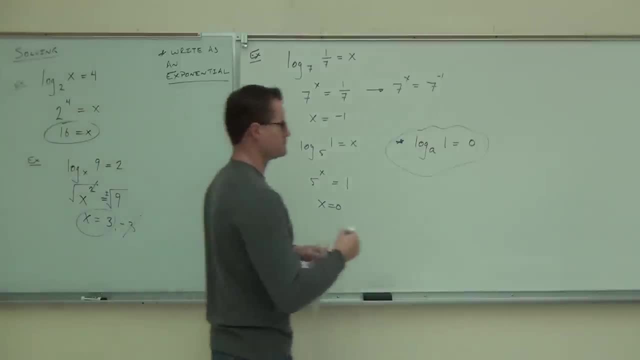 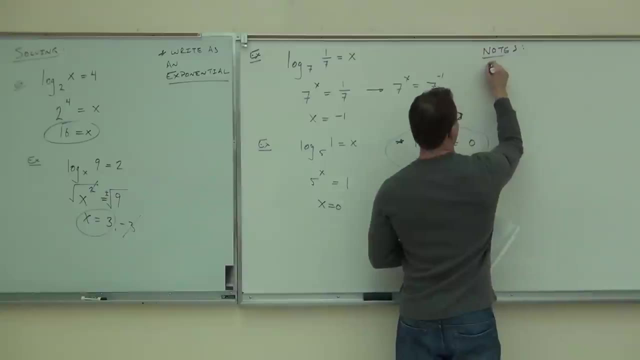 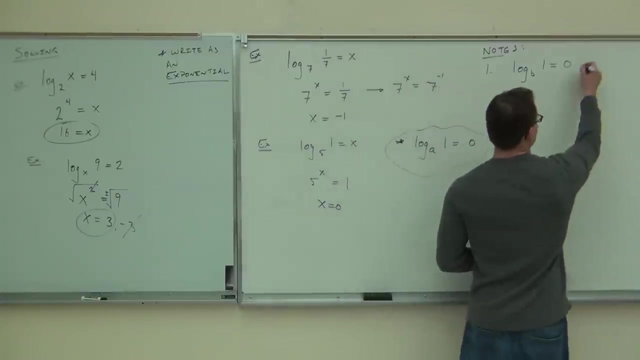 Let me show you a couple other properties that we've got. We'll call these things some notes. The first one. I'll organize it for you. The first one is this one: Log base B of 1 equals 0. I don't give you the reason why, if the right. 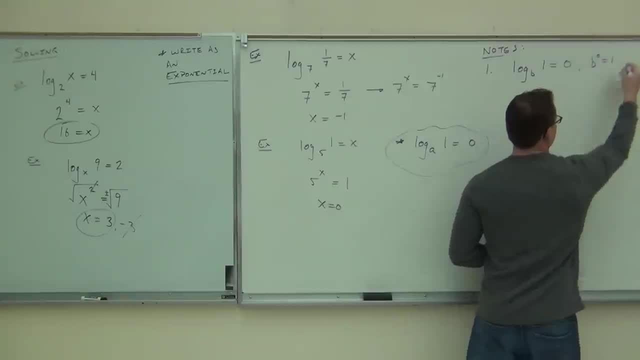 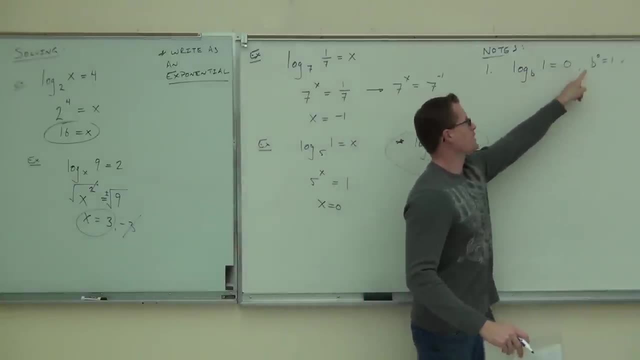 The right kind of thing, because b to the zero equals one Log base. b of one has to equal zero, because any base to the zero power gives you one. This is the property. this is the reason why I put a little check mark to make sure. 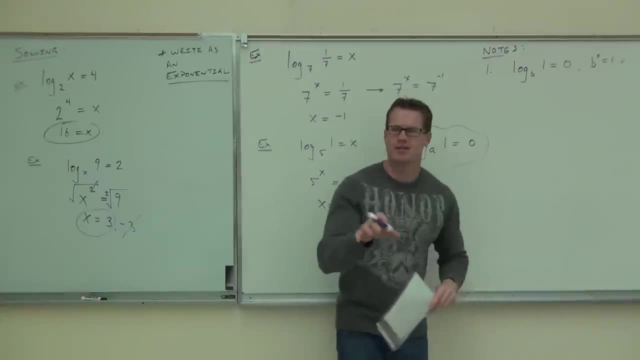 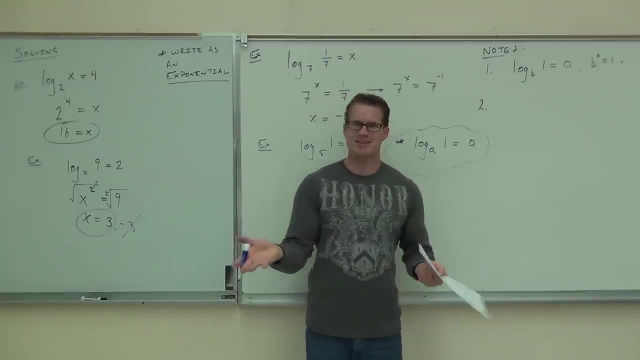 that you know it's true, true statement. Here's a couple other. these ones are really interesting. Well, they're interesting to me. I'm gonna make them interesting to you. See how that works? Okay, cool, All right, here we go. 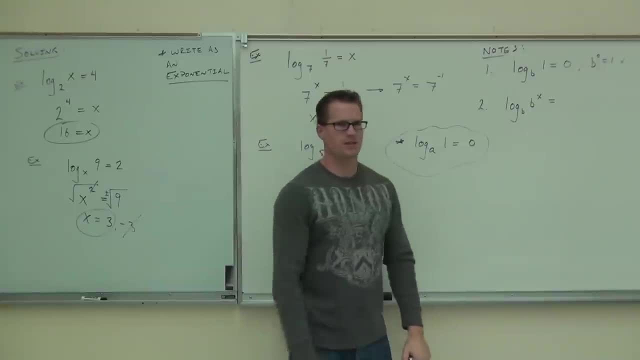 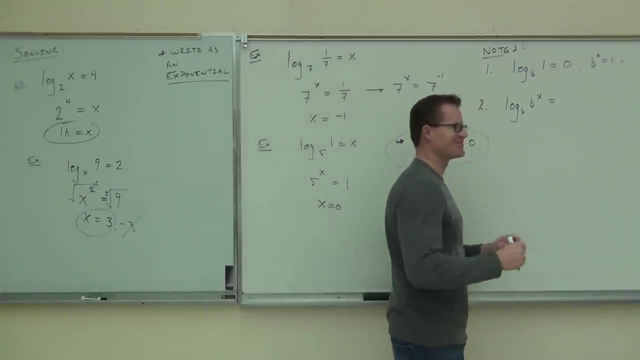 Log base b of b to the x equals what? Oh my gosh, that looks really confusing. x, x, x. Oh, you guys are good Y x. This is b raised to the x power. Check it out. 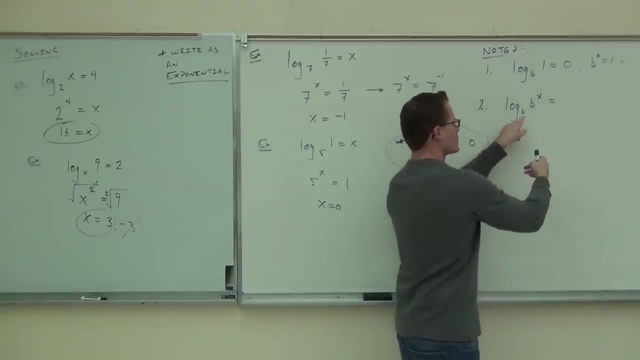 What is your base here? B, So this says watch. b to what, this is what right now. b to the what equals b to the x. If your bases are the same, what do you know about your exponents? They're the same. 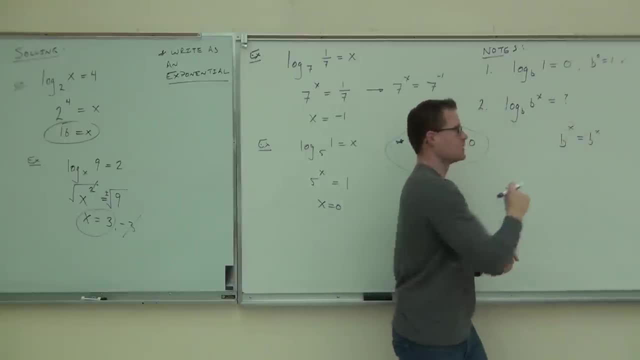 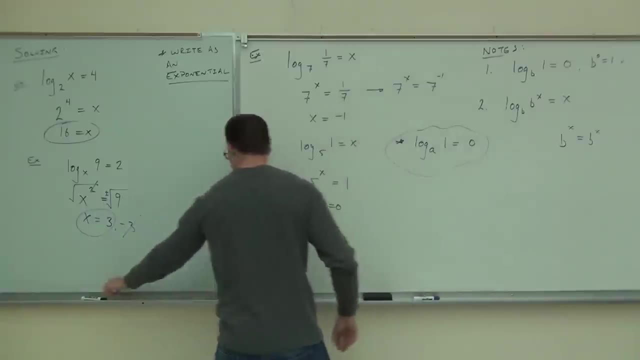 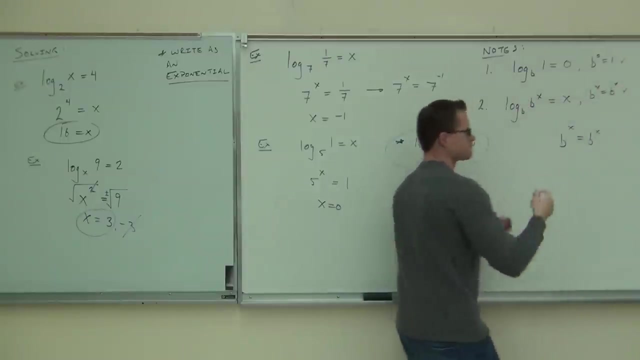 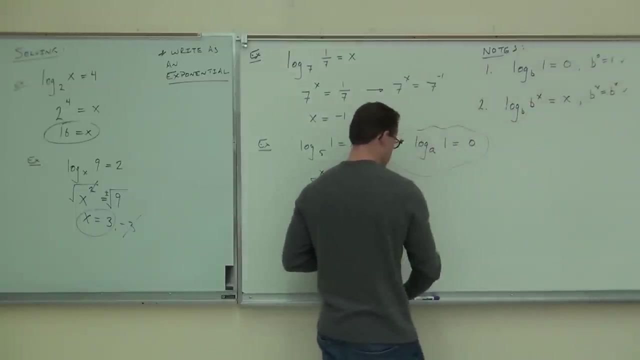 So then this would absolutely have to be an x. True, Then this is an x. You guys are right. very good, That's because b to the x equals b to the x. I have that right here, Okay, third one: 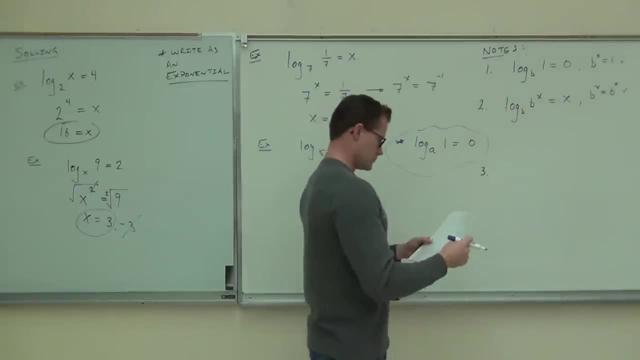 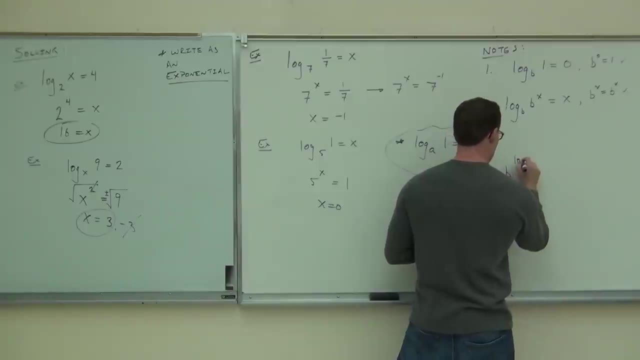 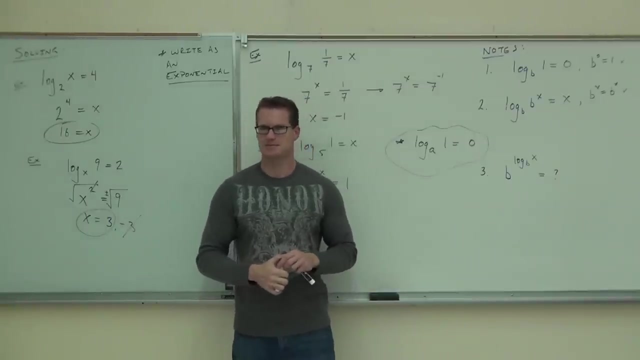 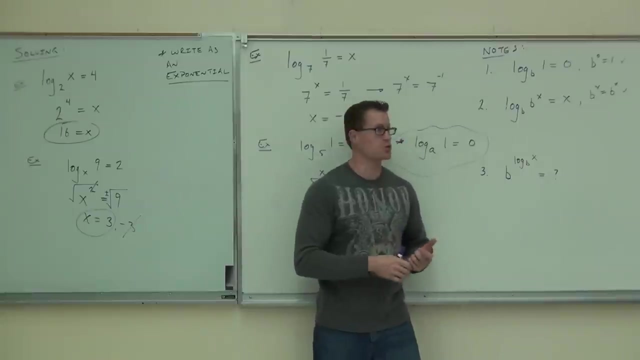 Thank you. How about that one? Hey, that looks even nastier. That's even worse. Well, this is actually an exponential, do you see it? It's a base raised to a power equal to something, Do you see it? 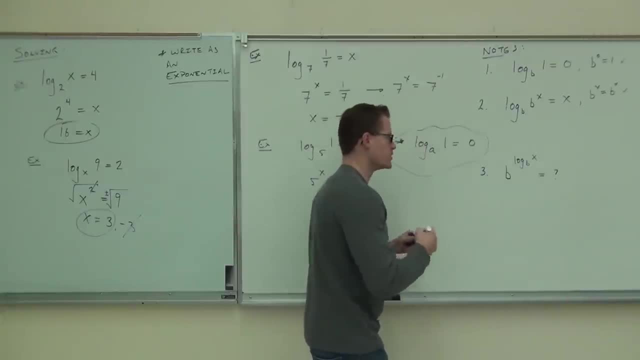 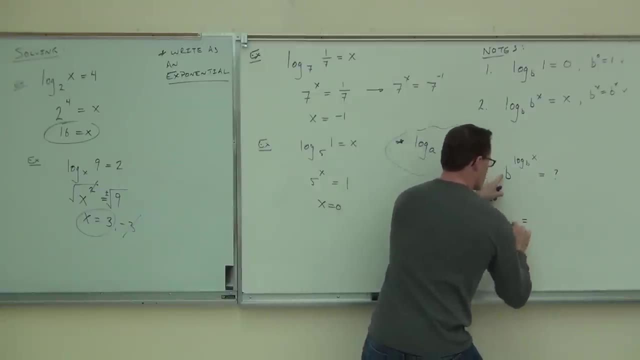 Let's write that as a logarithm. If I wrote this as a logarithm, here's what it would do. It would say: log of my base, of my base, would equal my power. Do you see how you can translate from here to a logarithm? 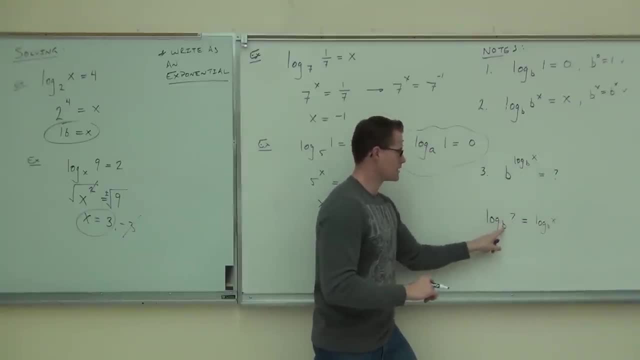 Are you guys okay with that? It says log base B. log base B of question mark- I don't know what that is- equals my power, because that's my exponent in this particular case. Hey, what does that have to be in order to make these things exactly the same? 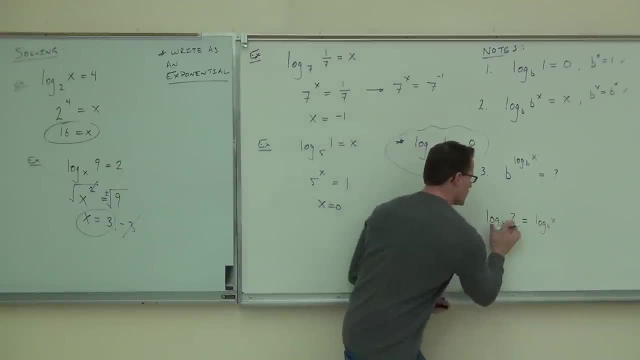 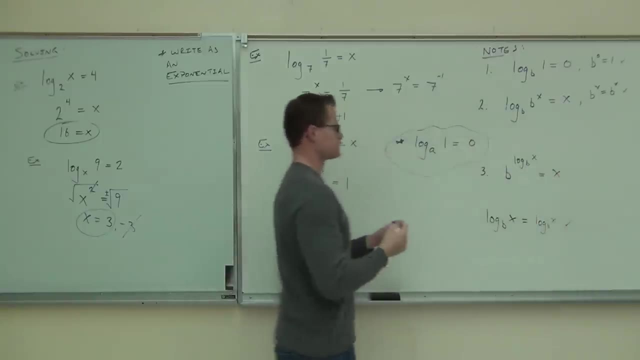 That's got to be an X. Do you see that that has to be an X? So this, if that has to be an X, means this has to be an X. Why? Well, because of this thing right there. Now, why don't you just learn those cool properties? 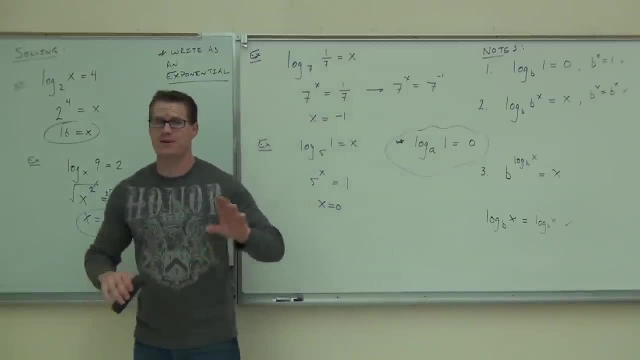 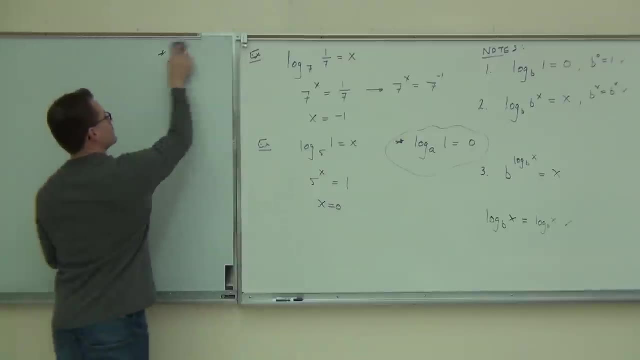 Well, check it out. Sometimes that makes your logarithms very, very, very easy to do, For instance, if you see some of these problems on your paper. we're going to use these properties later to solve some exponentials, But I'm going to show you how to solve them. 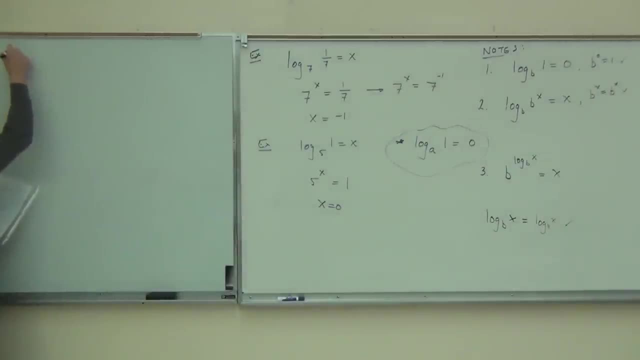 And to solve some logarithms. If you see this on your paper and you go: oh, what's log? base 6 of 6 to the 3rd. Well, what's that look like? Property 1,, property 2, or property 3?? 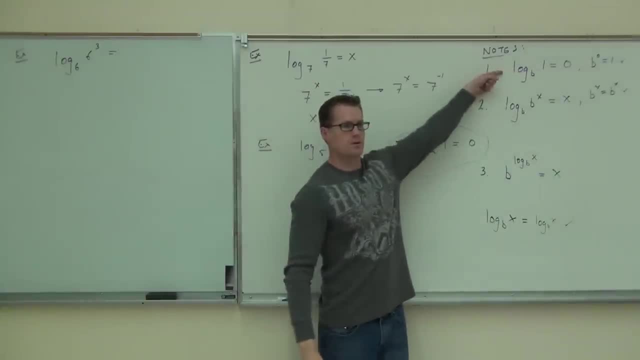 What do you think? Does it look like this one? Three, Two, This one Doesn't look like that one, because there's no base to a power, but it sure does look like that one, doesn't it? How much does that give you? 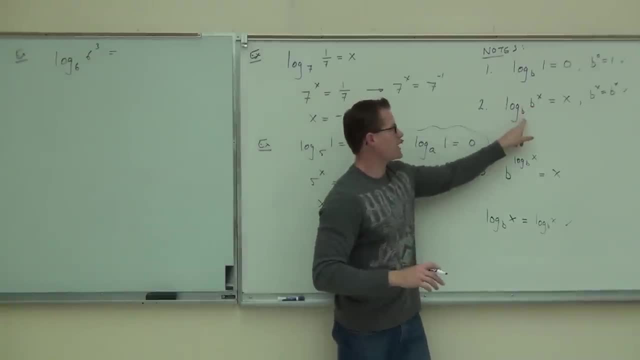 Here's what this basically says. here It says: if you have a power, you're going to have a power. If your bases are the same, if they simplify out of your, if you want to say cancel out, they cancel out. 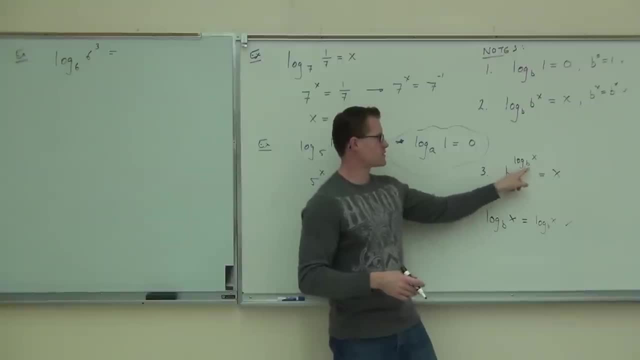 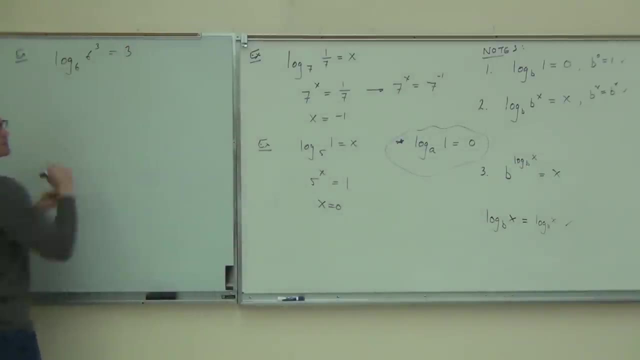 You're going to get the exponent If your bases are the same. look at that, bases are the same. you're going to get that x right there. So in our case, up here we go: oh yeah, those bases are identical. you're going to get 3.. 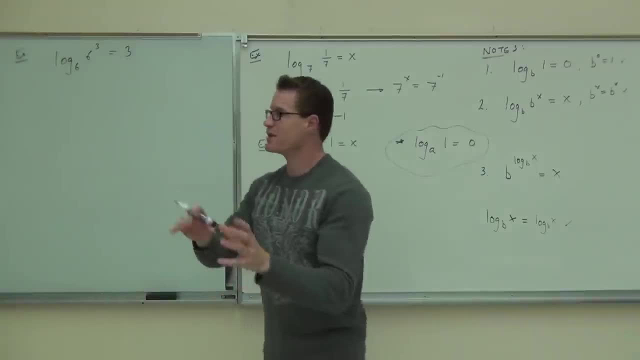 Do you have to show any work? No, it's a property. If your bases are the same, you're going to get that exponent. And the reason why is because if you were to write that as an exponential, you'd have your common bases already. 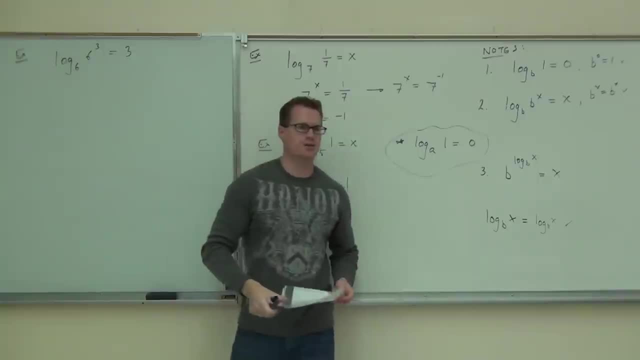 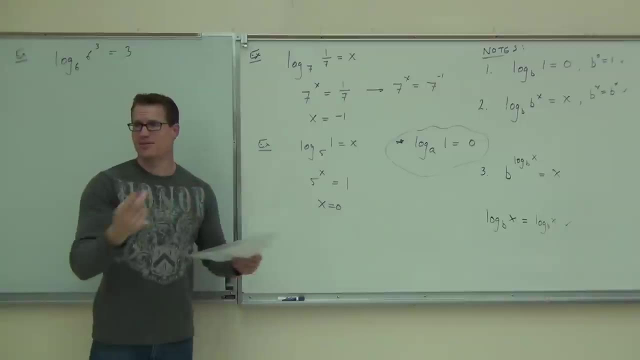 Your base would equal your base, You'd know your exponent. Your exponents had to be the same. That's the properties of exponents we've already covered. Isn't that kind of nice? Isn't that nice, Geez? I think that's beautiful. 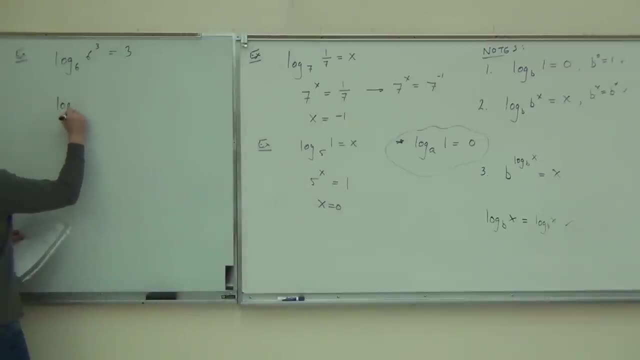 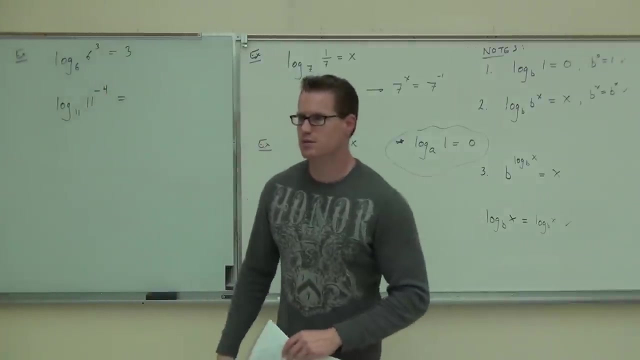 I mean that's fantastic. It lets you do a lot of work for free, For instance. if you look at that, you should be able to tell me immediately what that answer is. what is that answer? Yeah, where are you getting the negative 4 from? 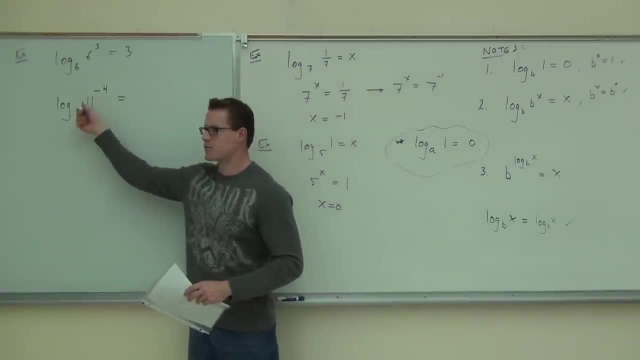 How do you know for a fact it's going to be negative 4?? Well look, your bases are the same, right? That means, if you set that up as an exponential, your bases would be the same, and this and this stand. 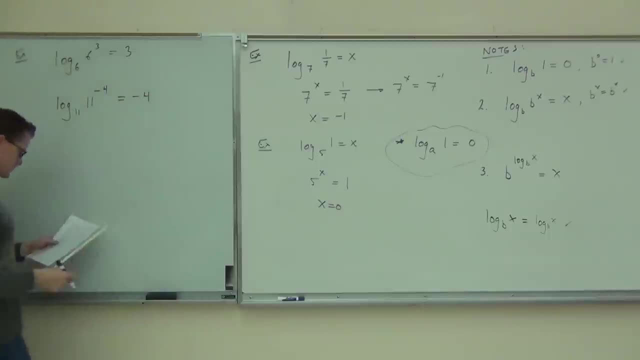 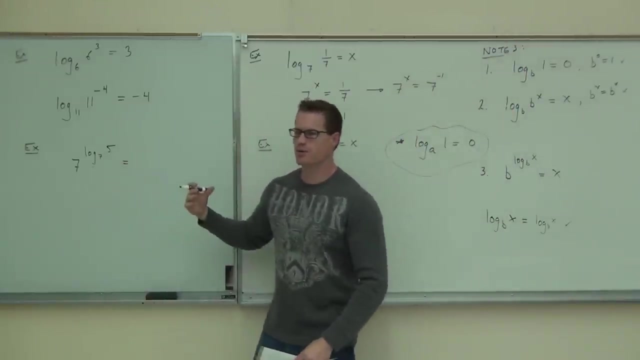 for an exponent that has to be negative 4.. Now that one looks a little bit different, but the same principle applies. We have an exponential now, but if we were to write this as a logarithm, This would be the inside part, and this stands: 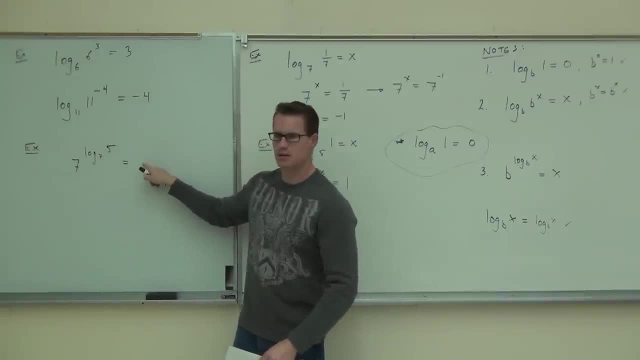 for the inside part of some sort of logarithm. So what does this have to be? 5. That would have to be 5.. If your bases are the same, it means your logarithms are going to have to be identical along with the inside part. 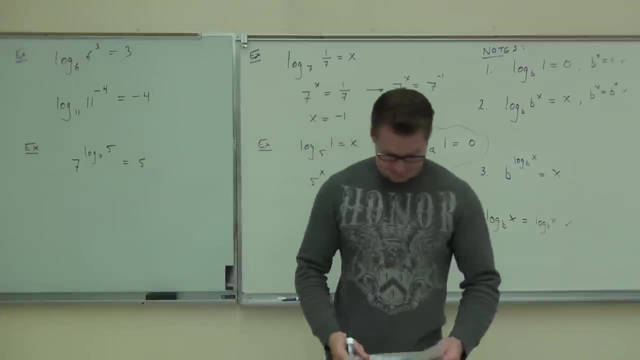 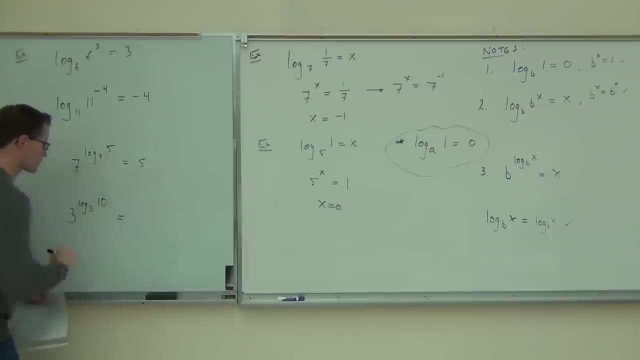 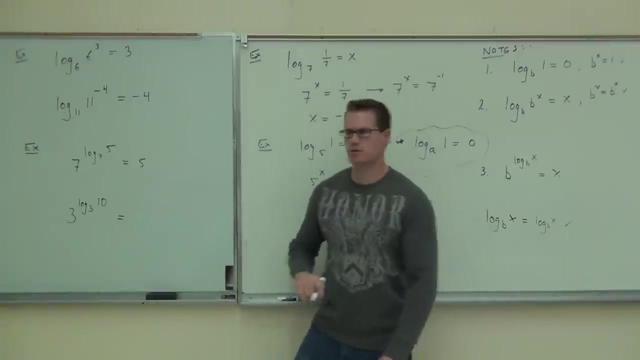 of those, we would have the 5.. How about 3 to the log base 3 of 10?? Everybody, how much is 3 to the log base 3 of 10? 10. 10. 10, sure. 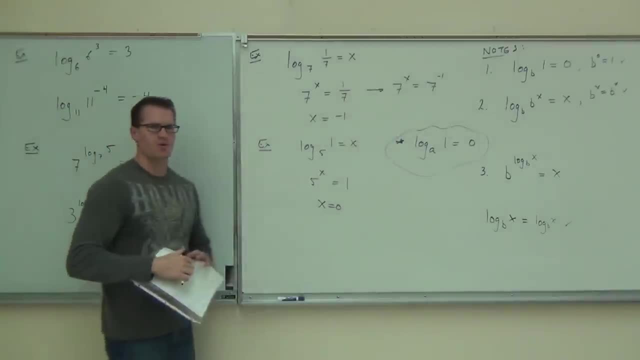 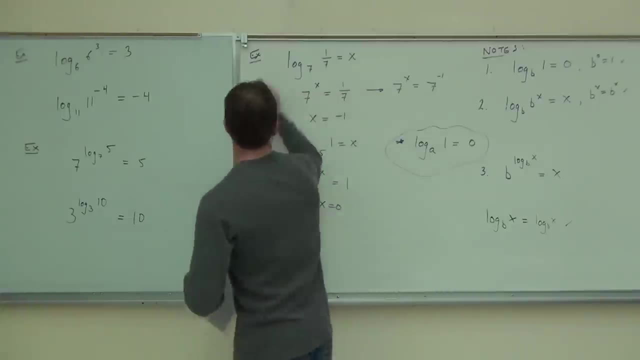 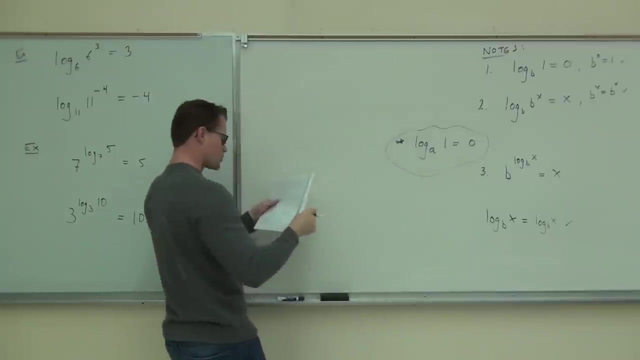 Absolutely, And your test? aren't you going to want about 30 of those? Just call it a day. No, No, right, Too bad. Yeah, it's not that easy. That would be nice, though. Try a couple of these on your own, and then we'll continue. 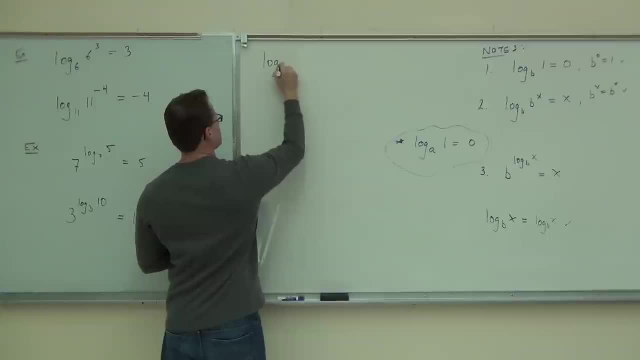 Let's do log base 5, 5 to the negative 2.. And we're doing log base 5.. And this is a fun final piece. this is a very exciting one. Come and find out what I'll do with all these� 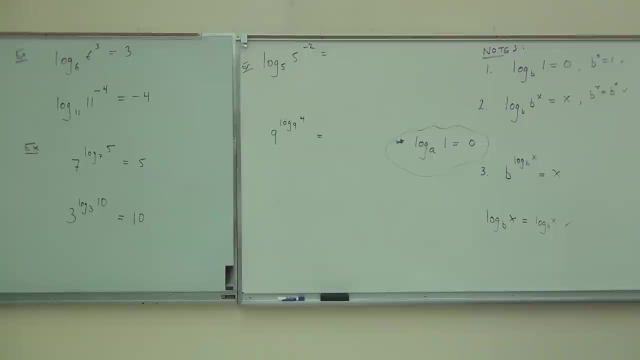 Log the logarithm of the pair. Sorry about that. Love to hear you talk. Yes, Yes, Yes, Yes, Yes, Very nice. Thank you y'all Doing a good job by explaining those repetitive pensari, But thoseradas. 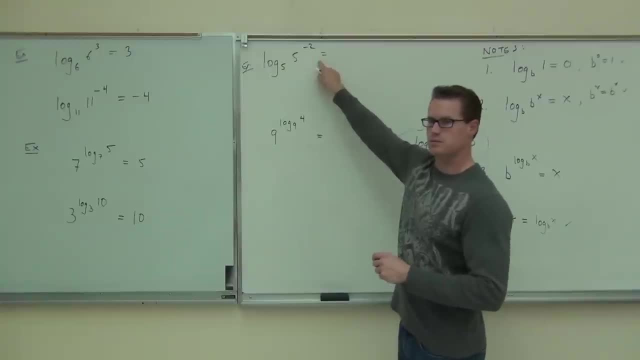 Thank you, Thank you, Thank you. How much is this one? Why, Because of that one, We know that those exponents would have to be the same. How about this one Four? Would you raise your hand if you feel okay? 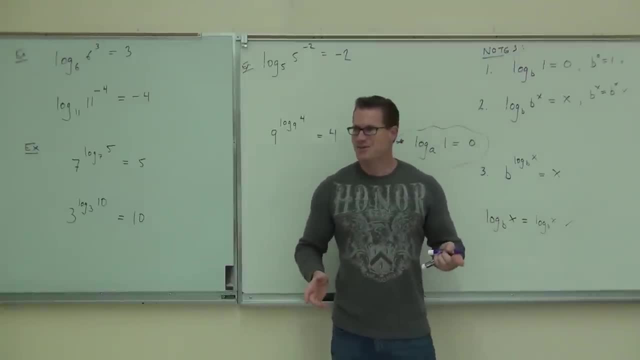 on these three things. Don't raise your hand yet. You don't know what I'm going to ask. Translating from exponentials to logarithms, Logarithms to exponentials, still And now solving these things as well, Okay, Last thing we've got to talk about. 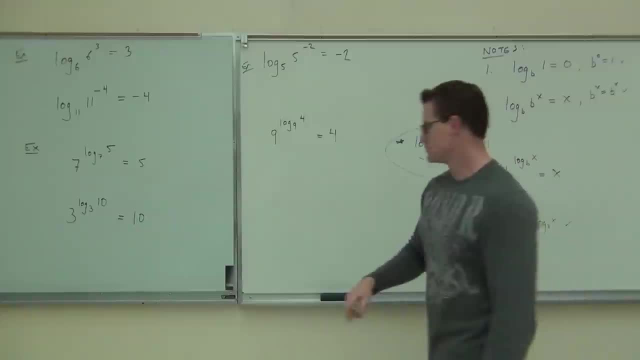 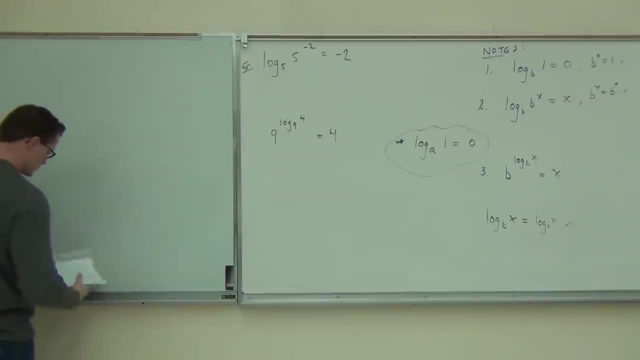 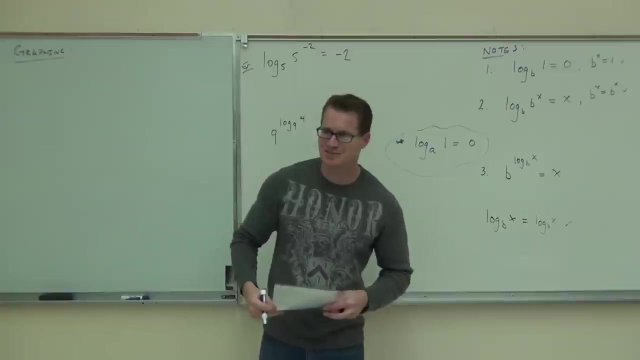 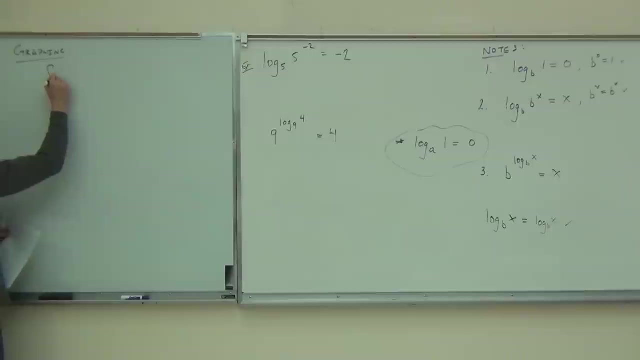 what do the graphs of logarithms do? Let's talk about graph. Energy level just went down. It's not that bad. It's not that bad. Well, here's the deal. all right, If we are trying to find the inverse of this. 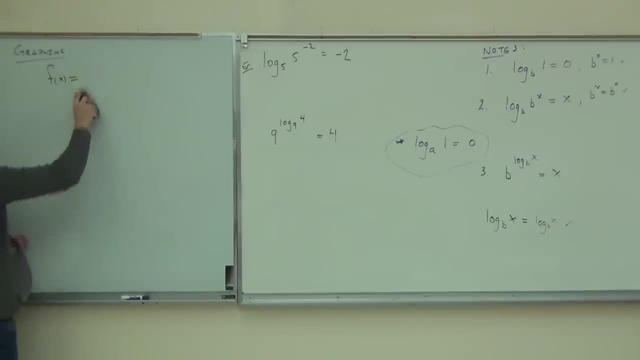 which is an exponential. oops, no, it's not. This is Like that, And we try to find the inverse. So this is back to our original problem. We of course have y equals 2 to x. You'd tell me x equals 2 to the y. 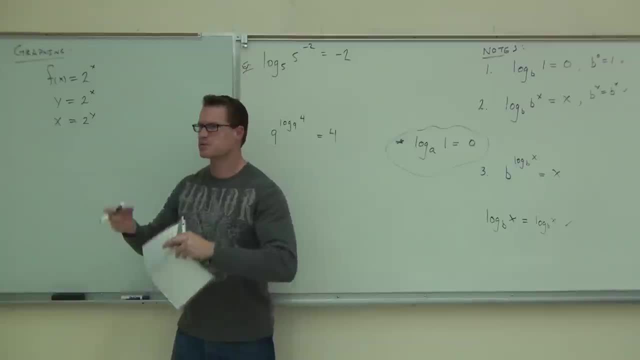 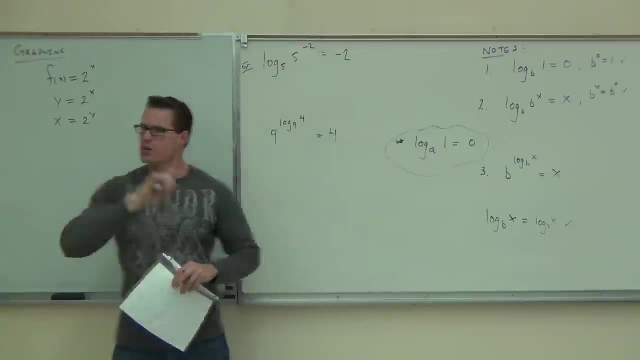 That's how inverses are found- is by writing the y equals and switching those variables, y with x. And then you'd say: oh well, wait a second, There's no way that I can solve this. I can't solve this for y unless I use a logarithm. 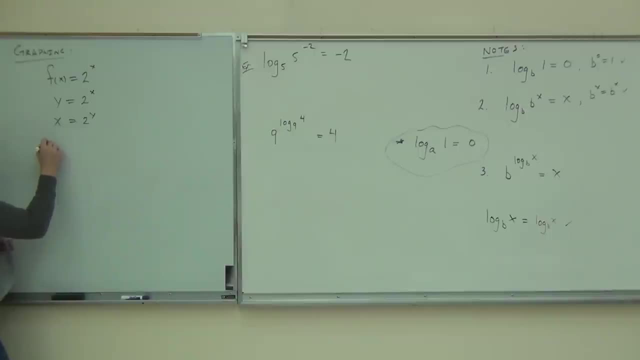 So I would say: okay, well then log base 2 of x would equal y. Are you okay on that so far? I hope so, because you just raised your hand. if you were okay on translating these to logarithms, That's translating to logarithms, right. 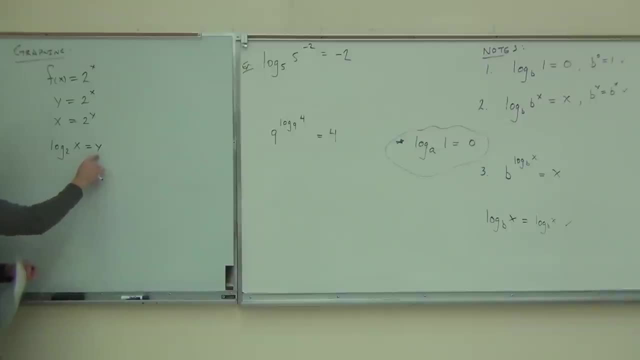 And we knew from before that this y would be written as f inverse. You follow me on that one. So you'd have f inverse of x would equal log base. 2 of x equals y. She's right. two of x. Hey, that's a function in terms of x. That's something I should be able to. 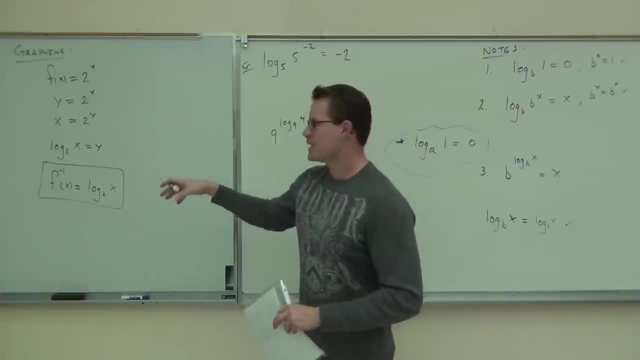 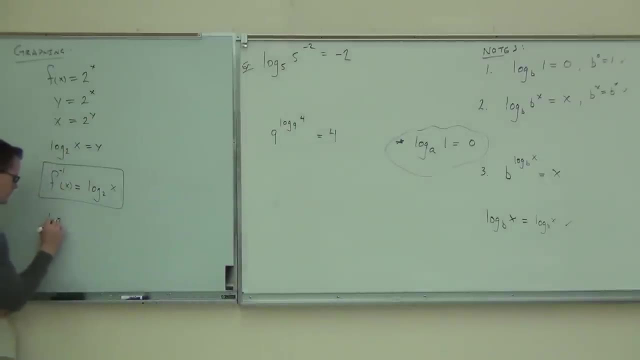 graph. That right, there is one example of a logarithmic function. In general, logarithmic functions look like this: Of course, they have a name of a function. They're going to have a logarithm in there, They'll have some sort of base and then they'll have some function. 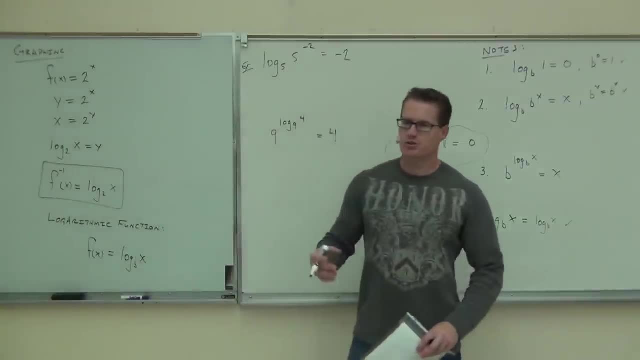 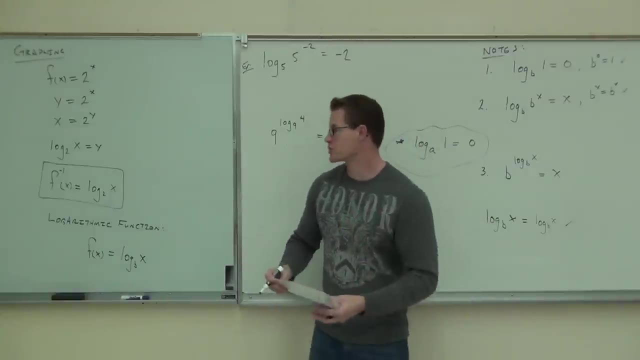 in terms of x Log base v of x. Now, what's very interesting is that every logarithmic function comes from an exponential. It's an inverse of some exponential, Just like this logarithmic function. look at that. That's an inverse, right? It's an inverse of 2 to 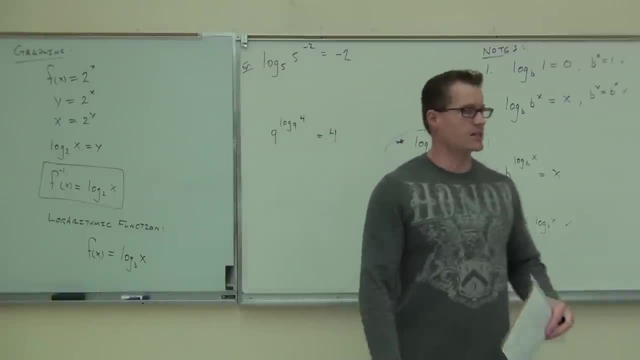 x. It's the inverse of that thing. That's how you get it is. it's an inverse. So in every case, a logarithmic function will have a logarithm, will have some sort of base, but this is always an x. 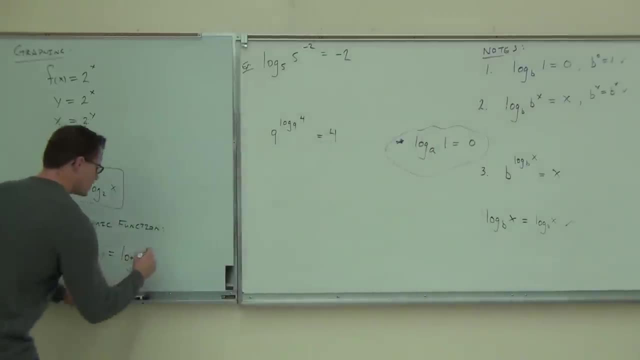 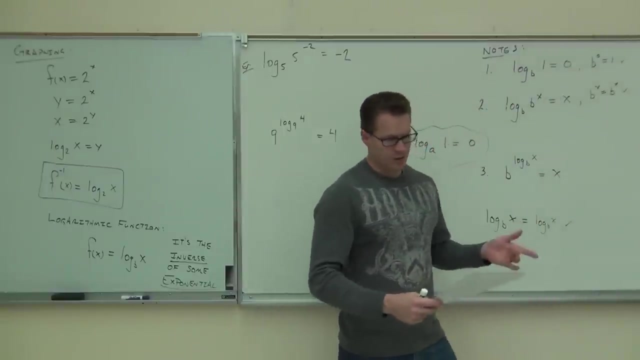 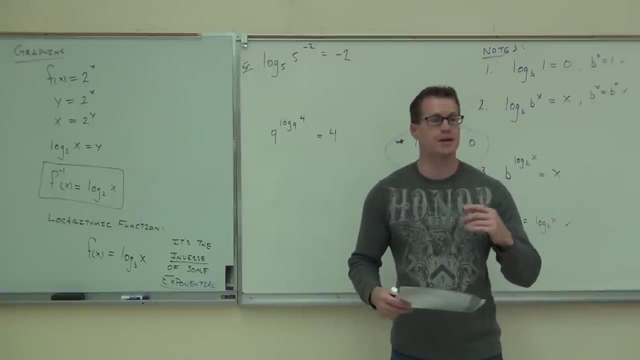 It's the inverse of some exponential. It's the inverse of some exponential function. Now, let's go ahead. We'll graph one of these things. I want you to get the idea about how this looks. I'll refresh your memory on what exponentials look like and we'll see. 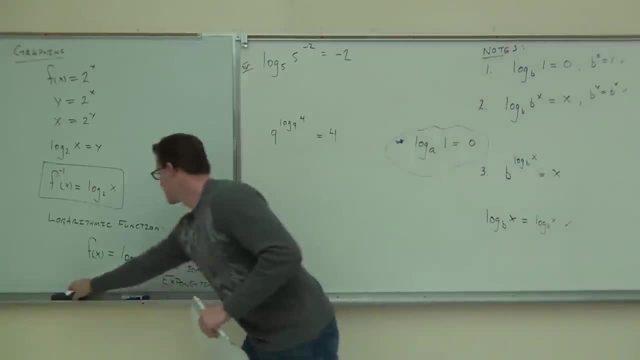 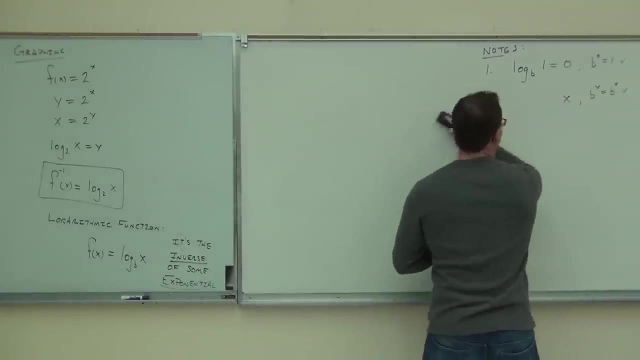 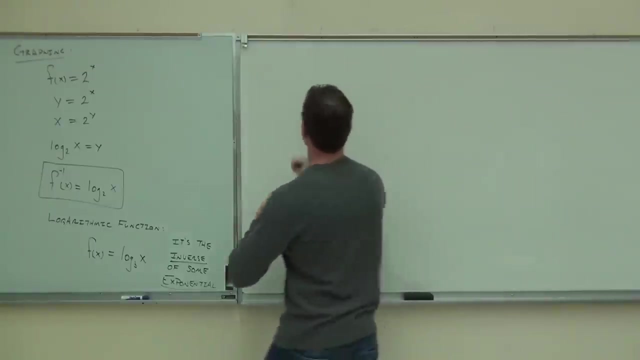 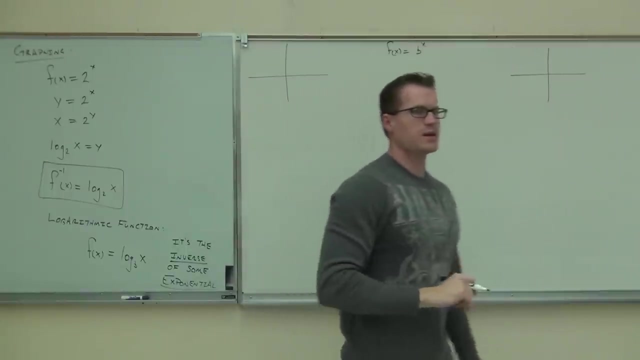 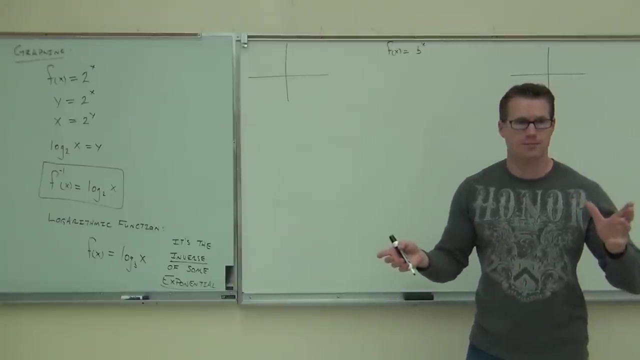 a very distinct relationship between them. f of x equals v to the x. Is that a logarithmic or an exponential? Exponential? That's definitely an exponential. It has no logarithm anywhere in there. right Now, these graphs have two shapes. Do you remember the different shapes? 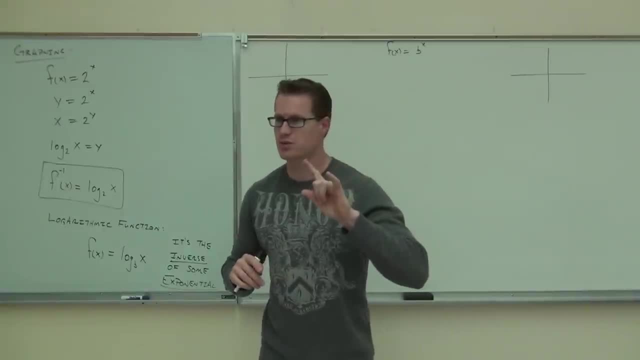 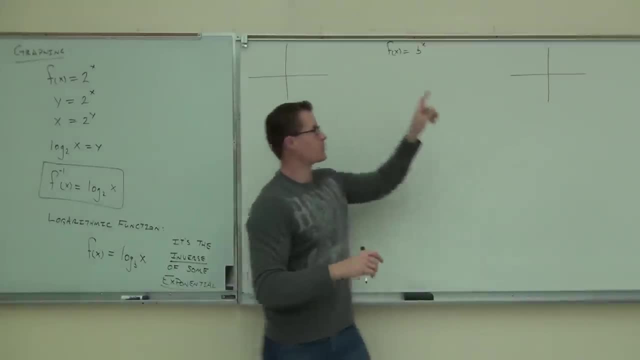 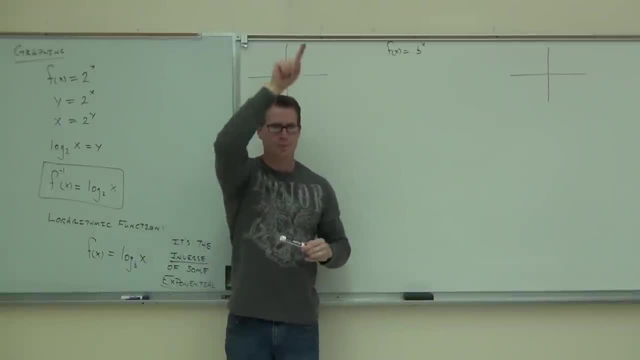 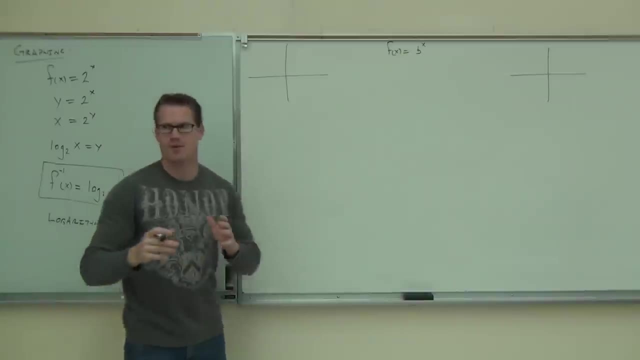 Were they down here? No, No, No, They were definitely above all of x-axis, right? Yes, One of them went. Yeah, Remember that, Mm-hm. Yeah, You know this sound effect, don't you? 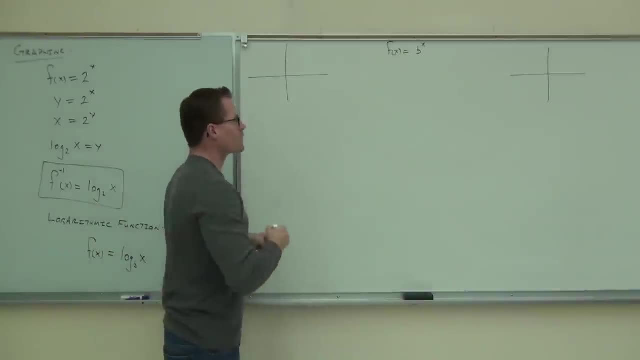 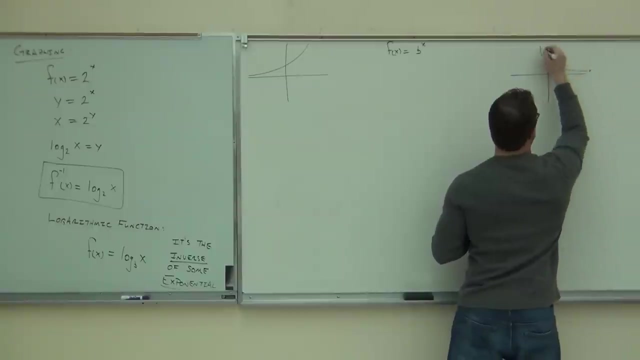 And that that's a real good way to well. it's the way I memorize this all the way through on math classes. One of them looked like this: Roughly. One of them looked like this: Am I correct? How does one look like this roughly? 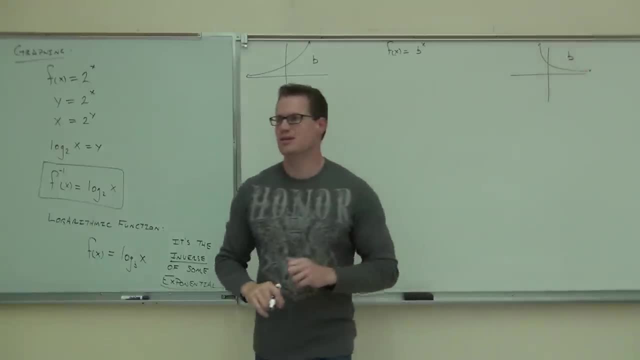 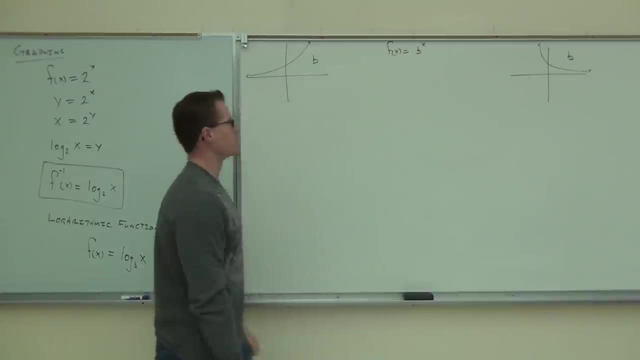 One of them, the base was greater than one. one of them, the base was less than one, but the base was always greater than zero. it was never negative. If it was negative, it'd be below the x-axis. you'd have a negative in front of it. 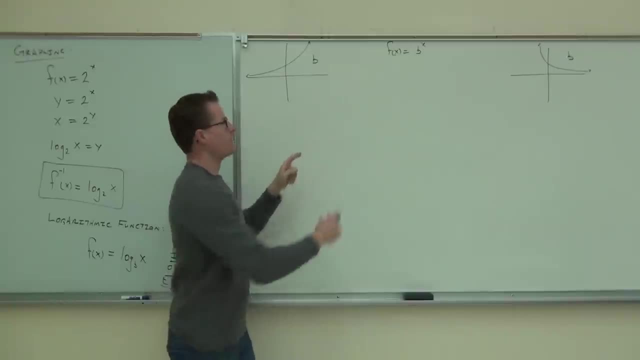 What's this one B greater than one or less than one Greater than one? This one less than one, But in each case they cross at the same point, unless you shifted them around. Do you remember talking about those shifts? 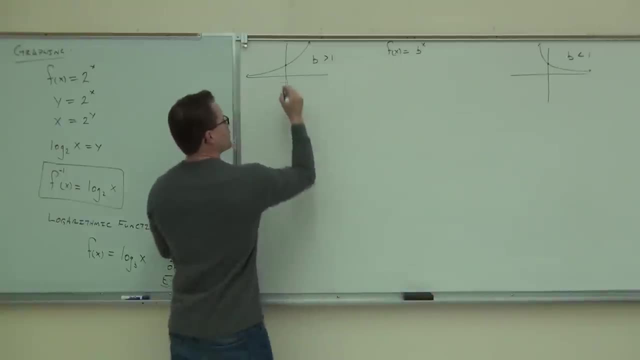 You saw the up down left right shift. I told you that last bit of class, last time They all crossed at what was this point? again, Zero and one. Zero and one. that's right, because when you raise anything to the zero power. 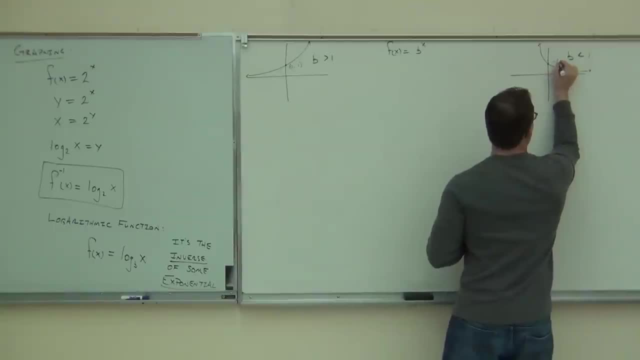 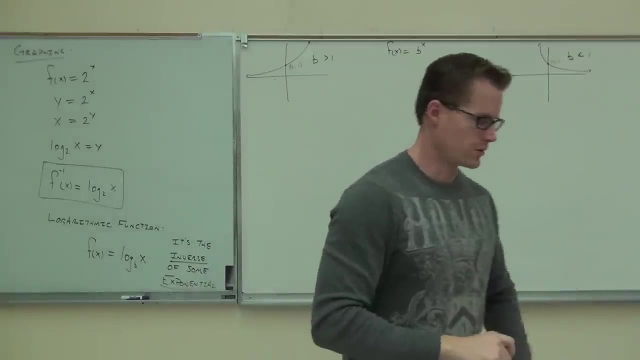 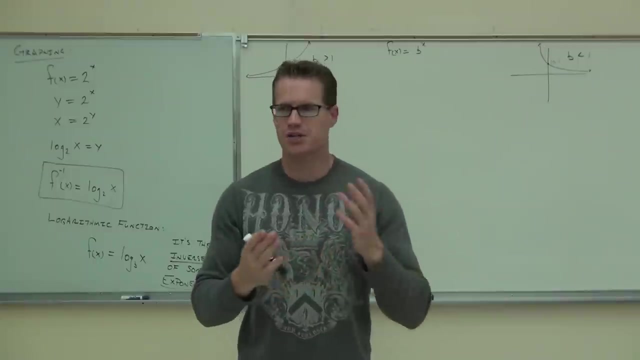 you get one out of it. Now, what we're gonna talk about are logarithms. What are the inverses to these things? Now, this would be so cool. I'm gonna tell you about inverses. Do you remember? inverses are simply a reflection across a diagonal line. 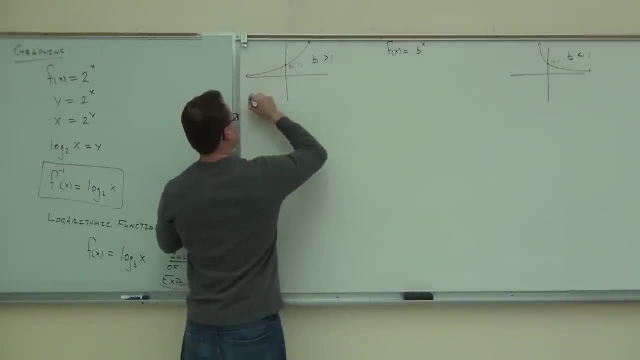 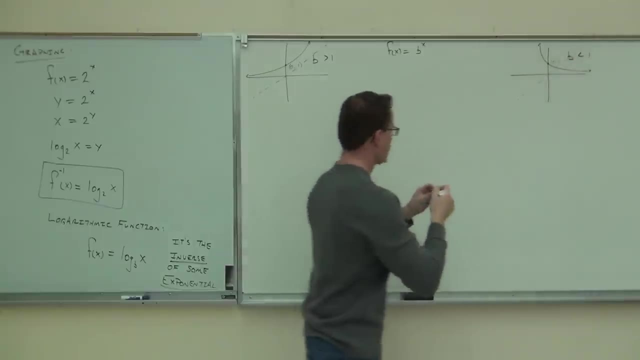 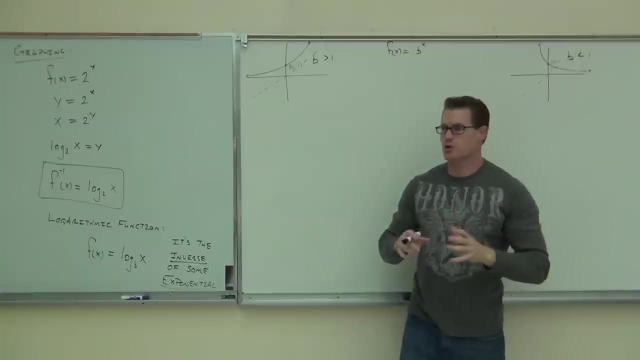 So basically, if I draw a diagonal line right here and right here y equals x and I flip this, that should be a logarithm And I flip this. that should also be a picture of a logarithm. You ready for it? 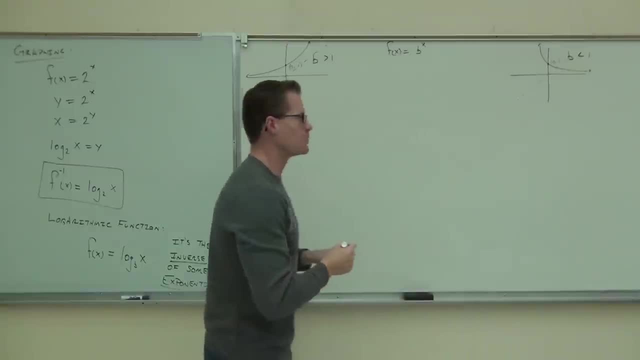 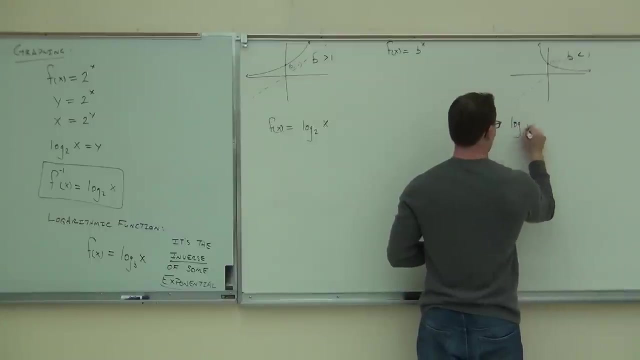 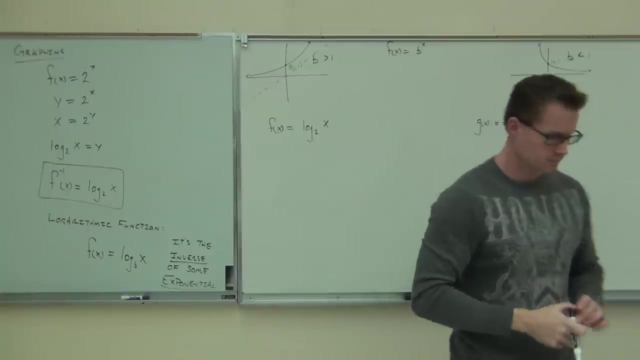 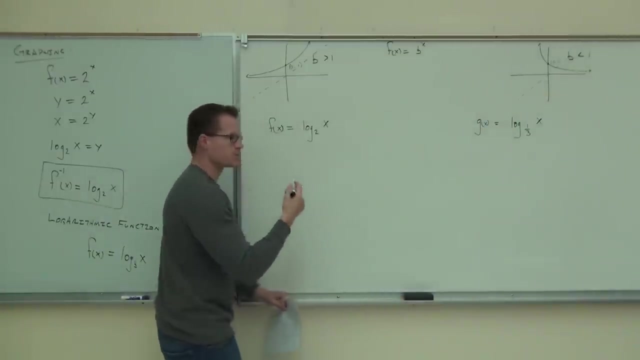 Ready to see it. We're gonna do this pretty quickly. We're gonna make a table of this thing. I'm gonna talk about f of x equals log base two to the x to keep it easy, and one third base x To make it a little bit easier for us to get. 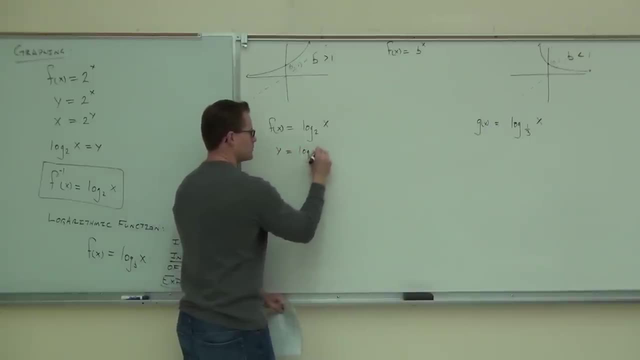 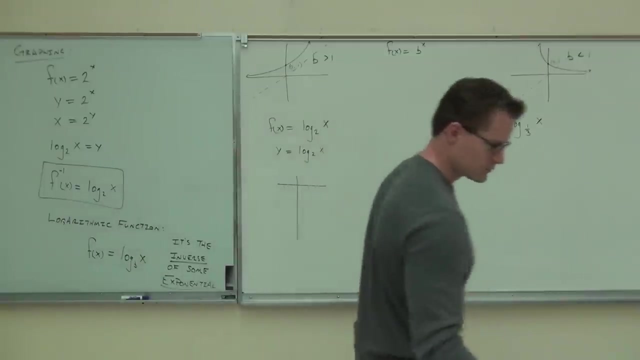 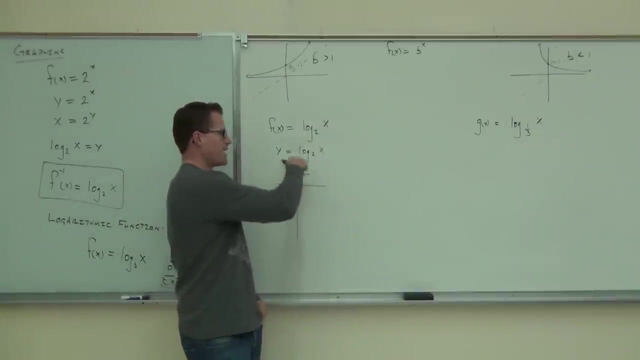 instead of f of x, I'm gonna talk about y. Hey, by the way, could you write that as an exponential? This right here would say two to the y would give you x right. So over here I typically have y's. 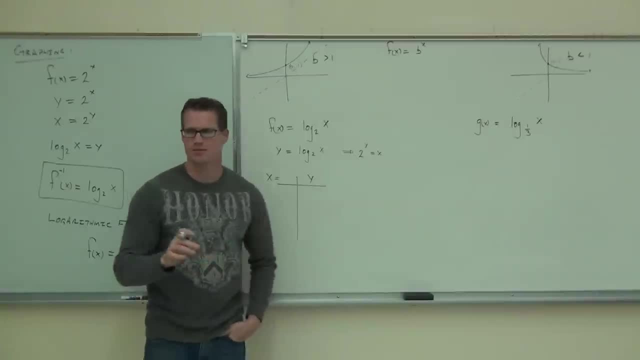 and I typically have x's. But here's the deal: to make these tables, you have to do them backwards because they're inverses. We're gonna have y's over here. we're gonna have two to the y right here, Instead of plugging in x's and getting y's. 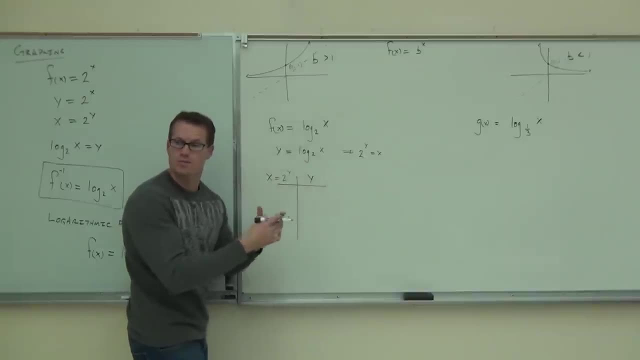 because that's hard to do. we're gonna plug in y's and we're gonna get x's. It's gonna be backwards, what we normally would do. So with my y's I wanna check for zero, one, two and negative one. 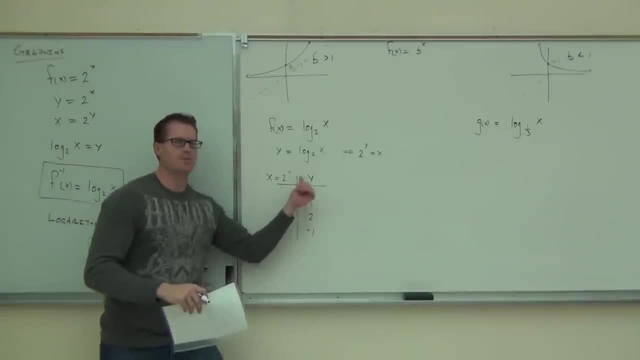 We'll see what happens there. So notice that instead of plugging in my x's, I am plugging in y's. first I wrote it as an exponential and I'm plugging in y's over here to get the picture of this graph. 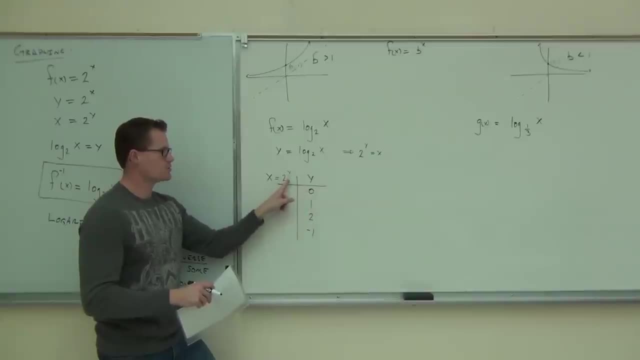 So if I plug in zero, everybody, what is two to the zero, please? It still gave me a point, didn't it? This x, that's y. I'm just finding x a little bit differently. Let's plug in one. 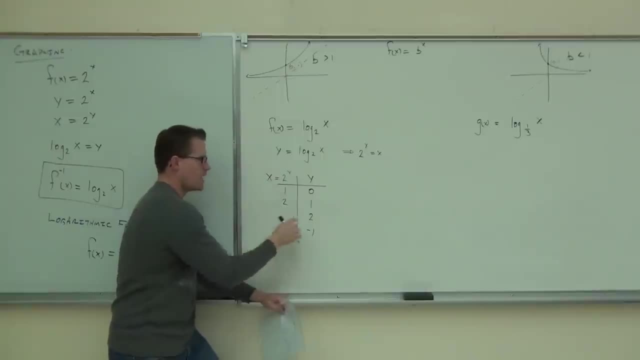 What's two to the first power? please Two, Okay, How about two? What's two to the second power? One, How about this? one? Oh, this is interesting. One half. What's negative one? Two to the negative one gives you what. 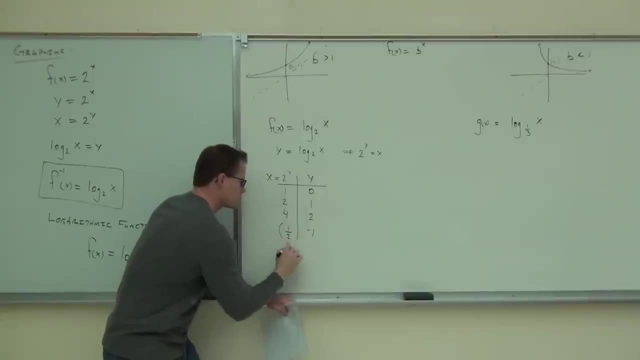 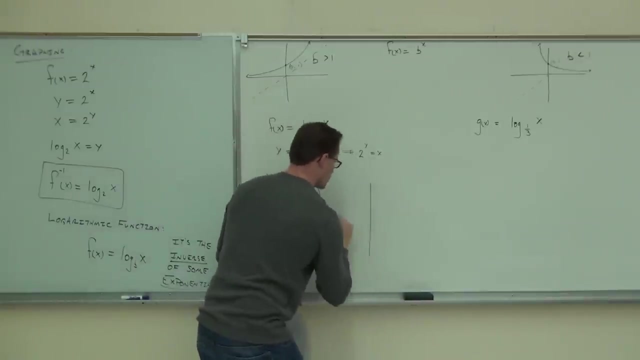 One half, One half. Do you still have points? Yeah, Don't lose track of your x's and y's. They're still in the correct order. If I plot these points, I get 1,0,. I get 2,1,. 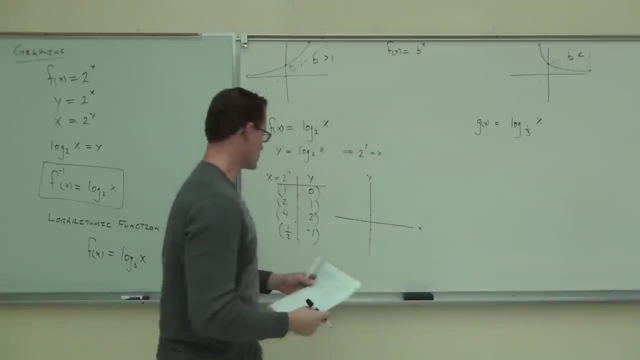 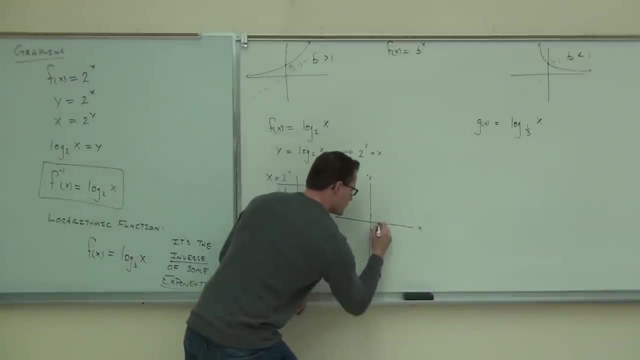 I get 4,2.. Do you see what that side of the graph looks like It's going to go? looks like that. So if I plot these points, I get 1,0,. I get 2,1,. 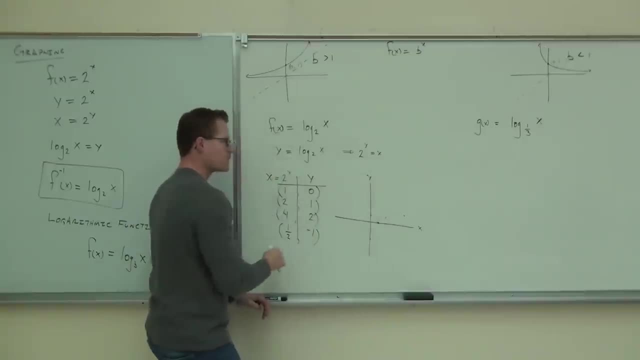 I get 4,2.. I get 4,3.. This side of the graph, if I plug in 1 half, if I plug in 1 half over here, try one more. 2 to the 1 half is a square root of 2.. 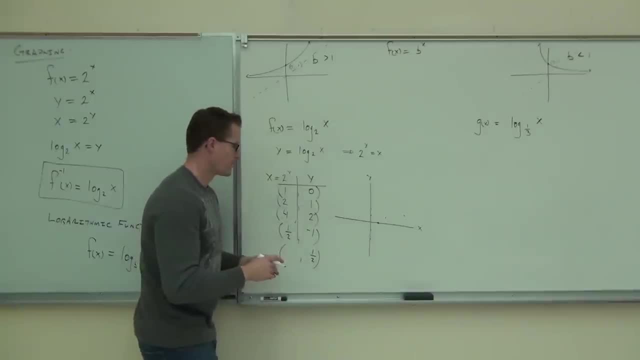 That's 1.41.. Oh sorry, let's see, I wanted no, I don't want 1 half, I want negative 1.. If I plug in negative 1, that means I'm going to get. oh, I already did that. 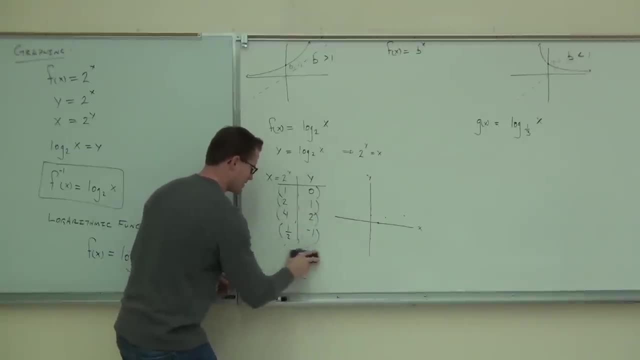 Oh, genius. Yeah, I already did it twice. I forgot I had that on the board. I was looking right at it. How funny is that? Okay, if I plug in 1 half, I get negative. Oh, that's what that does.